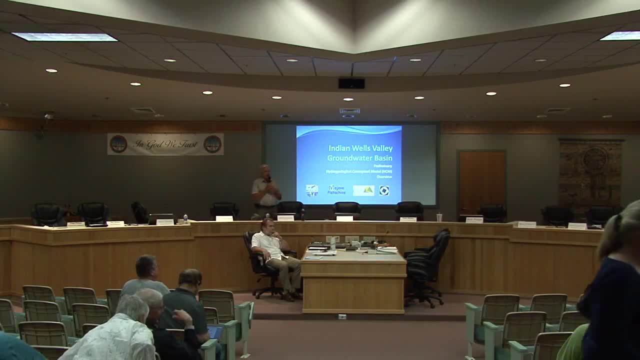 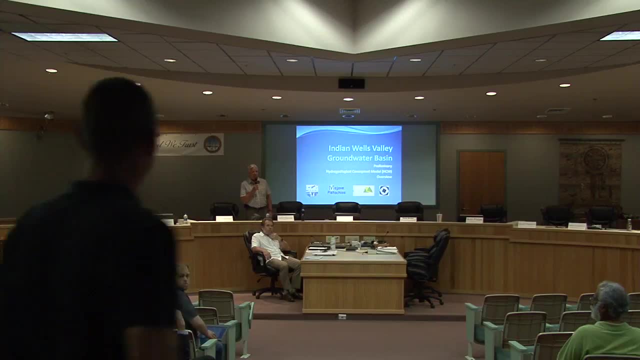 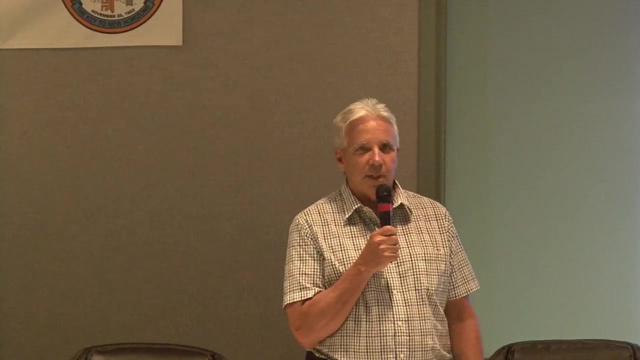 Okay, I'm Don Zadiv. I'm the general manager for Indian Wells Valley Water District and I want to thank those of you that are staying here to see this information. I'm sure there's a lot of glazed eyes out there. Our worst nightmare, if you will, came true. 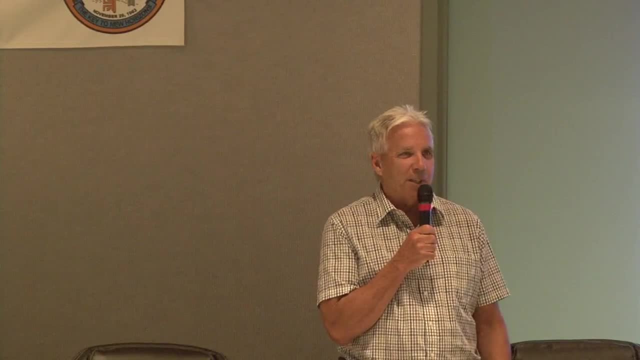 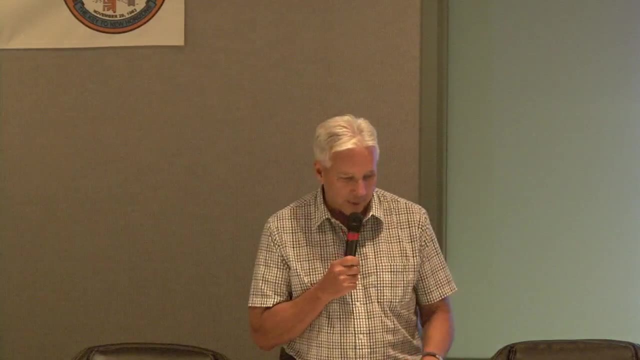 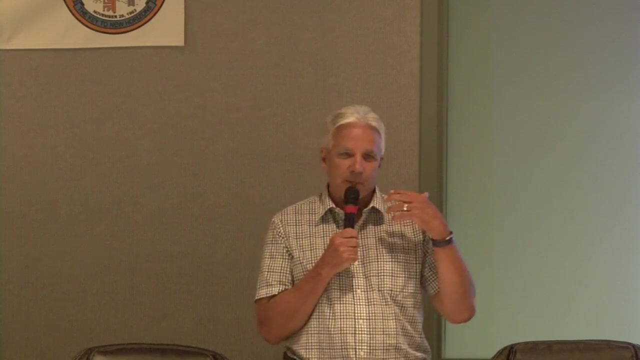 We were wondering how long this meeting was going to go, and it far exceeded our expectations, obviously. So we appreciate them going into closed session so we can do this and hold our 3 o'clock time. We planned this, I think we. I wasn't here for the dry run. I just got back from being out of town yesterday. 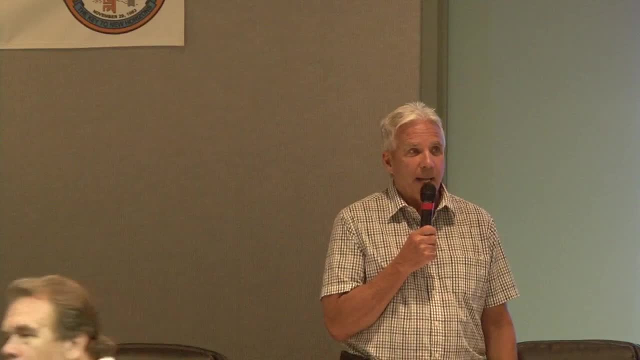 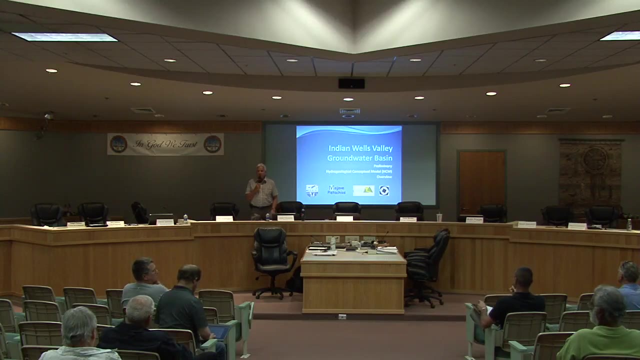 so I think we were planning on about an hour presentation and maybe a half hour for questions, so hopefully we can hold that schedule. I'd like to introduce the other members of the TAG team, if you will. that will be presenting. We have over here Tim Parker, who's 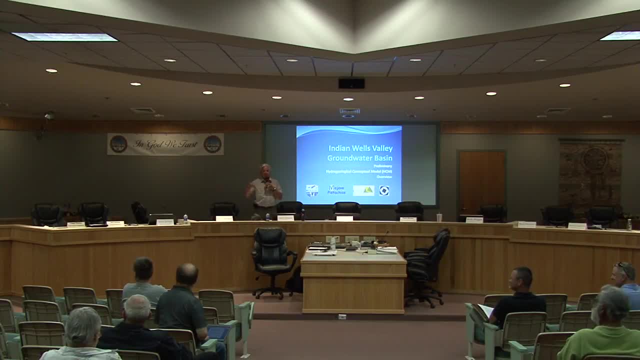 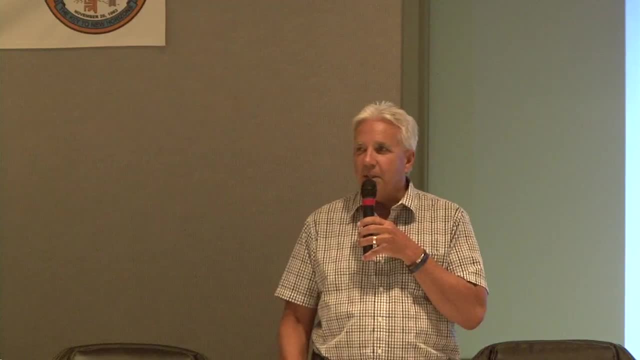 having a sidebar. Tim is with Parker Groundwater. He's the consulting hydrogeologist for the Water District and also our member on the Technical Advisory Committee. We also have Max Halkier. Max came all the way from Denmark to be here. He's with Rambo. 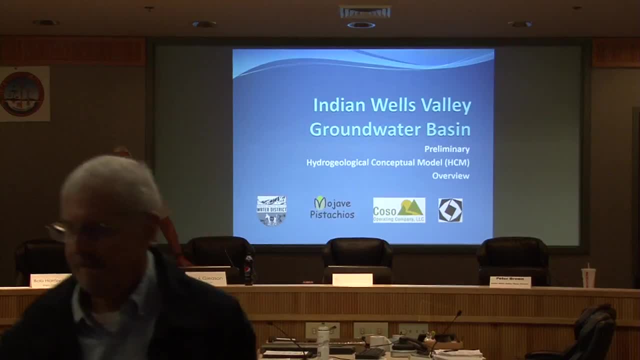 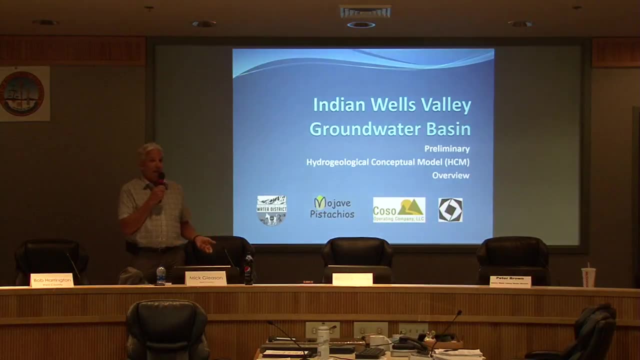 Rambo is the company that is doing the data management system and developing the hydrological conceptual model that is going to be based on the SkyTem data that was collected. We had hoped to present the model sooner, but it's not quite ready. So for those of you that are here, there will be a meeting plan for Friday, July 20th. 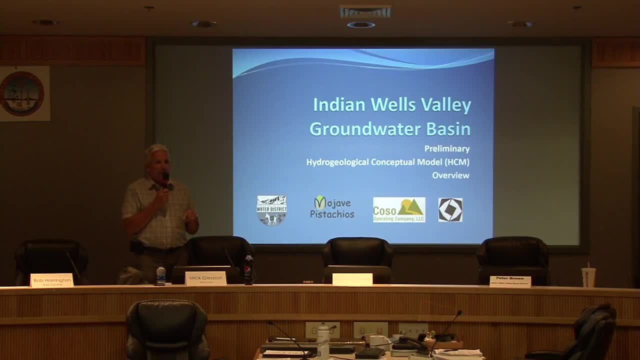 if you want to put that on your calendar here at 9 o'clock, And that meeting will be where the hydrological conceptual model is unveiled and thrown out for comment. So we'll get started. I guess I'm in control. I have a clicker here, so 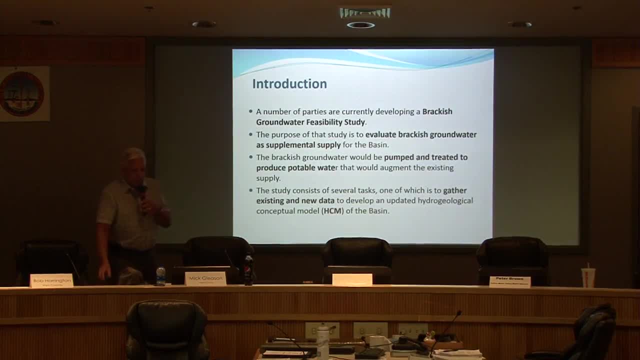 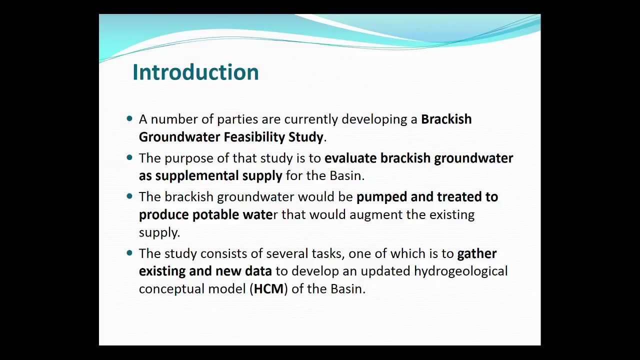 So, by way of introduction, the purpose of this – let me just stick to the script here. I'll do that. The brackish groundwater feasibility study includes a number of parties. 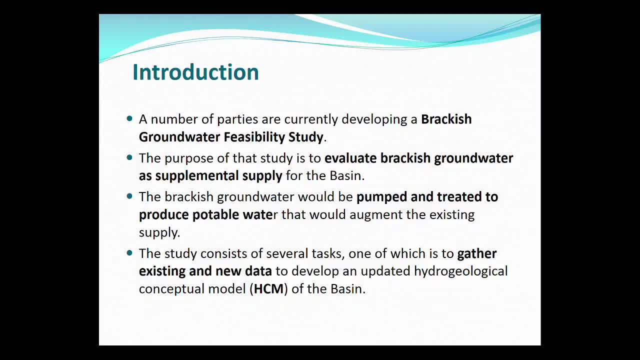 You saw them on the first panel there. COSO Geothermal, Indian Wells Valley Water District, Seals Valley, Minerals and Mojave Pistachios and Meadowbrook has been involved as well. The purpose of the study is to look at brackish groundwater as a supplemental supply for the basin. 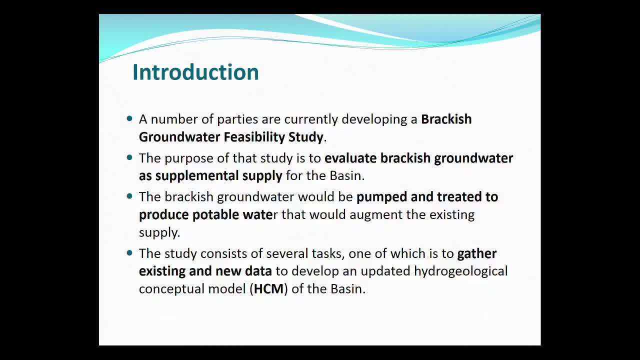 Some people have said it's not a new source. There's that back and forth, but the reality is it's another source within the basin that we can use, perhaps to offset some current use of potable water, and that, of course, would help extend the window, if you will, for us to help solve our sustainability issue. 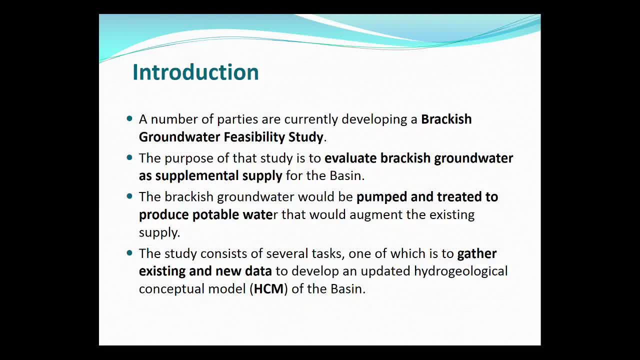 Brackish groundwater would be pumped and treated to produce potable water that would augment the existing supply. I already alluded to that. The study consists of several tasks, one of which is to gather existing and new data to develop an updated hydrological conceptual model of the basin. 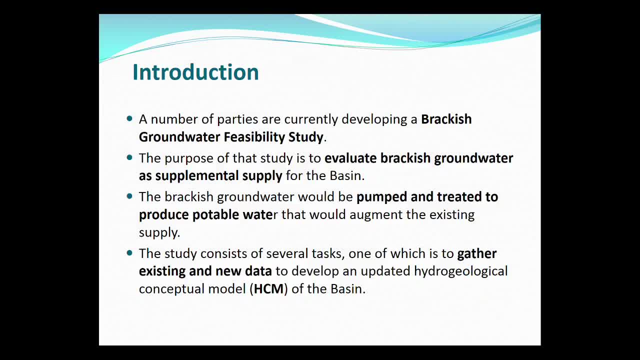 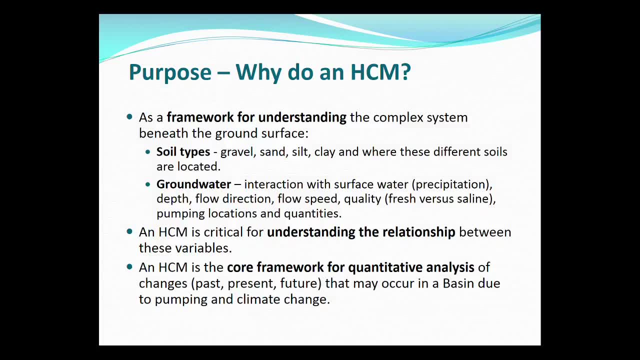 As I said, and then we do plan to bring that to Ridgecrest in July, July 20th. So why do a hydrological conceptual model? It's a framework for understanding a complex system that's beneath us- It will do. It designates soil types: gravel, sand, silk, clay, other types of formations. 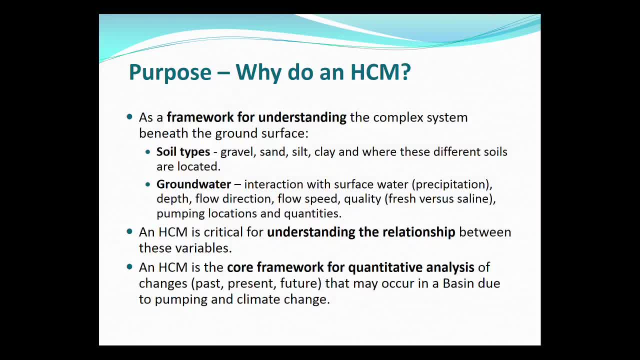 groundwater, the interaction with surface water, depth, flow direction, flow speed, quality- fresh versus saline- and pumping locations and quantities. A hydrological conceptual model is critical for understanding the relationship between all those variables. The hydrological conceptual model is also a core framework for quantitative analysis. 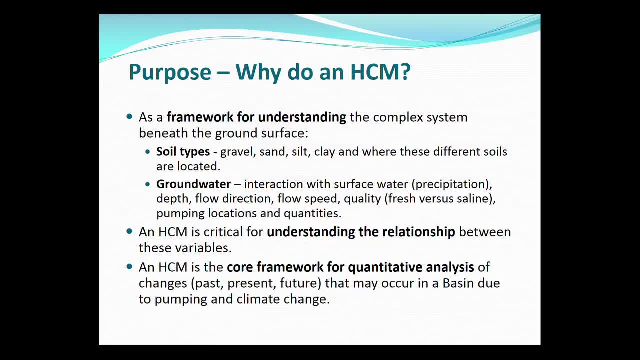 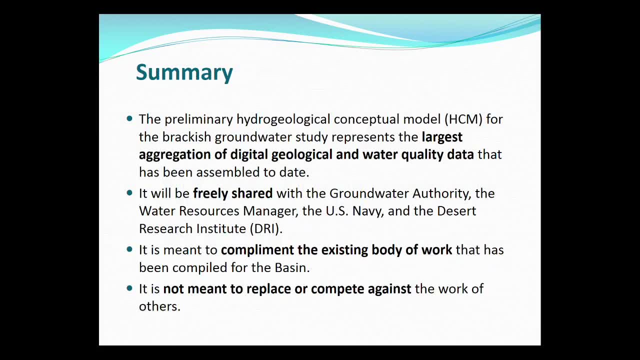 analysis of changes past, present and future that may occur within the basin due to pumping and climate change. The preliminary hydrological conceptual model for the brackish groundwater study will be the largest aggregation of digital geological and water quality data that has been assembled to date. 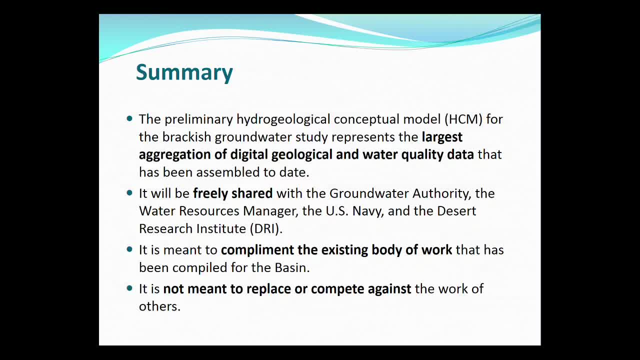 I want to make a point, to stress this: It's going to be freely shared. It's going to be shared with the Groundwater Authority, with the Water Resource Manager, with the Navy, with Desert Research Institute. Again, I want to stress that this isn't an attempt to have a competitive model. 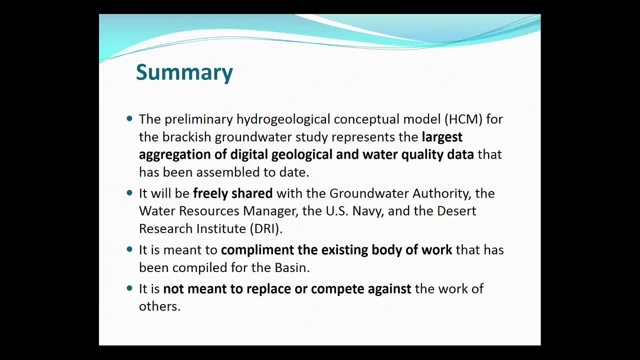 with the model that has been developed by Desert Research Institute, But it will have additional information that we can hopefully provide to the Groundwater Authority for their consideration to perhaps include in the model that DRI has updated. So, again, it's meant to complement. 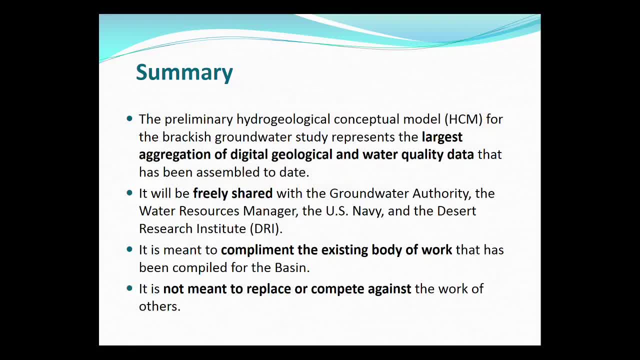 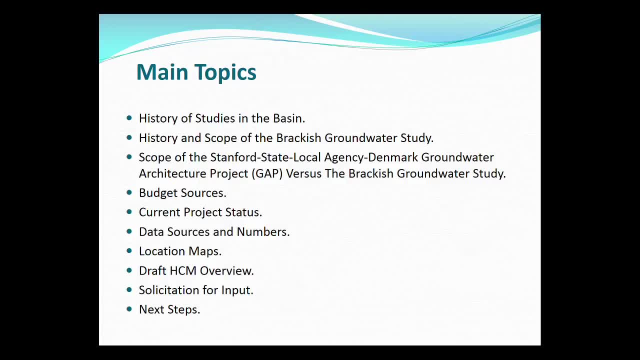 It's meant to complement the existing body of work, not to compete against it. Main topics for today: history of the studies in the basin. a history and scope of the brackish groundwater study. scope of the Stanford Groundwater Architectural Project. 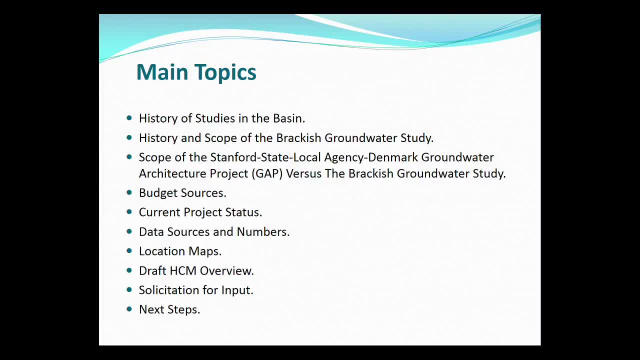 We call it the GAP Project. So if you hear that acronym, Stanford GAP- that's what we're talking about And how that is different and how it in some ways is similar to the brackish groundwater study Budget sources where the money's coming from. 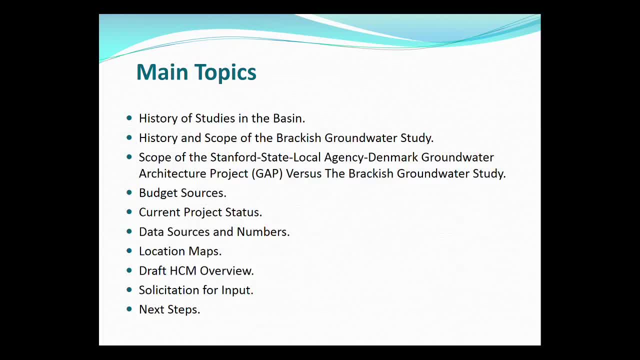 the status of the project where we're at currently. We'll share with you data sources and numbers, location maps, a draft of the hydrological conceptual model overview, I think, going forward, I'm just going to say HCM Solicitation for input and next steps. 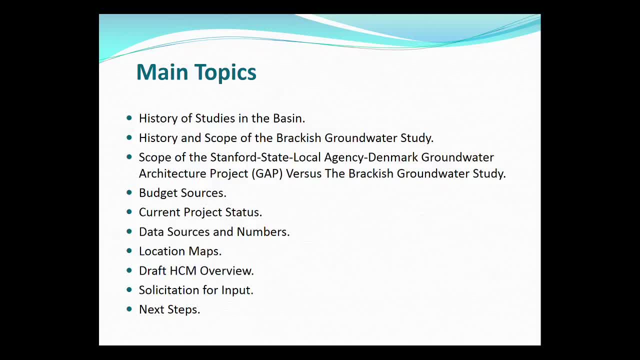 Again, we wanted to share this with Members of the TAC, members of the PAC, DRI, and I think they are involved, they're listening in on this And get the input, Show you what the interpretation is and see if it makes sense to you. 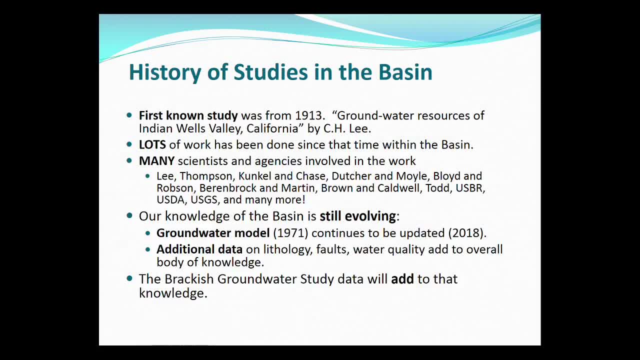 So that's the objective, one of the objectives of this meeting. So I'm going to just go through a couple slides and I'm going to turn it over to our team here. History of the studies in the basin: The first known study was from 1913,. 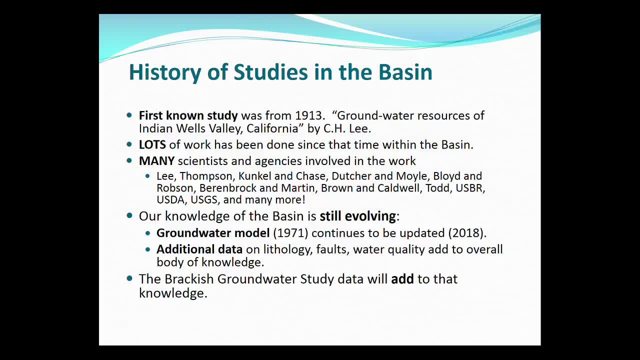 Groundwater Resources of Indian Wells Valley, California, by CH Lee, If I'm not mistaken. we have a handout, don't we, that has a list of all the studies and resources. If you didn't get one, Tim can pass them out. Tim and Max. 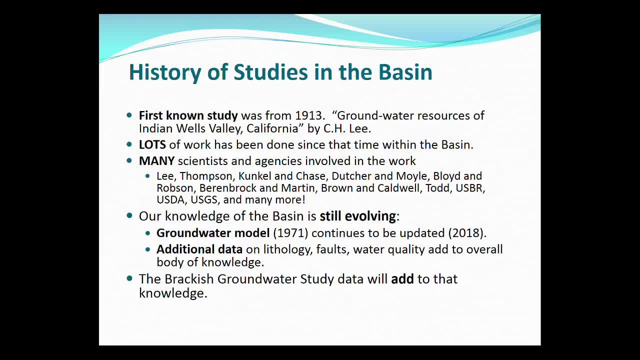 There's been a lot of work done within the basin within this time. since that time- and the paper that you're getting right now is evidence of that- Many scientists and agencies have been involved and you see on the screen some of the examples. 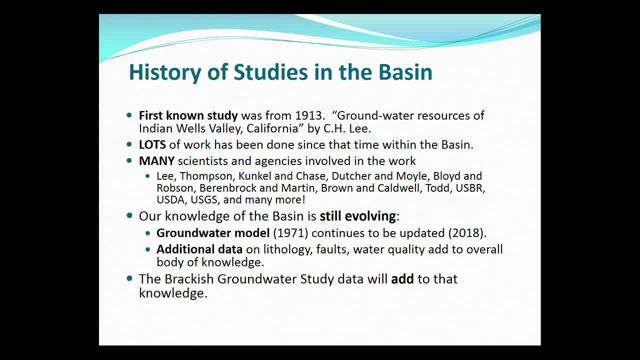 These are on your list, Thank you. It says on here: the knowledge of the basin is ever-involving. If you were here today- and I think most of you were- you heard the USGS present the results of their groundwater recharge study. 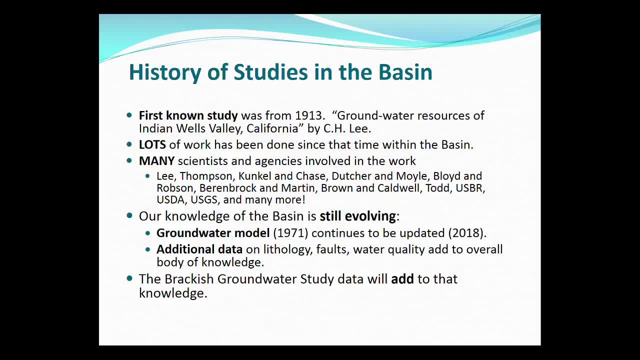 The SkyTem work is another example of more evolving information and the brackish groundwater study is another example. The original groundwater model was from 1971, but it continues to be up. The most recent update was of the Brown and Caldwell model. 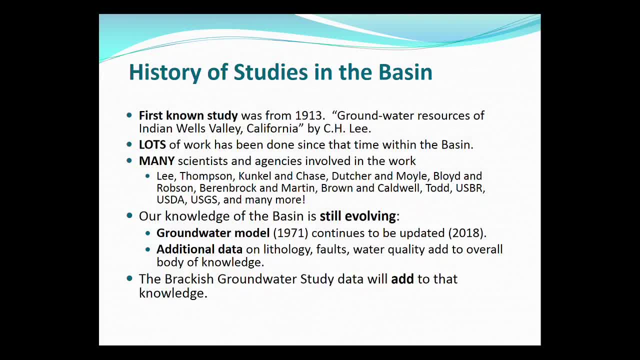 which I think was done in. was it 2010?? I'm looking at where Renee is here. Anyway, that was the model that the base used as their basis for updating The brackish groundwater study will add additional data to our knowledge of the basin. 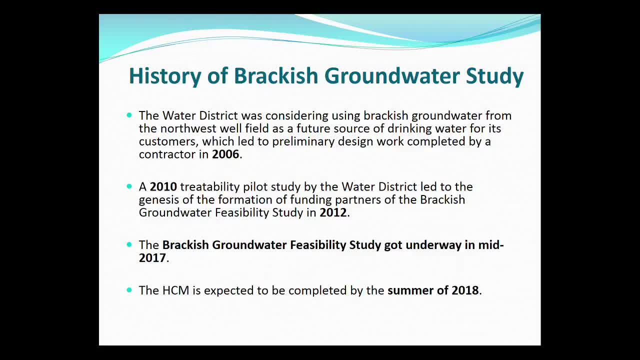 So just an overview of the brackish groundwater study. The water district was considering brackish water, has considered brackish water for many years as a potential source from the Northwest Wellfield to actually serve our customers. to treat it and serve our customers. 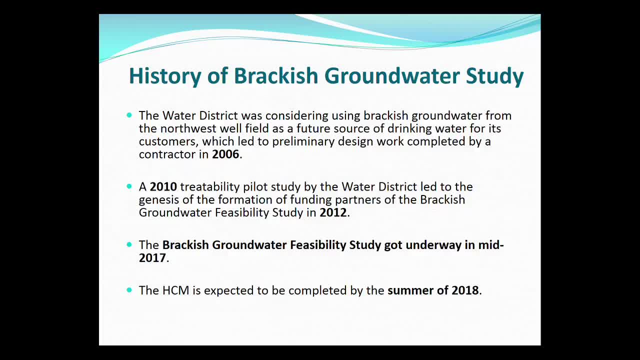 There was preliminary design work done in 2006.. Since I came on board in 2012,, and maybe even a little bit before that, the district has been looking to do a further study and we actually developed a cost to do that study. 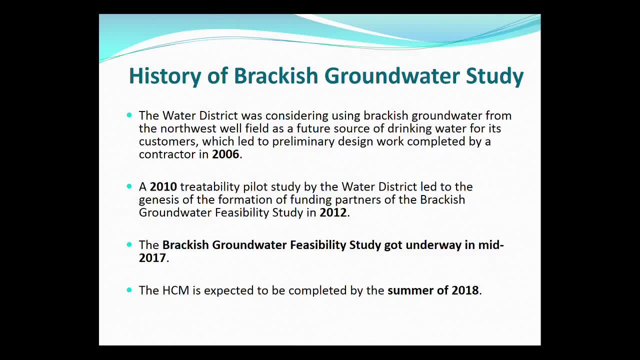 and my recollection was it was somewhere around $400,000 to $420,000, and we were looking for partners to do that study. Initially we were going to try and do it ourselves, but then we thought it would be better and more beneficial. 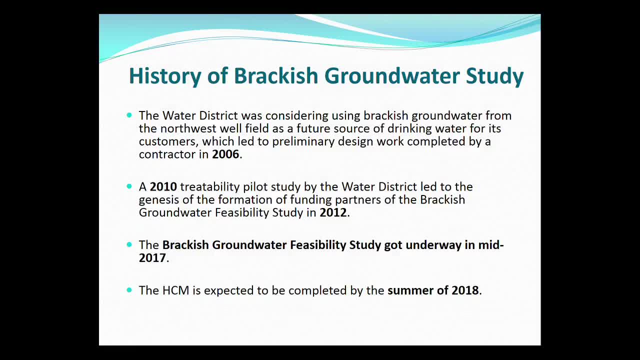 if we involved more people. So, as it says here, a 2010 treatability study was done by the district, which led to the formation of some funding partners for the brackish groundwater feasibility study in 2012.. That's when initial conversations were held. 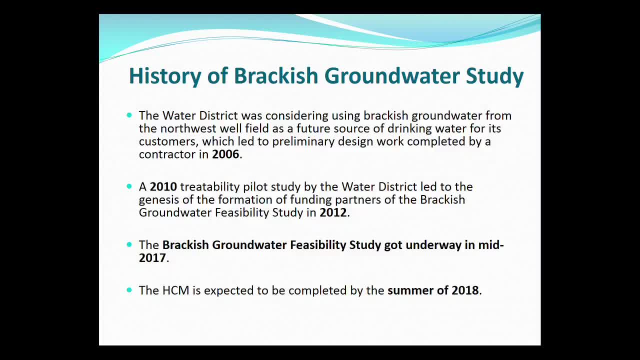 in October 2012, about the possibility of using the brackish water resources, First of all defining where they are, how much is there, and once you do that, then you can determine if it's feasible for the cost to treat it and use it. 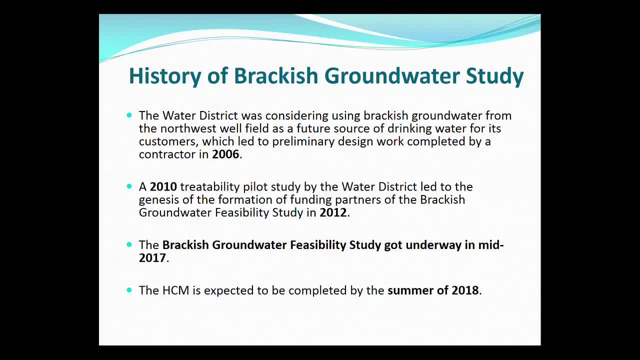 Excuse me, Hello. Hi, this is Jean, and somehow we're not able to get in on the WebEx- neither DRI nor Stetson- And I was wondering if there's a way to address the WebEx. We have our IT person coming out of his hiding place right now. 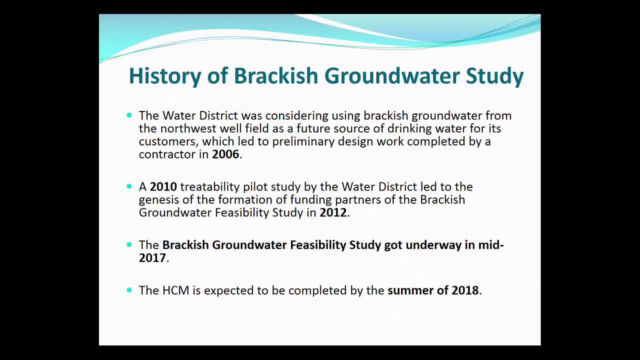 and hopefully we can get it addressed. You're not missing too much in the slides, but hopefully when we get to the data part we'll get that corrected Right. exactly That's why I interrupted. We're all able to hear. 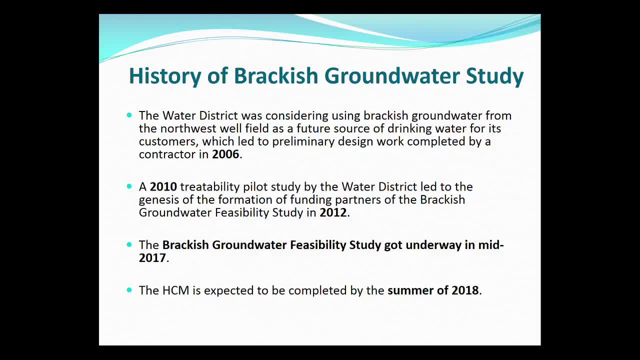 and somehow the meeting number says that it hasn't started yet. but it hasn't started yet. Okay, They are working on it as I speak. Okay, thank you. Okay, I think I've just got a little bit more. You probably don't need to see the slides. 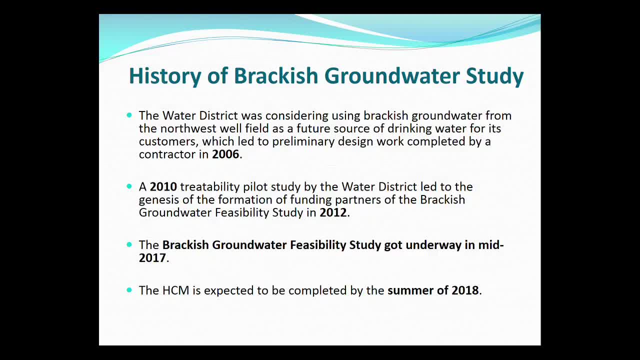 and you probably don't need to see me. So the brackish groundwater feasibility study got underway in mid-2017.. We submitted a grant application for Prop 1 funding to the Department of Water Resources and we were successful in actually getting more than we needed. 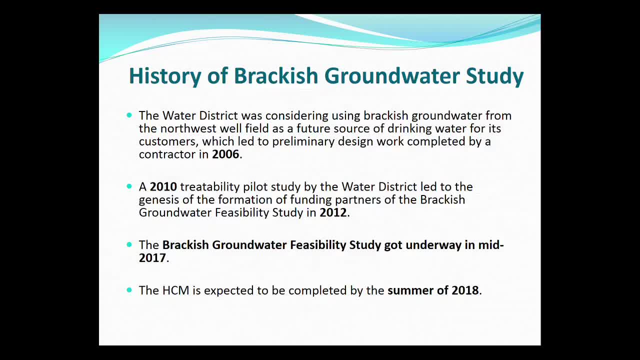 Very rarely do you get more than you ask for, but we were awarded $1,084,000 for this study, so we were very happy to do that. We do expect the model, as I said, to be completed by summer and, as I said, in case you came in late, 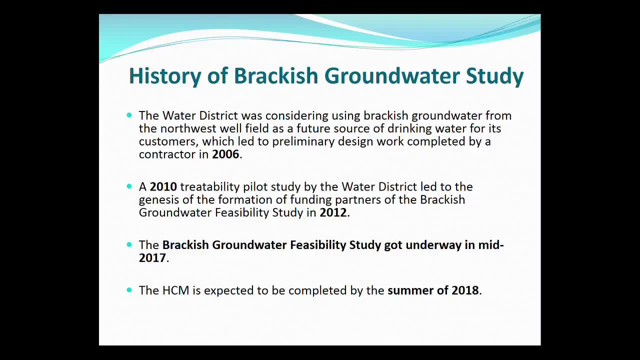 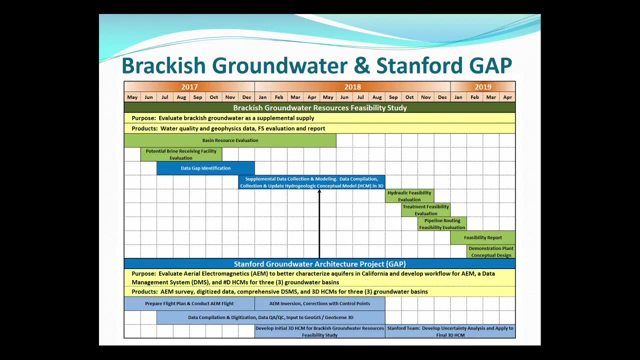 the intent is to share that at a meeting July 20th, which is a Friday, at 9 o'clock here in council chambers. Now I'm having technical difficulties. Oh, there it goes, Okay. So at this point, hopefully we've gotten it fixed. 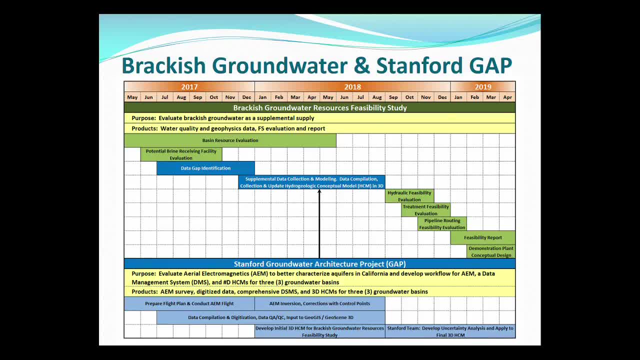 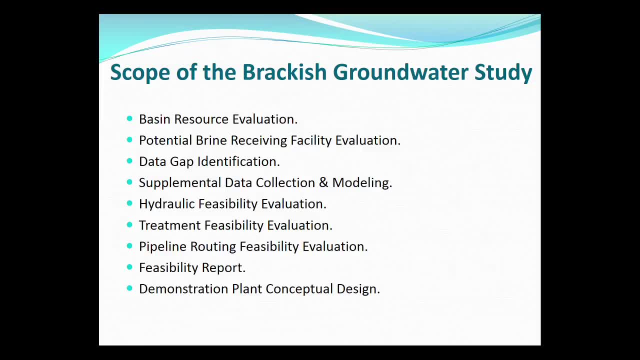 and I'm going to turn it over to Went too far, Oh Okay, So I'm going to turn it over to Tim Parker, now in his capable hands, and here he is, Thank you. Thank you, Don, for that introduction. 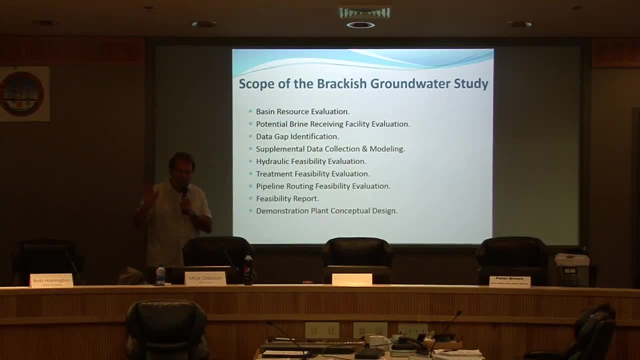 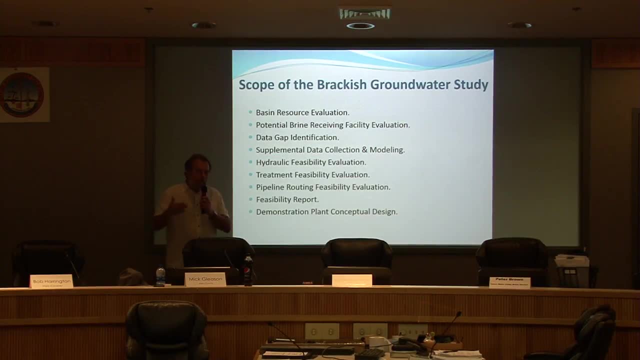 And we'll get this worked out behind the scenes. Don't worry about that. We're here to. Actually, we wanted to take this time to actually give you information on this and get your input, So that's why we're here. 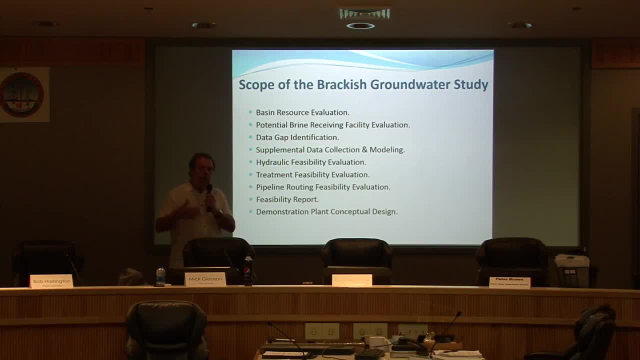 We're interested in getting feedback on what we're doing, the data we've compiled, and then we're not going to get into too much interpretation today, but we are going to talk about the data and the challenges we have with the data And my experience here. 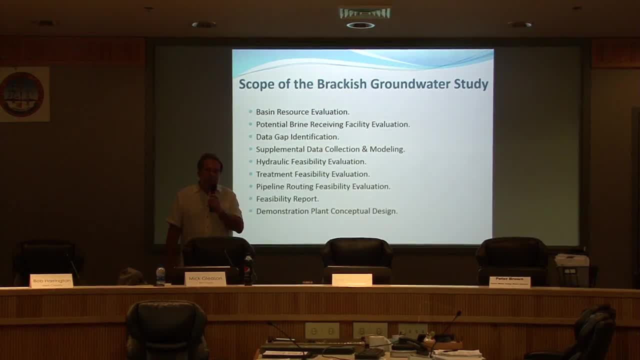 and this valley has been that there hasn't been this kind of a comprehensive effort to bring all the data into a 3D model, And you'll see what I'm talking about when we get there, but anyway. So this is the actual scope. 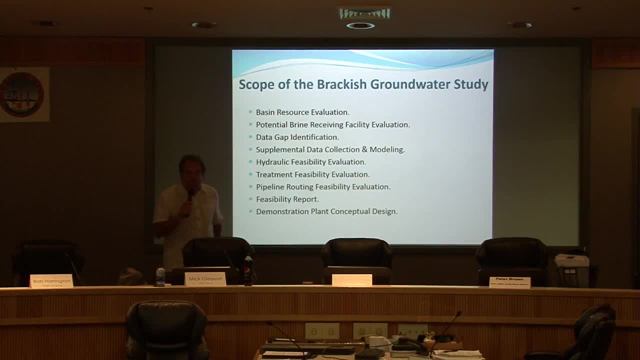 of the Brackish Water Project. So it's a resource evaluation, a potential brine-receiving facility evaluation, a data gap identification, supplemental data collection and modeling, a hydrologic feasibility evaluation, a treatment feasibility evaluation, then a pipeline routing feasibility evaluation. 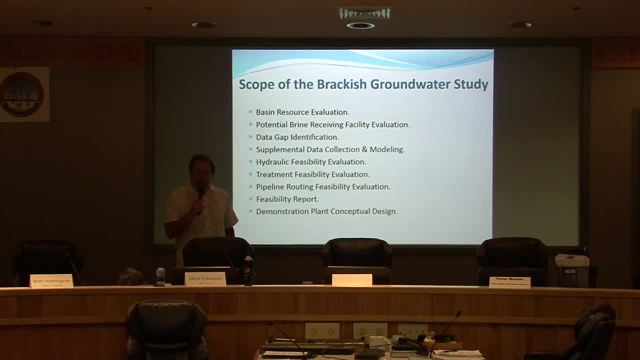 then there'll be the feasibility report and then a demonstration plant conceptual design. So that's it in a nutshell. It's a lot, but And I'm going to just kind of go to that diagram that Don has just given us, And I'm going to just kind of go to that diagram. 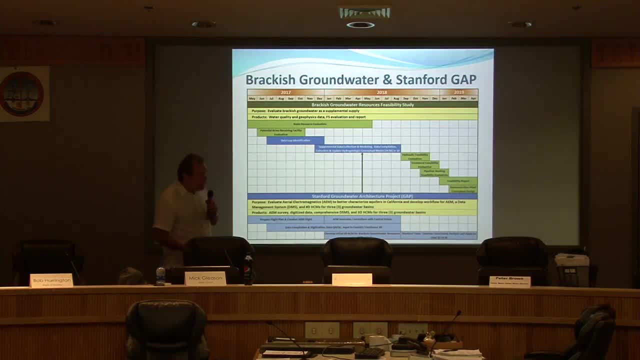 And I'm going to just kind of go to that diagram Don had up before. There we go Now. this is going to be hard to see from back there, but we will put this on the web and I'll talk through this. 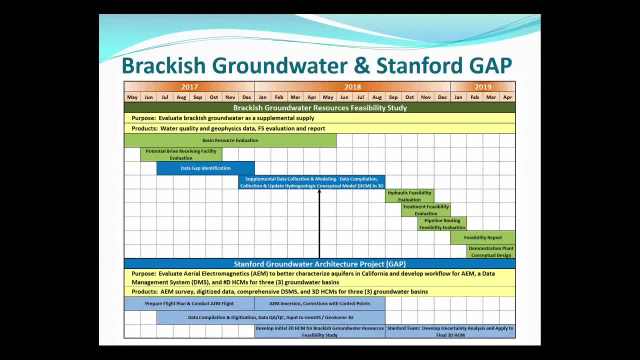 The two main points I want to make initially is this: outlines the Stanford Gap Project, which is actually a component of the Brackish Water Project, And that is the Gap Project is these blue bars and it's data gap identification and supplemental data collection and modeling. 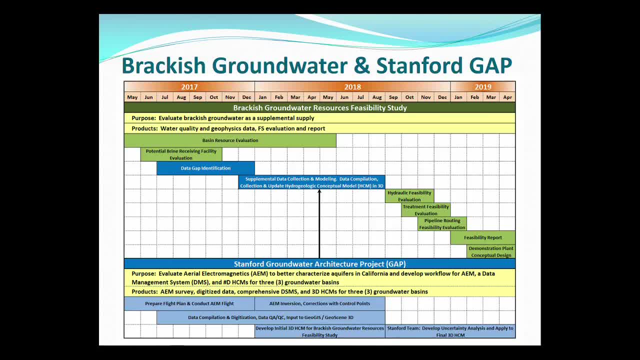 data compilation and then updating the hydrogeologic conceptual model in three dimensions, And so the start of that project, and my compadre over there, Max, is going to get into a lot more detail on the SkyTemp survey and the preliminary results. 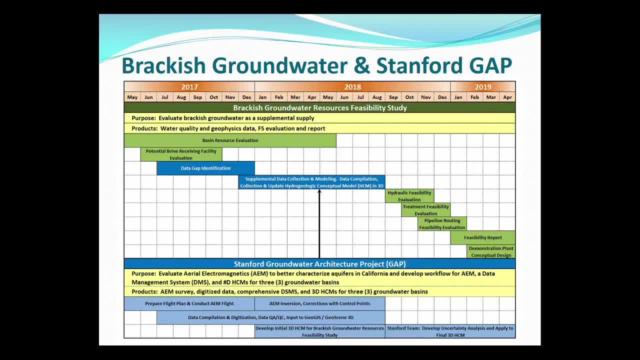 But that was the And it wasn't a black helicopter. but it was a black helicopter. it was a helicopter flying around to do aerial electromagnetics, And Max is a geophysicist and he's going to provide more detail on that. 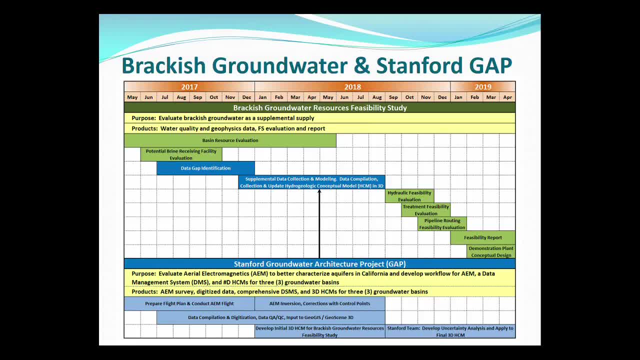 But that's to better characterize the aquifer here. And then there's the development of a data management system. so all the tabular data that's in paper, the drillers logs and everything, and I'll get into more detail on that. 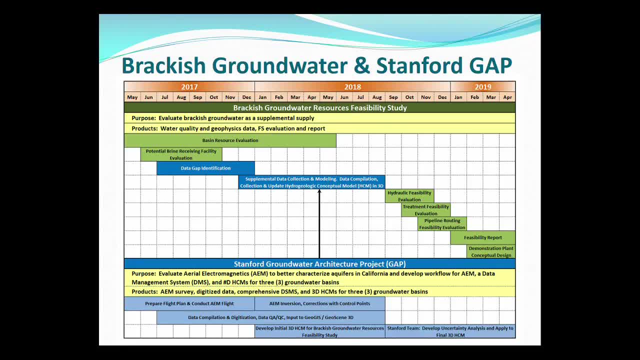 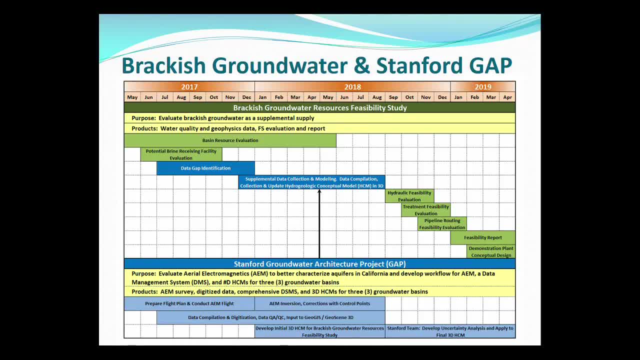 then it's very easy to put that into your model and update it electronically. This hasn't been done here before in this basin. So then the other product is this 3D hydrogeological conceptual model, and it's HCM. we're going to call it. 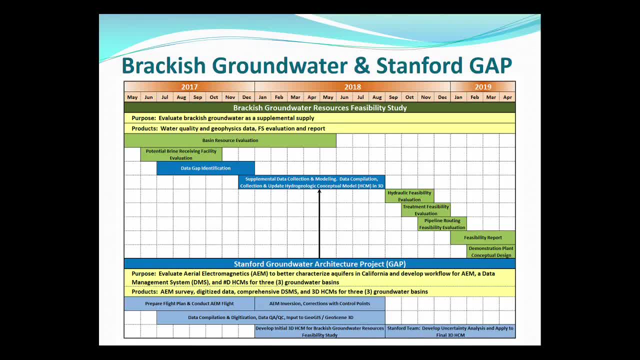 So this Stanford Gap Project actually involves Stanford, the Kingdom of Denmark they call themselves- they're laughing over there- and then it involves the state of California Department of Water Resources and the State Water Resources Control Board and then three local basins. 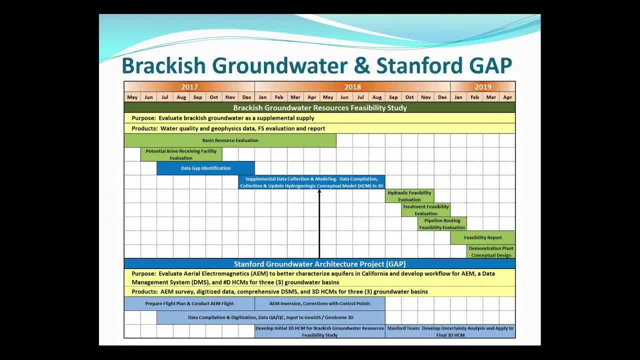 Indian Wells Valley is one of them, And so that is kind of a kind of a briefer on that Now. I should point out: so this goes from the middle of 2017 to April 2019.. And you can see the different components. 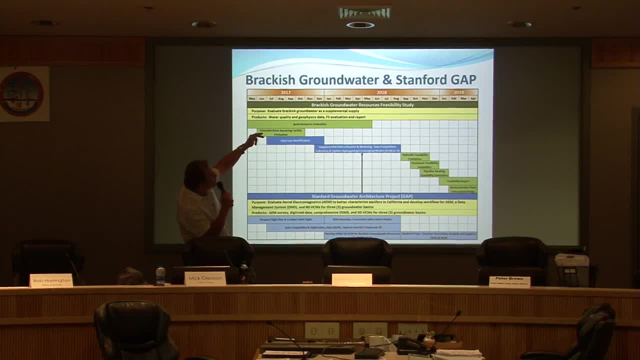 that we mentioned earlier: the basin resource evaluation, potential brine receiving data gaps, et cetera, all the way down to feasibility report. That's where that ends. It's planned to end to be wrapped up in April of 2019.. 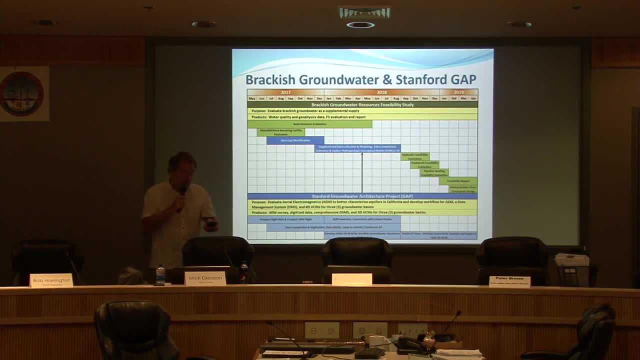 It's a big project, so could go a little earlier, could go a little later. I didn't say the three basins. I said there are three basins. One of them is Indian Wells Valley, Another one is Butte County. 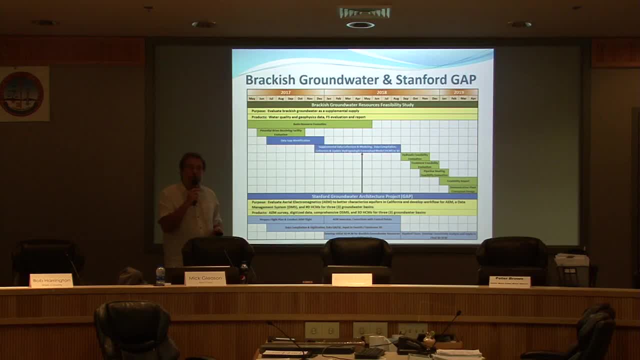 is part of this project And another one is San Luis Obispo County, the Paso Robles Basin. Neither one of those basins have flown AEM yet. They're still in data, they're still in planning phases to actually decide where to do their surveys. 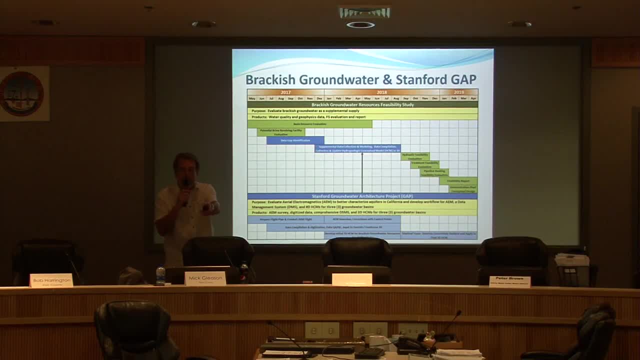 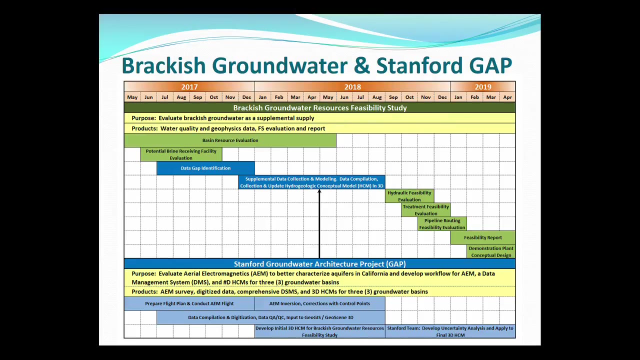 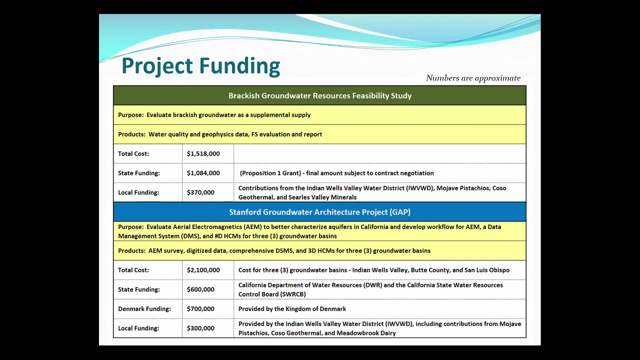 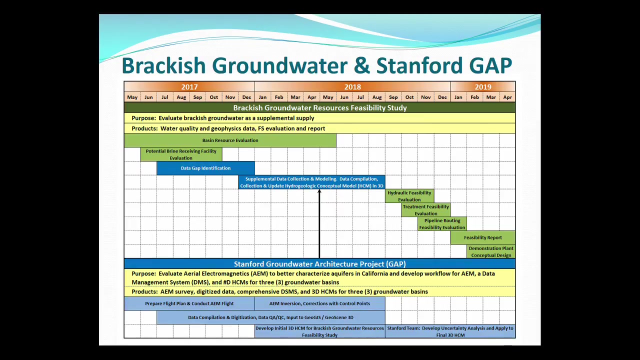 Great, Gary. can you advance the slide? Gary Max or somebody, could you get him to try to? Oh, okay, okay, Hey, how you doing Steve Back one, I think. Oh, okay, Oh wait. 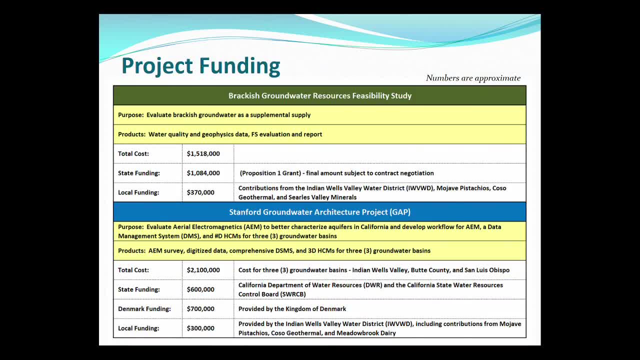 No forward one, That's it Okay. so, as I mentioned, there's the Brackish Groundwater Resource Feasibility Study and then the Stanford Gap Project. This just lays out the funding, in case you can't read it. 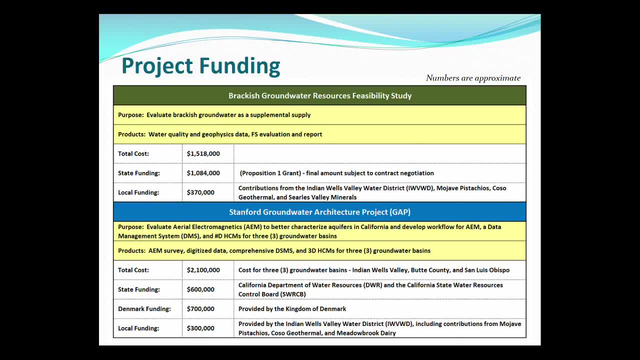 I will tell you. for the Brackish Groundwater Resource Feasibility Study, the total cost $1.5 million, State funding is $1 million. Local funding is $370,000.. And then on the Stanford Groundwater Architecture Project. 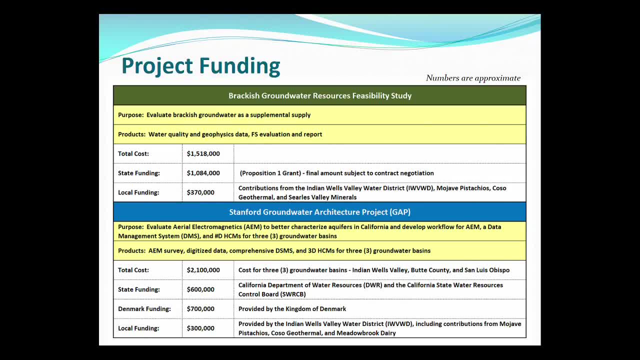 and these numbers are approximate. So it's around $2.1 million. State is funding $600,000.. Denmark's funding over $600,000.. And the local funding here is about $300,000.. So those are approximate, but that's just to lay out where the money's coming from. 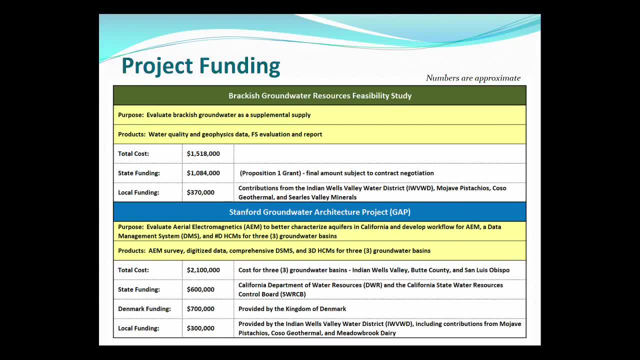 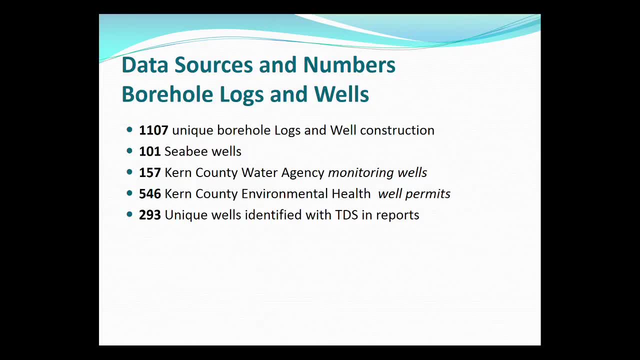 so you know who's paying for it. And now let me talk about some of the data sources and numbers. So we have a a bunch of different data sources that we've had to tap into to compile all this data. We're starting with all the borehole logs and wells. 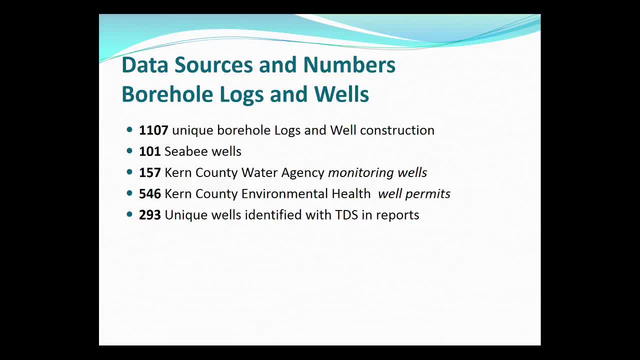 So we've found 1,107 unique borehole logs. This is well drillers' completion reports that contain well construction information About 100 what we call Navy Seabee wells. Seabees are the you know, I think everybody knows who the Seabees are. 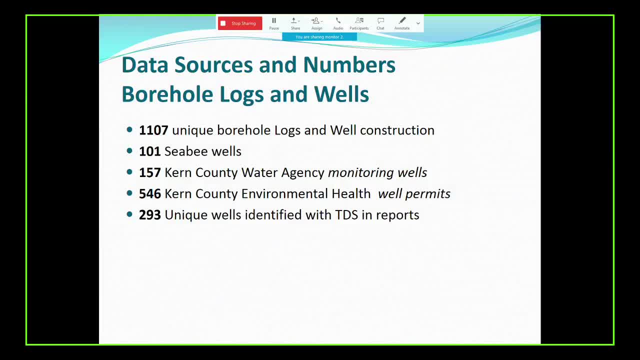 They have a drilling, a training operation here And they basically they provide monitoring wells here. They've been drilling monitoring wells here for a number of decades And so we're very fortunate for that. We have 157 Kern County Water Agency monitoring wells. 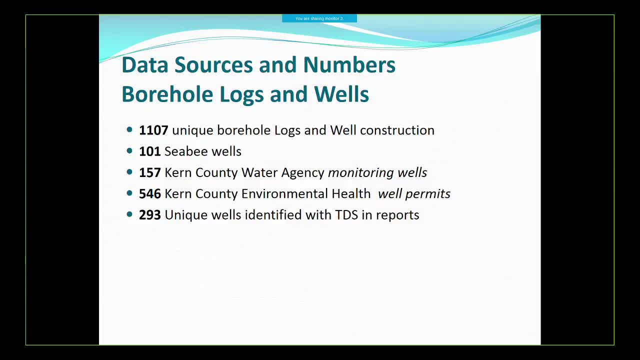 Then 546 Kern County Environmental Health permits for wells. And so again look at the. There's 1,100 drillers' logs. I'll explain that. And then 293 unique wells identified with chemistry, with total dissolved solids and reports. 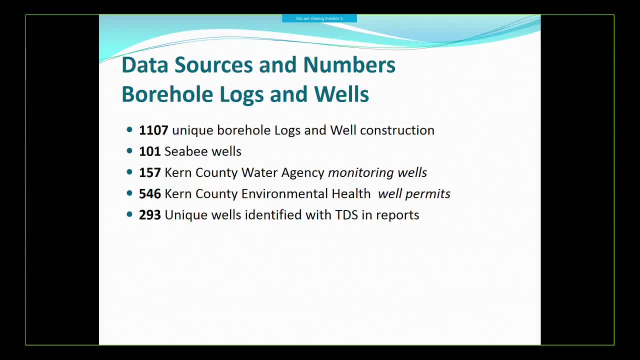 So these are different data sources and they don't all fit together very well: The well completion reports. we rely on DWR to take the information submitted by a driller, which sometimes is a hand-drawn map, to then put in a township range section located with a BLM land plane designation. 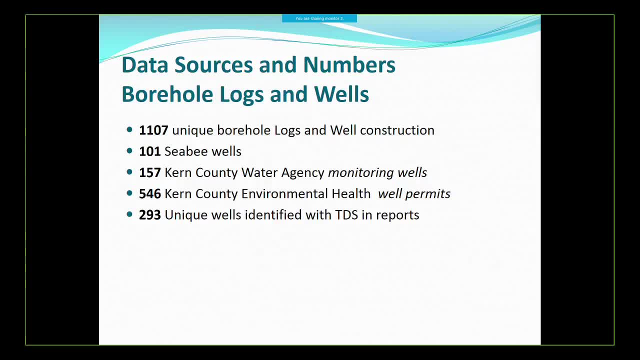 So it's the township. It's the township range, section, quarter section, letters and numbers to locate it. So the problem with that is that DWR got overwhelmed in the 1980s when people started drilling monitoring wells, So they didn't do that much anymore. 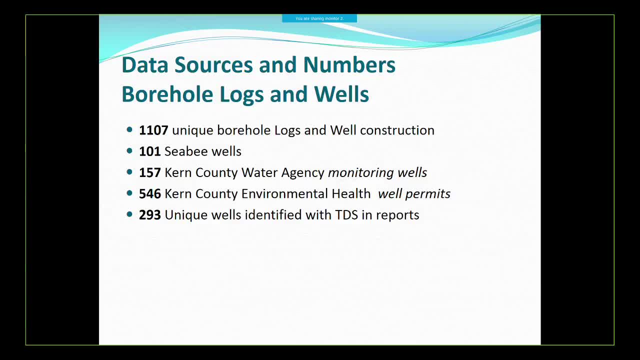 So we've got a lot of well completion reports. we don't have very accurate data on The Seabee wells were in the process of locating, co-locating the wells, The well with the lithology. the Navy's been really good about helping us with that. 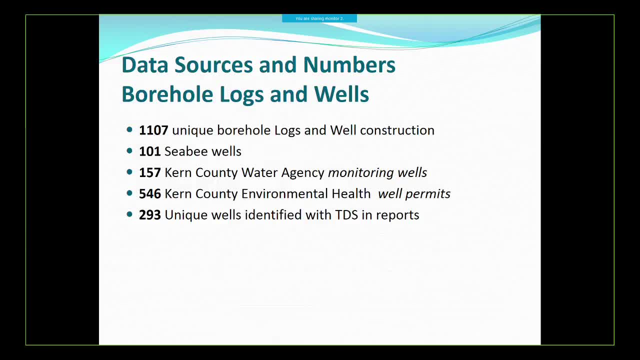 We're almost there. The Kern County Water Agency monitoring wells. the locations are good on those. They went out in the field and located those, but we can't correlate those with the drillers' logs, So we're trying to cross-correlate those. 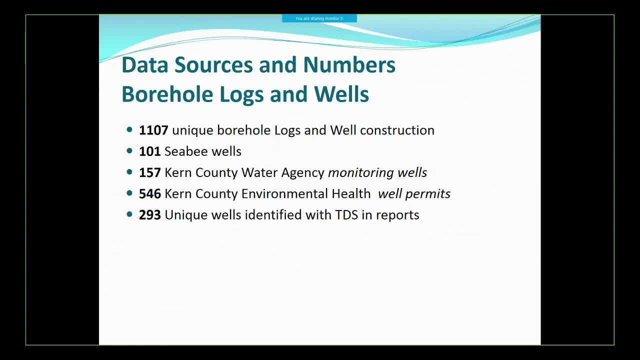 And if anybody's wondering about the CASGEM monitoring wells, that's a subset of the Kern County Water Agency monitoring wells, And then the Kern County Environmental Health Department well permits. well, they've only been doing that, I think, since the 80s. 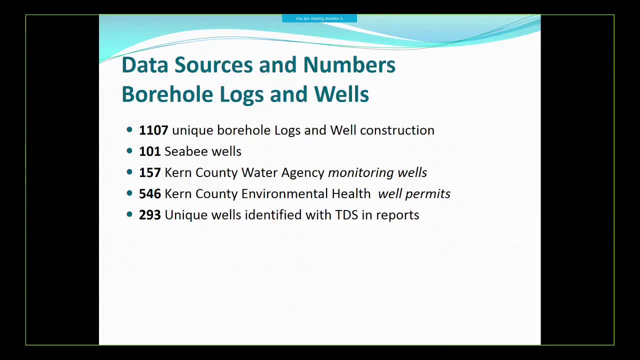 So that helps account for some of that. And then of course, drillers, I think, don't always turn in a permit, but I'm not going to say any more about that. But then the 293 unique wells identified with TDS. 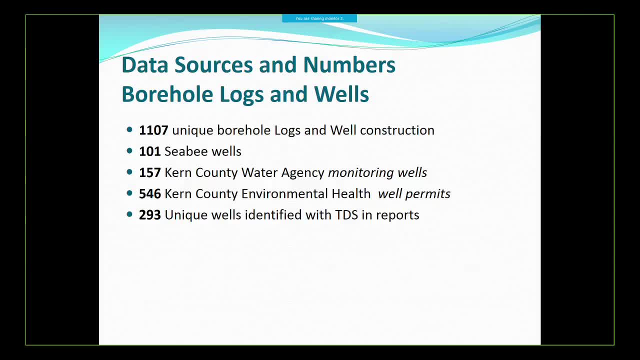 those come out of reports and some of those have coordinates. So we've got this mixture of coordinates we're working through to try to sort out And that's the nightmare that you have in every basin in California if it hasn't been done before. 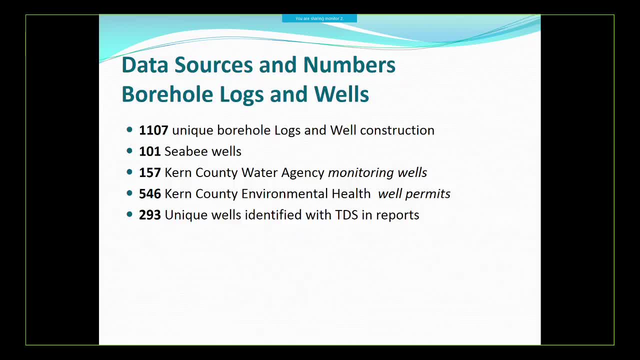 Once you get your house in order and you get a process in place, you don't have to do this again. Tim, this is Jean. If I could just interject one thing, The meeting has started, but it requires a password that we're not able to get in on. 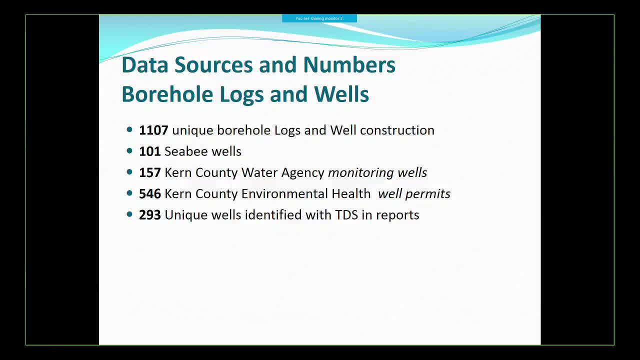 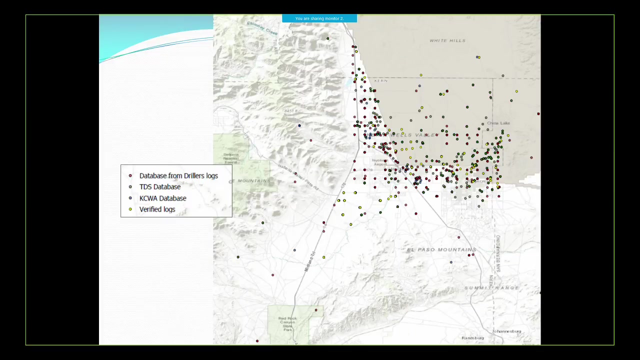 You getting that, Gary? Okay, I think Gary's helping you on that. Okay, good, Thank you, And I guess Gary is going to advance my slides for me because it's not Okay. so here's a map with a good deal of the wells in it. 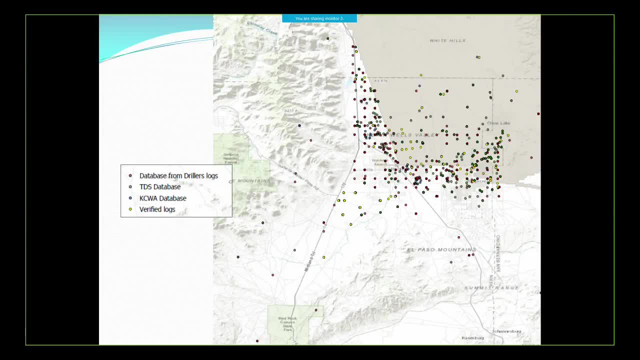 And so it's a database from the drilling Okay logs or the red dots, which I'm sure you can't see from back there. but again we'll make this available: the TDS database, the KCWA database and some of the verified logs. 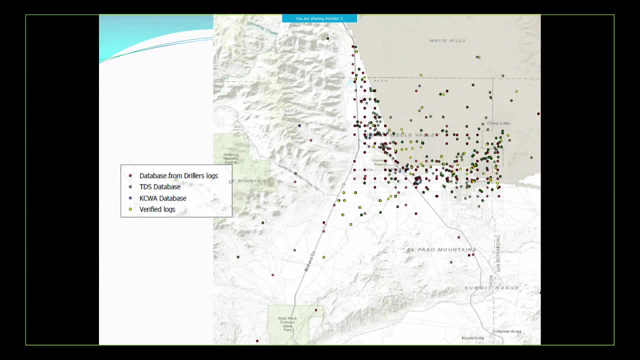 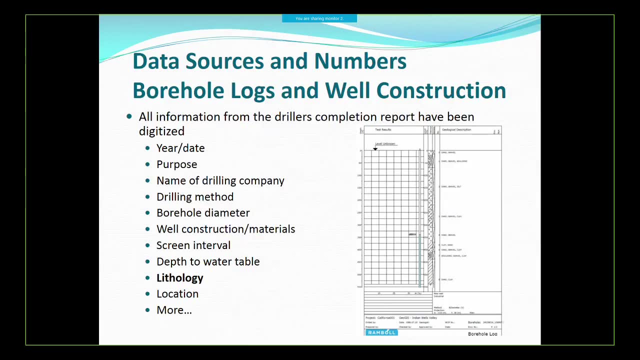 So this will be available in a PDF as well, as there'll be a YouTube, I understand, on Monday, if you want to watch this all over again, and so on Data sources and numbers: borehole logs. So all the information in these borehole logs is listed here. 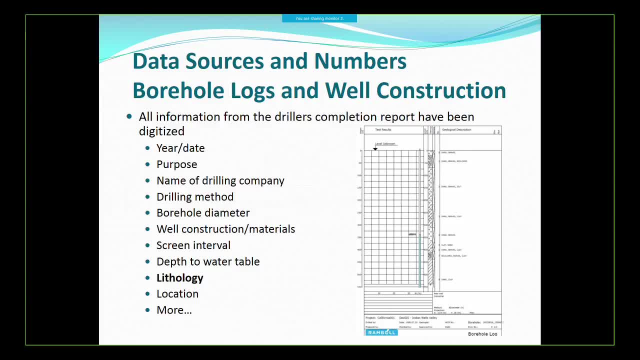 I think I just want to stress the lithology- and you'll see more of this as we move through. You know geology. the lithology controls groundwater flow along with the structure, So that's why it's so important we understand this. 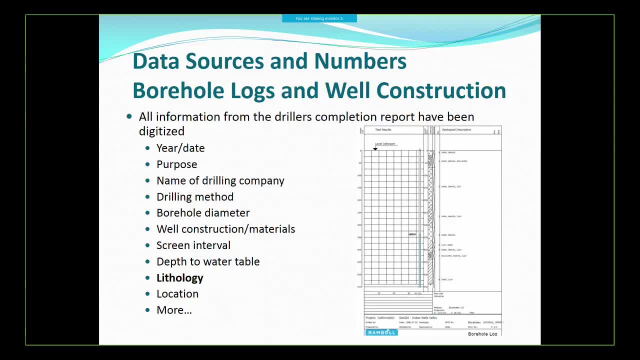 And when you have a model, you make assumptions about how much water is there storage coefficient and how much can it store, And it also affects how it moves. So these things are critical: The well construction and screen interval. if you're getting water levels you need to. 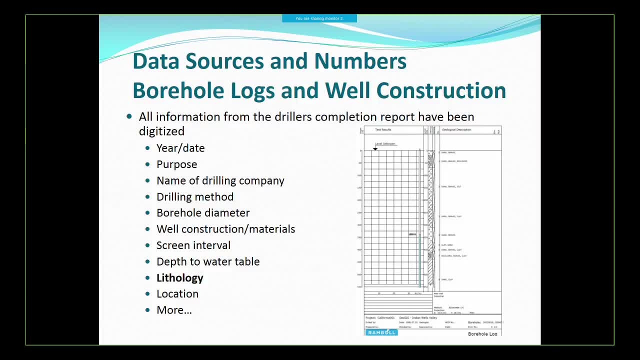 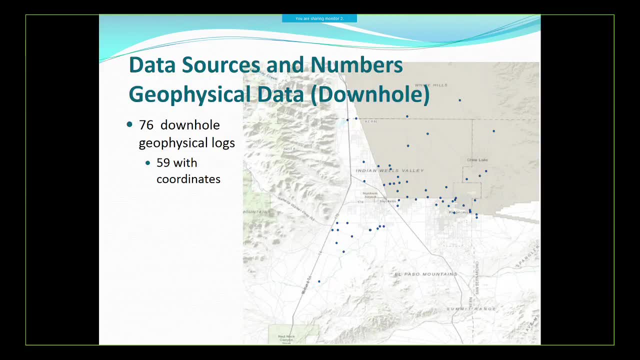 know where you're collecting that information for, and so on. So just wanted to pass that along Now. geophysical data: Lots of wells: when they get drilled, they go out and they do geophysics- downhole geophysics. 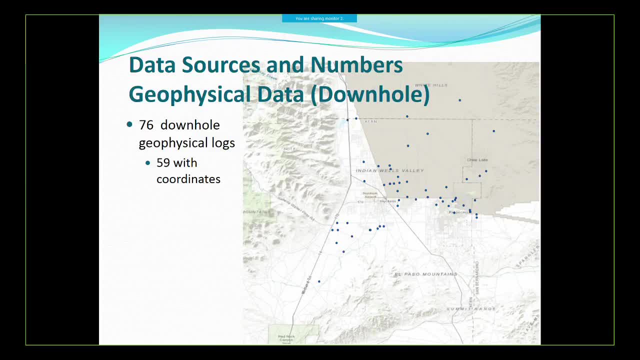 And we have 70 downhole geophysical logs And they're Shown here, 59 with coordinates. Again, we're struggling with locating every one of them, But that's pretty good. These geophysical logs help you understand the geology because you're relying sometimes. 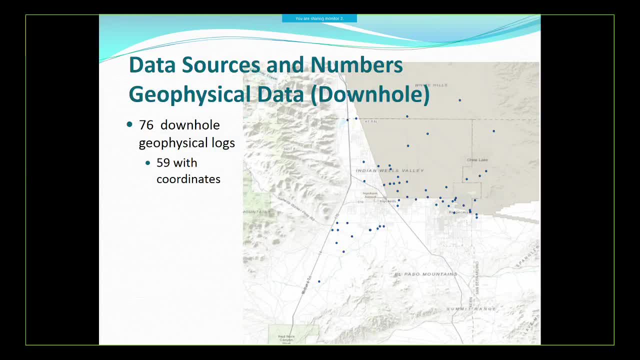 on the driller's description to do that. This is also: You get a consistent measurement from hole to hole so you can help correlate those measurements. And finally, this is going to be very helpful in using the SkyTem data, because now we have 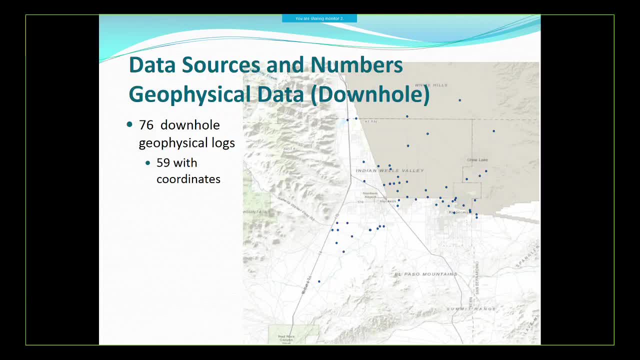 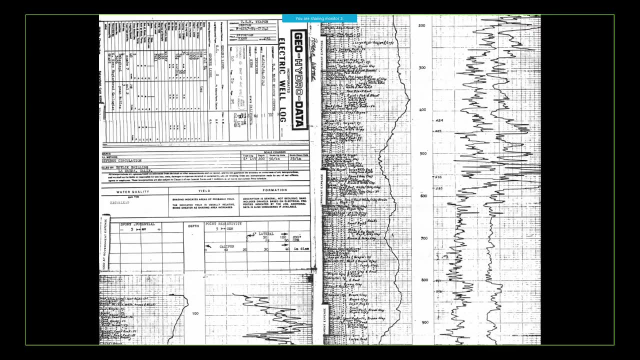 another measurement. As hydrogeologists, we like to have many different types of data. we're dealing with many tools in our toolbox, so this is one of them. This is a very ugly geophysical log, but I just thought I'd throw one of these up in. 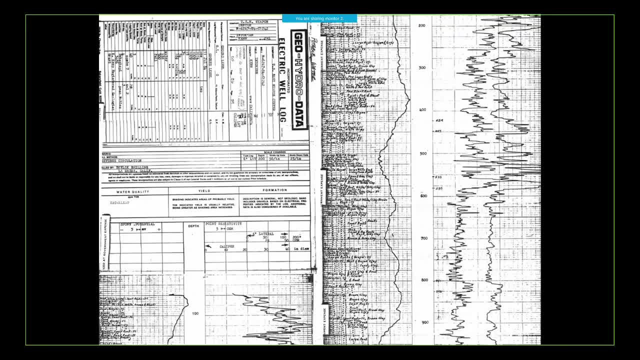 case you're interested in seeing it. So we have a spontaneous potential measurement and point resistivity and those help us understand whether it's sand, silt, gravel or clay- And this is Actually I know this guy, But anyway do we? 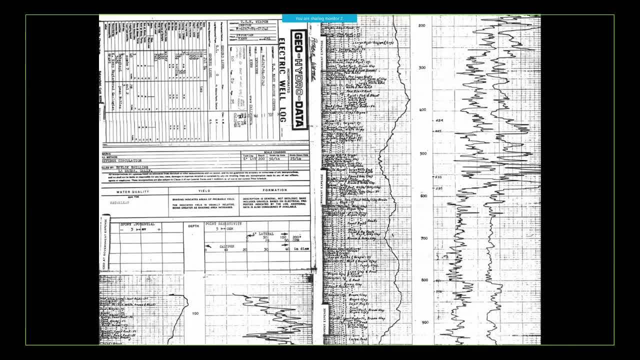 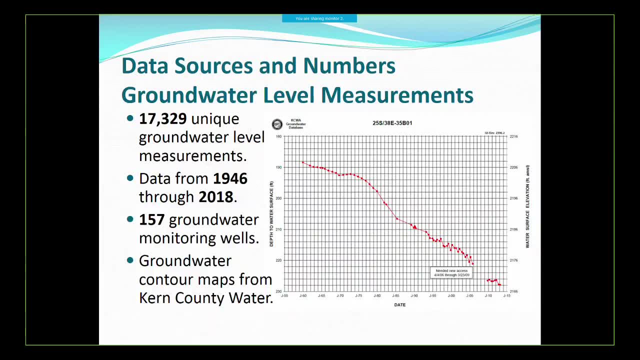 Anyway. so this shows a lot of clay down here and here's some sand and gravel, so you can see how you use these tools to determine and understand the lithology. So now groundwater level measurements. There's been groundwater level measurements collected here for a long time, and so we've 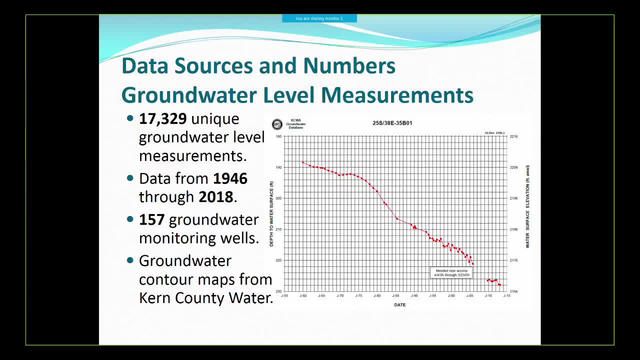 got about 17,000 unique groundwater level measurements. Okay, Okay, Okay. Yeah, Jean, are you there? Yes, I'm there. Can you tell Gary your email address? We're getting there. We're just talking about the data so far. so Gary's walking back to his room. 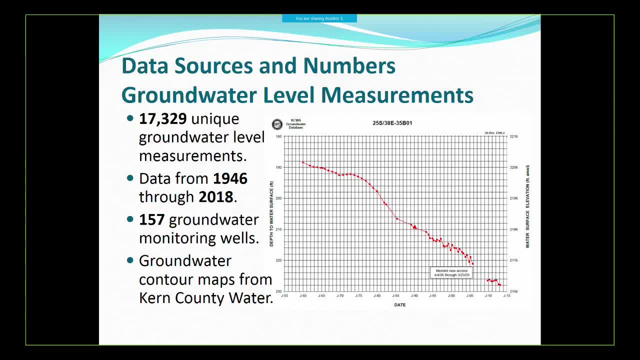 Give him a couple more seconds. Hey, Tim, This is Tim Godwin. I'm also having the same problem. How about you give us the password? Yeah, So we've got two people that need the password. Gary, Four people. 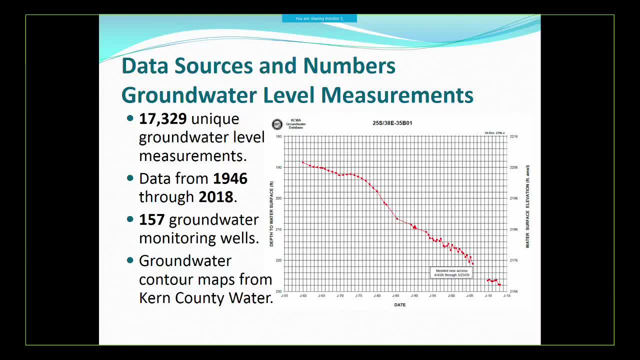 Okay, Is there a text number we can send it to You? can? Yes, Can I say something, Of course? Okay, Sorry, Can y'all hear me, Those of you who are waiting for us to come out of closed session, we're going to come. 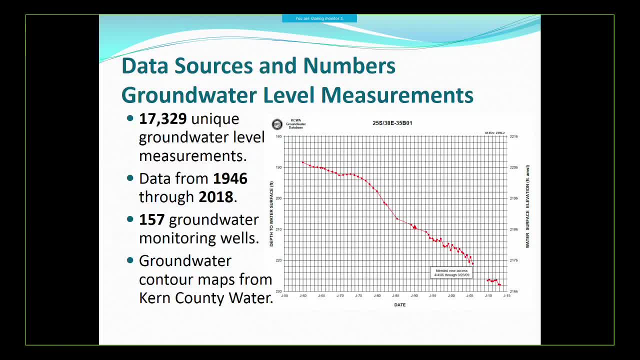 out of closed session. but we're asking if we really want to stay and wait for our meeting, because after this we're asking if any of you mind if we continue the TAC and the PAC report and the ending to the next meeting. Anybody have any objections? 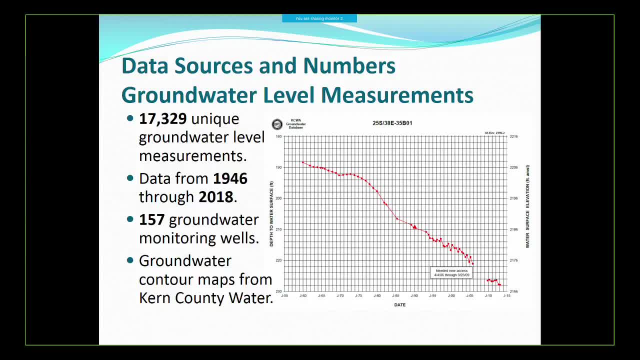 I really want to hear them. if you do, You have Okay, Okay, but I Now is Adam still here, I won't cry. Donna's still here. We've got staff that would like to go home and I understand that. 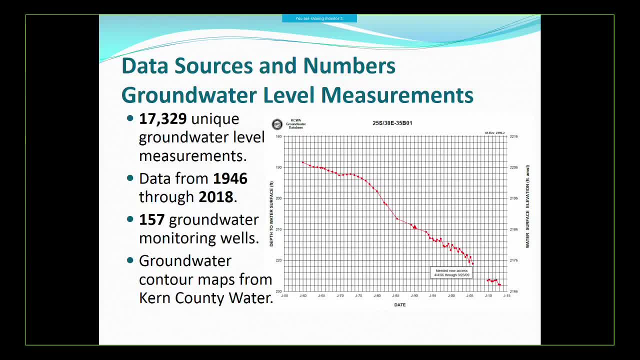 We've got some board members that had to leave because of time. Inyo County- I mean Inyo County- has already left, and so we're trying to figure out how we can do this. We're trying to figure out how we can do this. 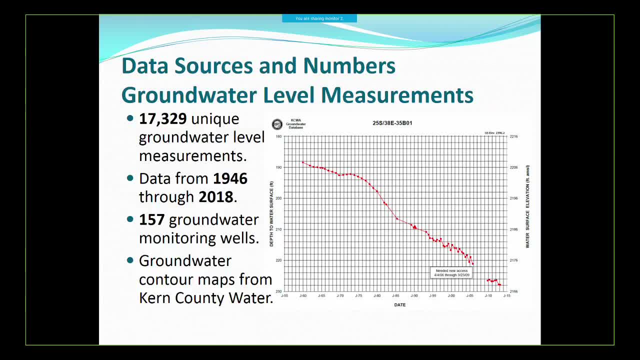 We're trying to figure out how we can do that Well, that's why I wanted TAC and PAC to be able to give the report. So all right, we'll say we'll have TAC and PAC. If you want to stay, I'll make sure we have three board members here and we'll go from. 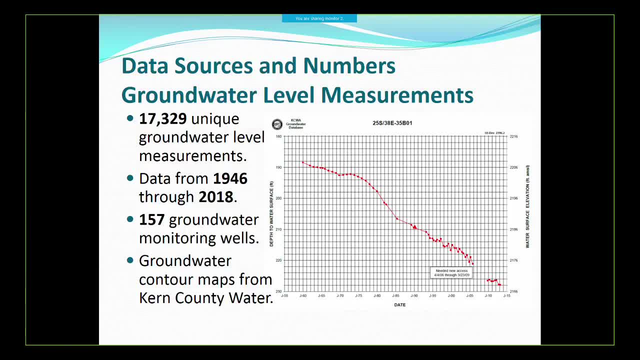 that, I'm sorry, Didn't mean to interrupt. How much longer do you think you're going to need? Ten hours or eight hours? I think we're looking at. We're looking at probably potentially an hour, Another hour. Yeah, just because we've had a few snags and so we're trying to figure it out. 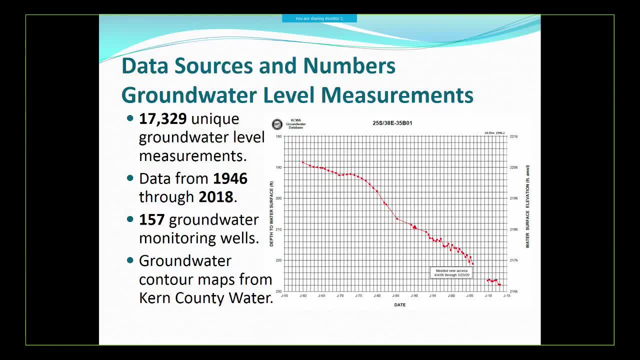 People don't have the passwords, but I see I know I want to come on. That's why I wanted to get done. Okay, Okay, Okay, Okay. So Let me come Okay, And I just sent you their email, a few people's email addresses, so this is juggling. 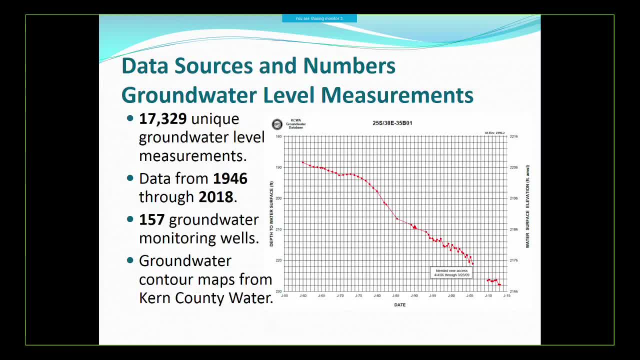 So the password, The password is Okay. Everybody don't listen, Plug your ears, because it's a secret password. Two, two little y cap P, little d. five little y cap B, little d. 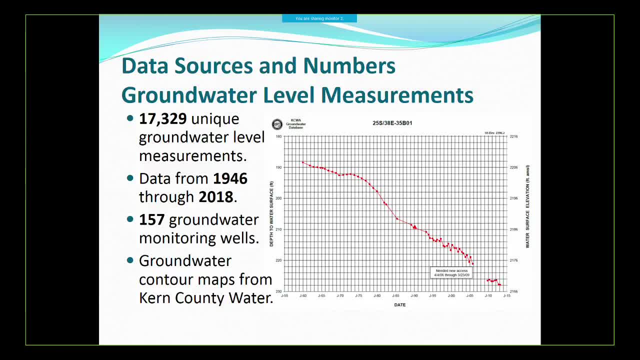 I'll repeat that, okay. Okay, Two little y capital P, d, little d. five little y capital B, little d. Everybody got that, Thank you, You bet, Okay, Oh, I can't see now. 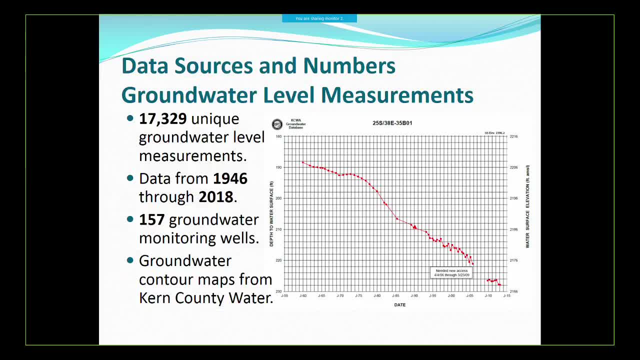 Okay. So, as I was saying, we have about 17,000 groundwater, Unique groundwater, Hello, Okay, Okay, And this is A lot of this has been collected by the Basin Monitor, Kern County Water Agency. So when you think about that, you know they're doing their part in the basin and they continue. 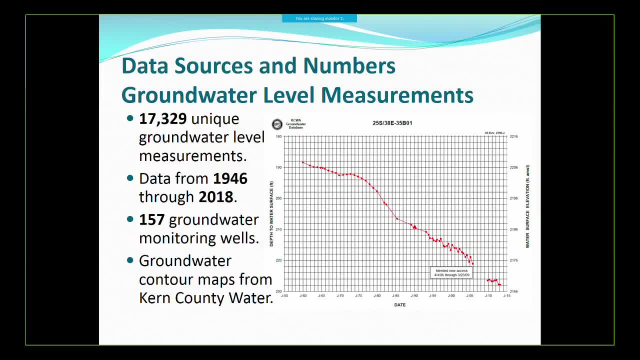 to They're And that comes out of funds they collect from the county. So data from 1946 through 2018, and it's from 157 groundwater monitoring wells, although I'll have to say that a lot of these wells 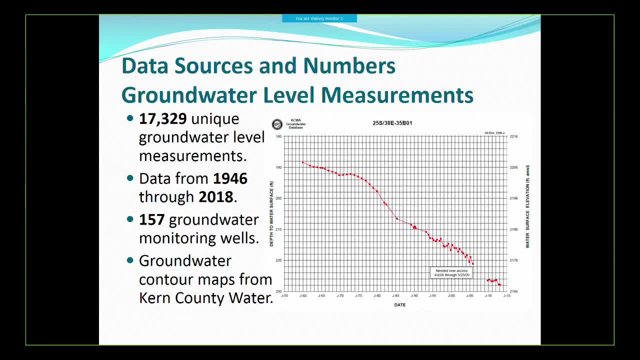 Are either clusters or nested, so there's actually two, three, four different screens in these 157 locations, And then Kern County Water Agency produces groundwater contour maps. This is just an example of what a hydrograph looks like. It's about a 50-year period and this one is going down as you can see. 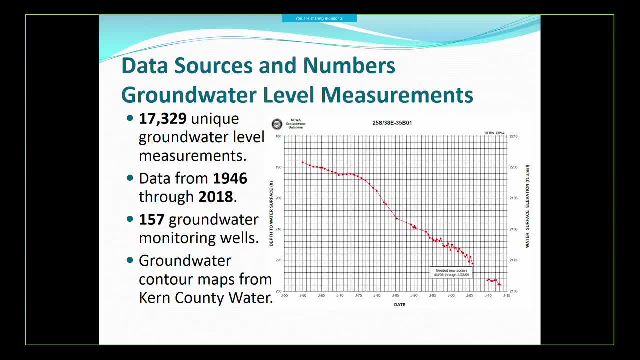 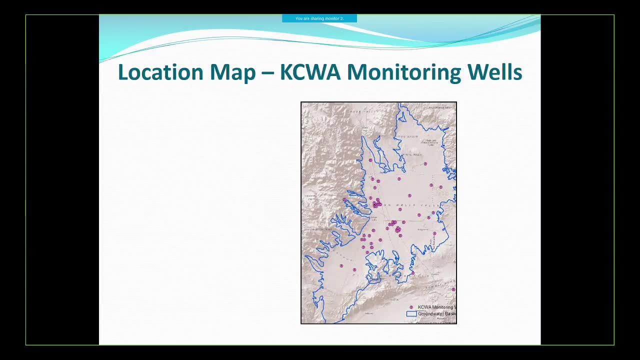 What's the next one? Okay, Okay, Okay, Okay, Okay, Here we go. Here we go. Okay, Okay, Okay, Here we go. And this just shows a map of the wells. We did notice that we had a little bit of problem with the coordinates in the database. 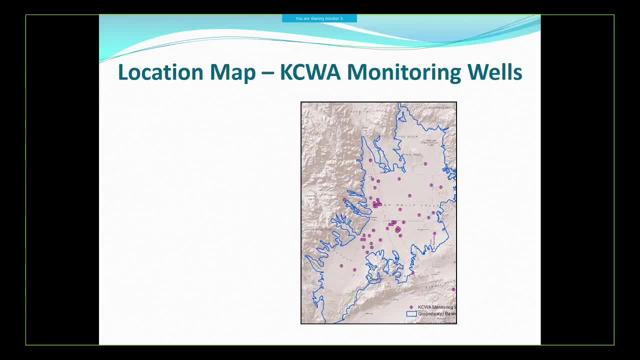 So we're sorting that out. but this shows the approximate location. So again, coordinates and getting everything just right in a GIS system can be challenging. Now Denmark: on the other hand, They've been been putting all their data together since early 1900 in a very exact way. 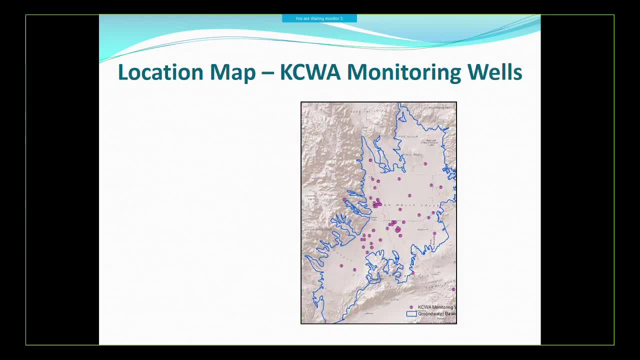 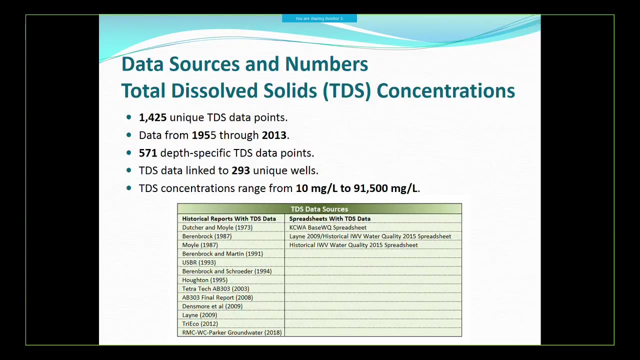 So I don't think Max is going to talk about that, But it's been real interesting having discussions with him as we're struggling through these legacy issues of data here in California And next slide, Poor Gary. So, in terms of total dissolved solids, 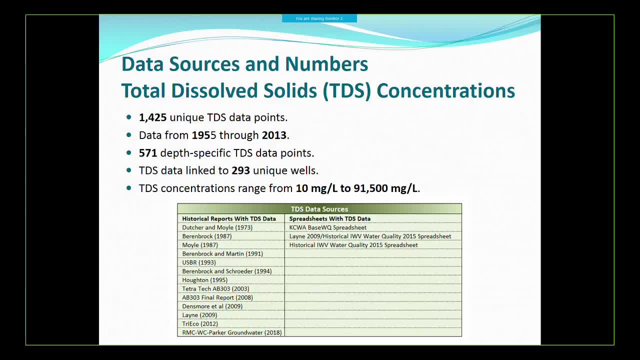 Now that gives you a count of basically the salts. Now I know that's not an exact term, but it gives you a basic estimate of salinity. And so we have 1,425 unique TDS data points, data from 1955 through 2013.. 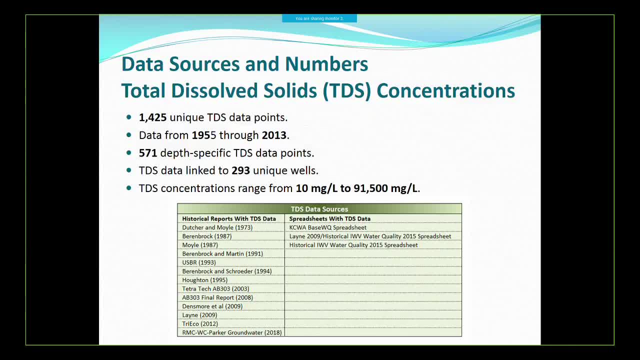 And we could probably extend that- But 571 death-specific TDS data points- And you'll see the importance of that as we start looking at the SCITEM data again- And then linked to 293 unique wells And the concentrations run from ten to up to 91,000, which is basically very salty. 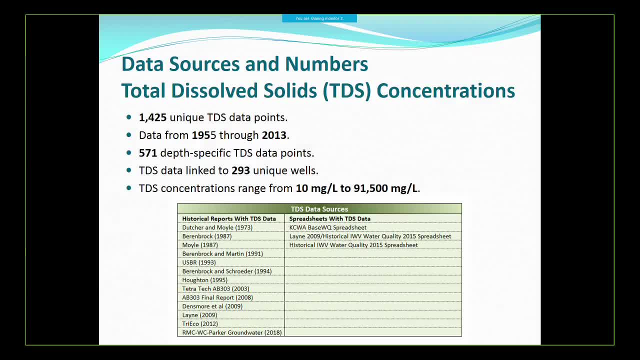 And this just basically shows some of the TDS data sources. I should note- this is a reminder for me- in that document we handed out, it lists a lot of stuff And it's not just TDS-based, And that's not just TDS-based. 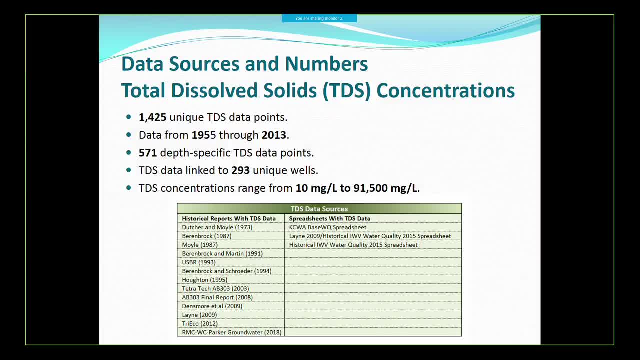 TDS-based requires a special class of binaries, not complete, and we're looking for input from everybody on that. if you think we've missed some reports, if you know of some that aren't listed in there, give them to us. It's also missing some authors. 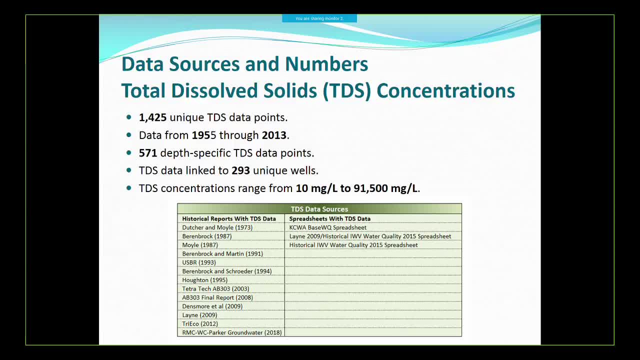 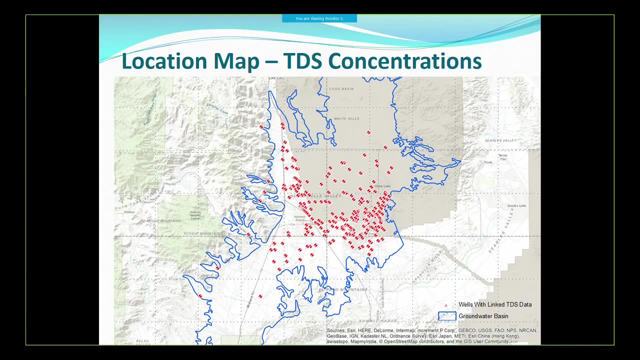 which we just haven't had time to go through that, but we just got the database from the water district and decided to pull that together for this meeting Onward. here's a location map showing the distribution of the unique TDS well locations that we have. You can see a lot of them. a lot of the data is over in. 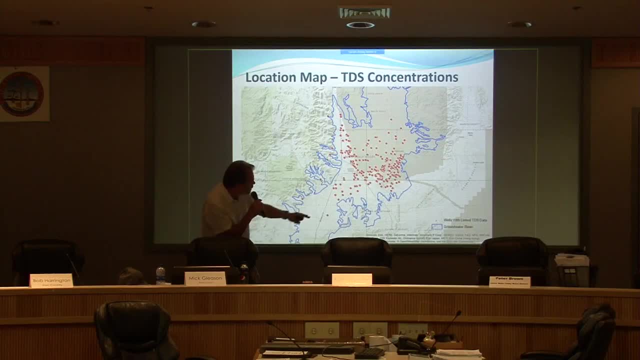 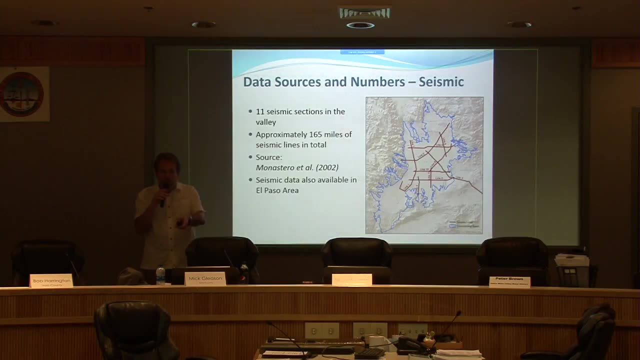 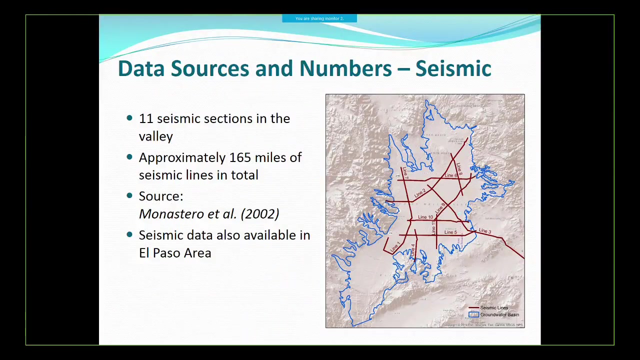 this part of the basin, This is the whole Indian Wells Valley basin here. We don't have a lot down here and you'll see the importance of that as we move forward. The other thing is seismic data and we have 11 seismic sections that were. these were seismic. 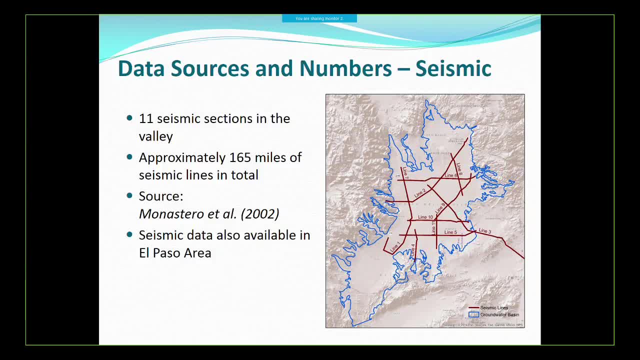 lines generated by the Navy geothermal office and approximately 165 miles of seismic lines again concentrated in that portion of the basin. Of course geothermal office, of course it kind of gives a hint of kind of what they were looking for. They weren't focused on the shallow. 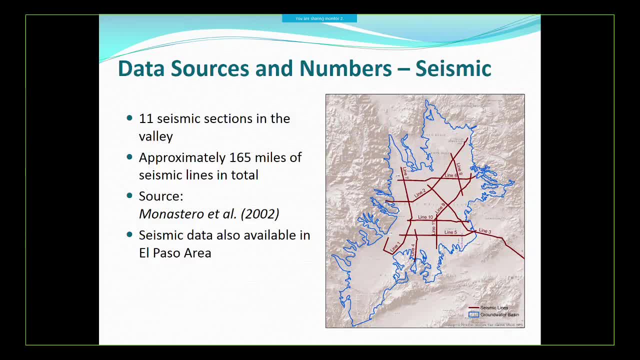 materials, so much, but some of the seismic lines have been reprocessed to look at that and they're reported. some of that's reported in a document referred to as Monastero 2002, which is listed And we're going to have a Q&A. 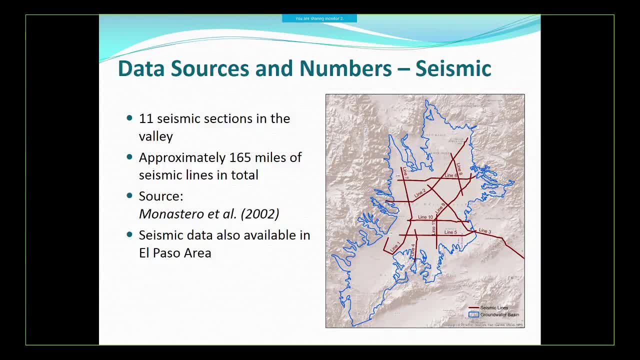 in a few slides, Oh, I'm sorry. So seismic line is basically: when you do a seismic survey, you send some sort of a pulse of energy into the subsurface. that can be with explosives, it can be with trucks with plates on them. They call them dino-size or vibro-size that. 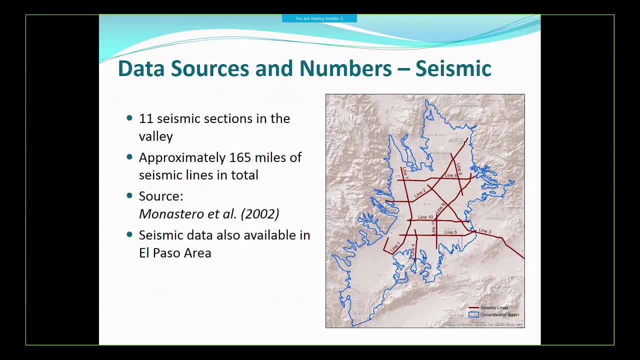 vibrate And with these big trucks you can vibrate at a particular frequency, adjust the depth of penetration, And then you have what we call geophones at the surface and measure how long it takes to come back up. You can see contrasts in materials with that as things. 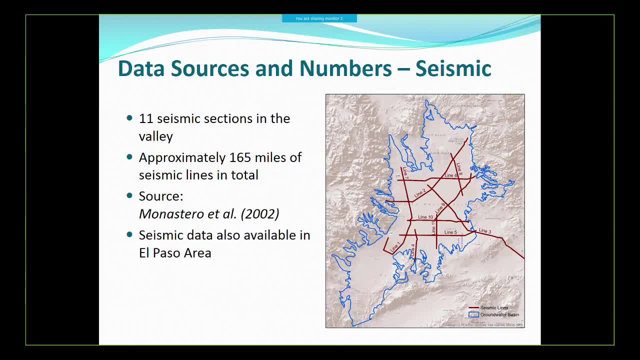 are refracted or reflected. So it's a way to look at the subsurface remotely with a force of energy. and, yeah, these are the lines along which, with these things, these seismic surveys were done And you can see that we also have. I should back up just a minute. 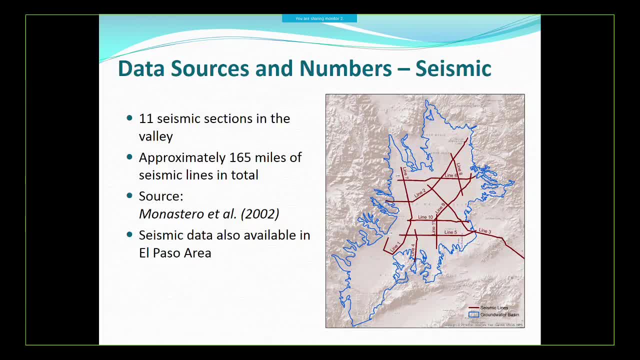 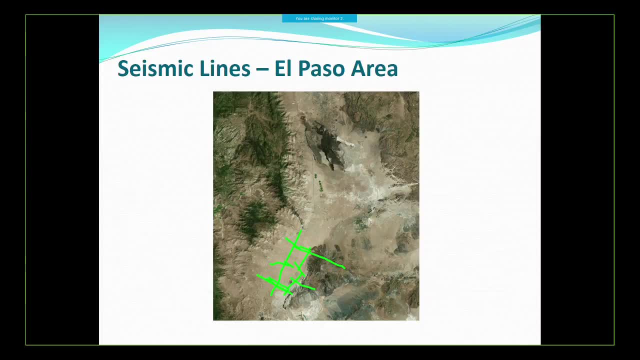 So these lines, we have the data for the process data and we have the output and you'll see some of this In the El Paso area, the southern part of the basin. sorry that there isn't a groundwater basin outline, but this is the outline of the basin again. 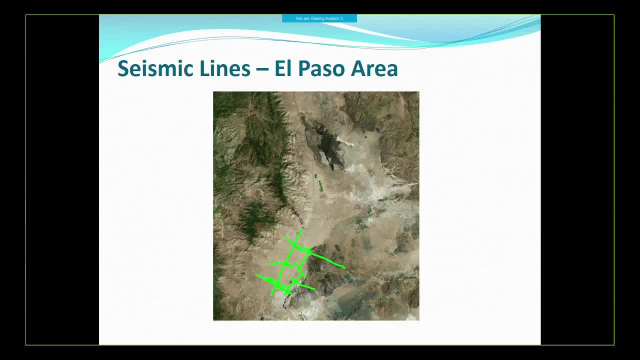 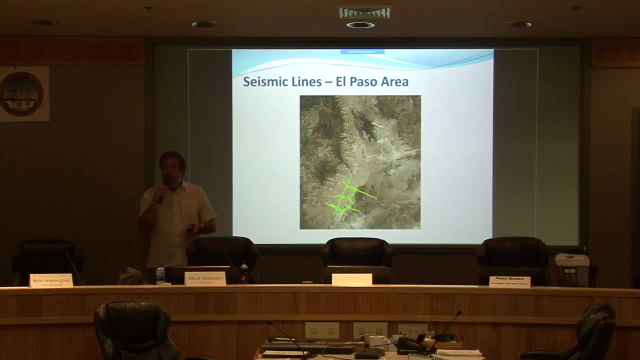 These are lines that we found that are available. They were done by oil and gas, So again it's going to be focused on the deep, but sometimes these can be reprocessed. But so there is some additional data in the El Paso area, the southern part of the Indian Wells Valley. 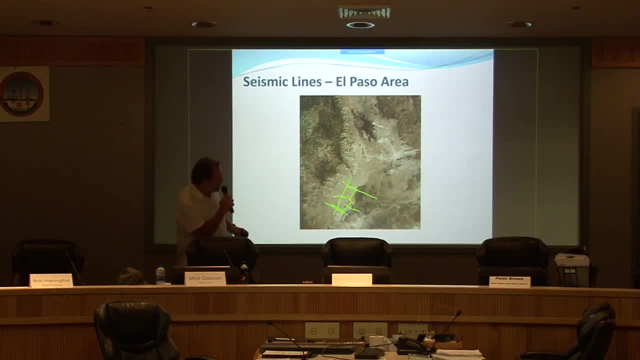 Basin. Yeah, it's over here. I'm sorry, Right, So this is the southern part of here's Red Rock State Park and you're driving up 14 here. Where did the Garlock fall? It's down here. Yeah, it's down here. 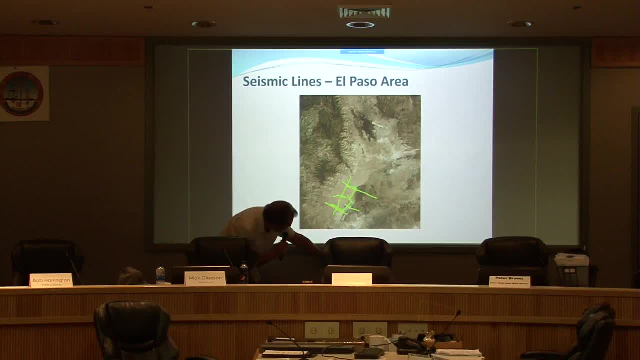 The basin kind of comes here and yeah, Garlock's probably down about here, Right, right, Actually, it's right here, Right there. Okay, I don't see very well, so sorry, Yeah, Any other questions on that one? Okay, So here's just one of the outputs. 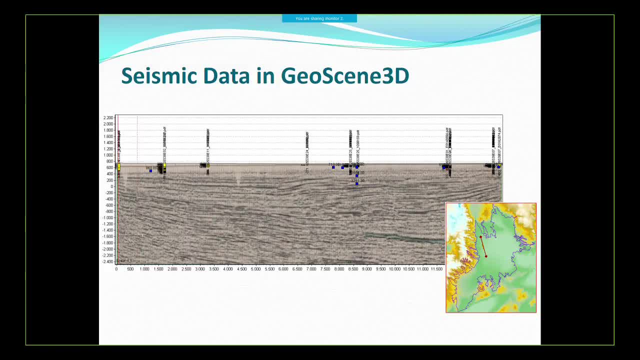 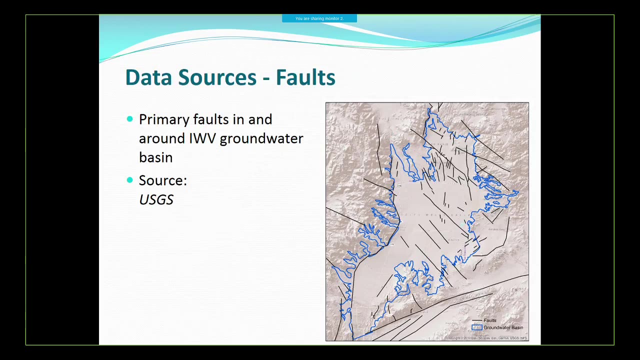 from it and you can see some layering here, the lines. You can see how it's got some sort of basin structure here, And so this just is an example output and where it's located is right here, And so another source of information we have is faults from the USGS. 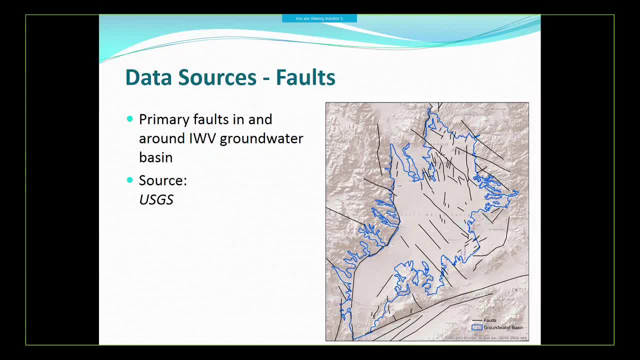 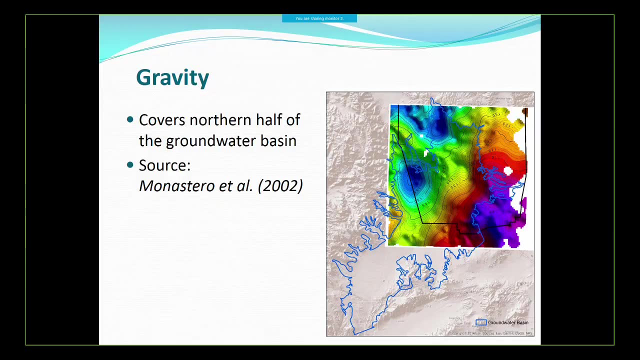 So these are some of the mapped faults. California Geological Survey's also mapped faults. So these are some of the data sources we'll be using in the hydrogeologic conceptual model, or HCM. And then a gravity survey was also done by the Navy in basically the northern half of 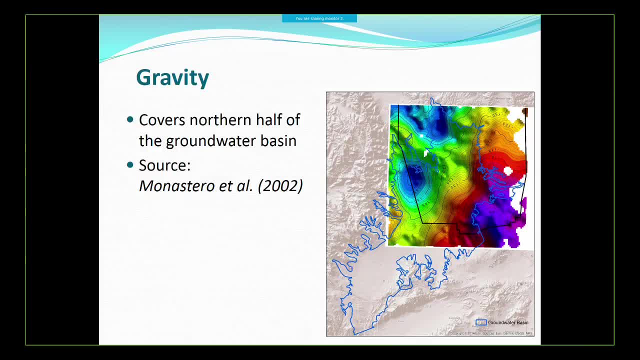 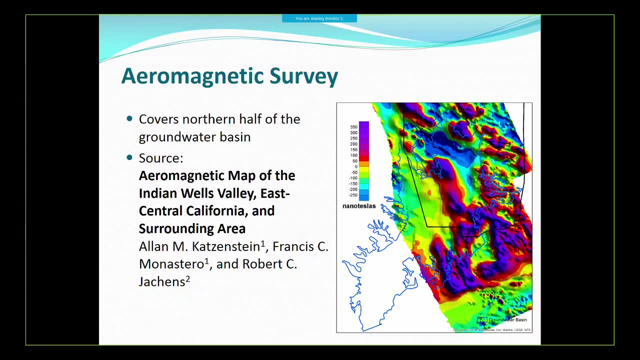 the groundwater basin, And again this is summarized in Monastero et al 2002.. And then there was also a magnetic survey done by AIR, And this is another survey that was done by the Navy, And Monastero was involved. 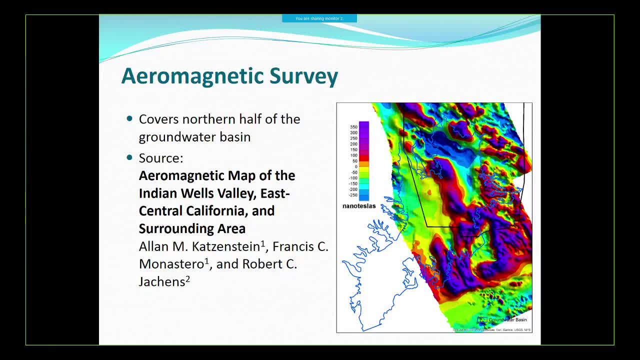 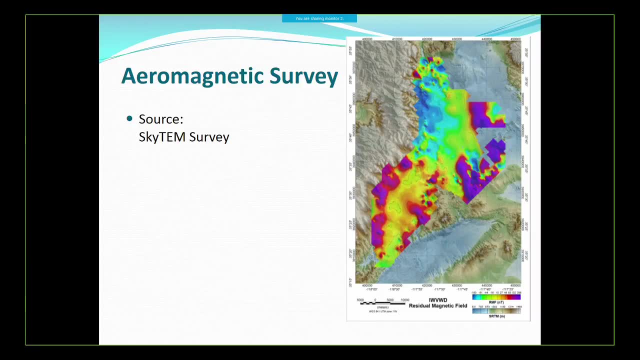 with that one as well. as you can see, I think there are some other folks that were at the geothermal program. I'm not going to get into their interpretation, I just want to make you aware of the data that's available. And then when the SkyTem survey was run, they also ran magnetics, so aeromagnetics And 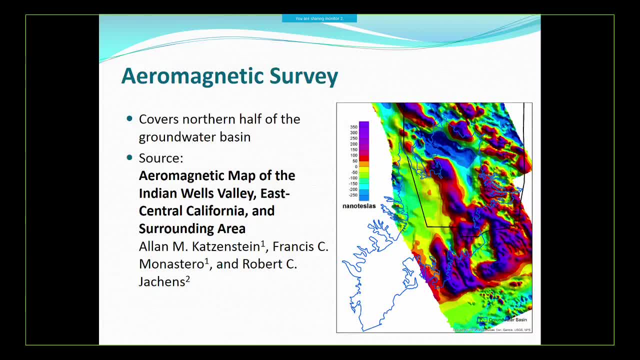 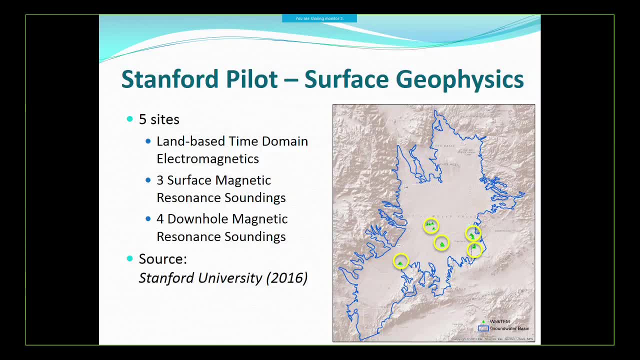 just to show you, they're pretty similar in terms of looking at the output, And Max is going to talk a little bit more in detail about that- And then surface geophysics. Now, when Stanford, a guy by the name of Jesse Cruz and I talked 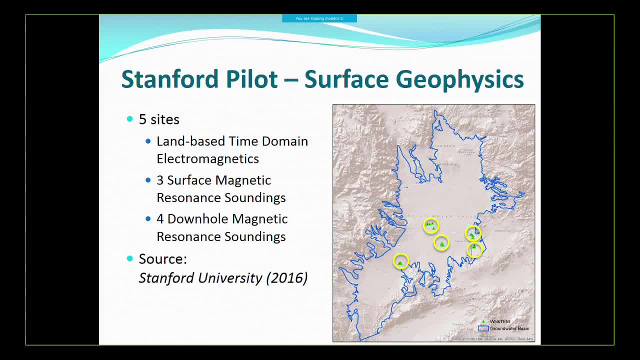 a number of years ago. he's a research geophysicist with Stanford, or was, And he talked about coming down and doing a pilot And I said: sounds great, how much will it cost? well, he said that they would do it, so they. 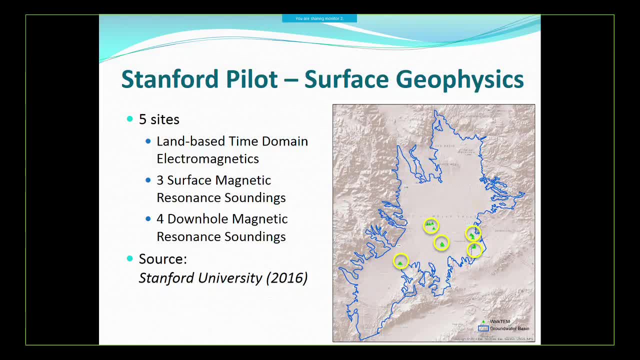 came down and they, they did basically time domain electromagnetics, which is in principle the same thing that sky Tim runs on in terms of the basically methodology of the approach. and then they also did surface magnetic resonance soundings at three places, and then they found that didn't work so well. they came. 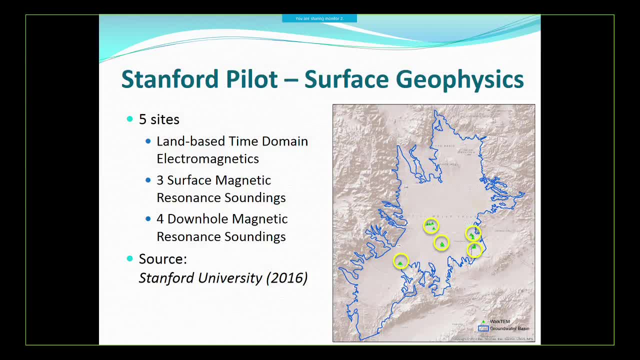 to the district and said: hey, we'd like to do some more. we've run out of funding in the district- funded them to come down and do another pilot with Koso- I'm sorry, Chris. thank you very much with Koso- and and they did the second time around. they. 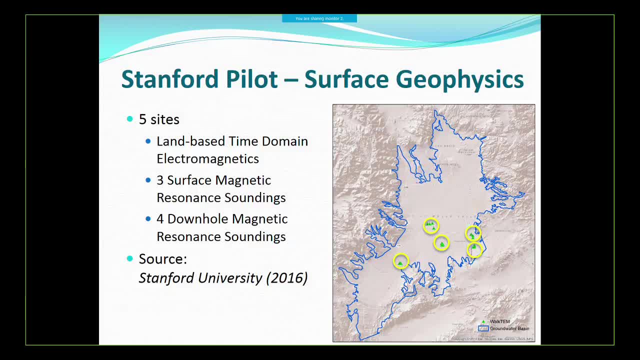 they used downhole magnetic resonance in some plastic wells and basically they said: hey, this, this is great, this stuff works here paired, and that's what we were looking for. and they said: hey, this is great, this stuff works here paired, and that's what we were looking for. 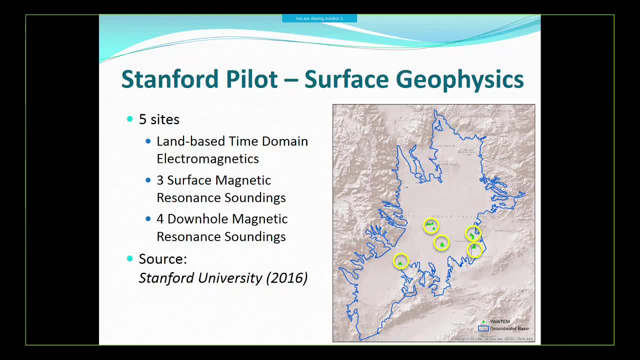 for. but you know this is really an ideal place to do aerial electromagnetics for. but you know this is really an ideal place to do aerial electromagnetics because there's a lot of open space and it looks like it would work very well. so that was a recommendation that came out of their report, and then that's really. 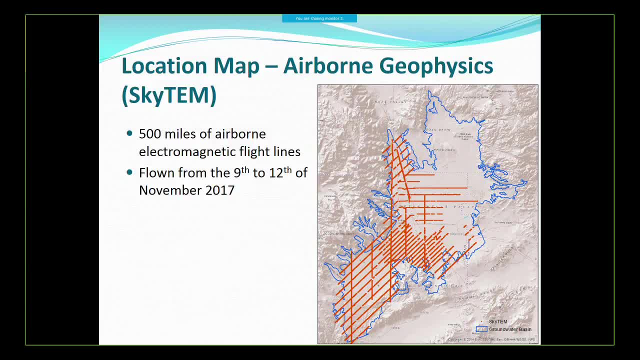 how this all came about. we started talking about it. I actually met some people from Denmark. while we were in the midst of discussing it got one of their salespeople on the phone and we had several conversations over several months and finally came up with some suggestions and we met Chris Goldstein, who's a 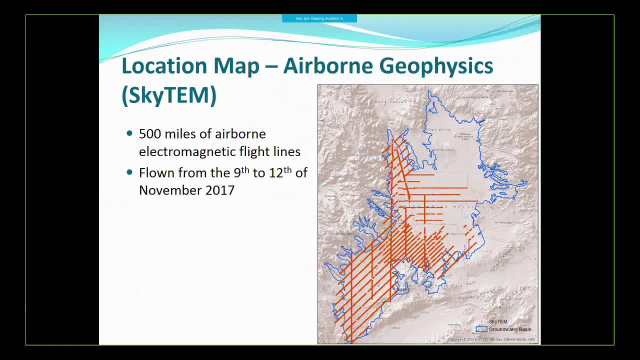 with the idea of flying it And I'm almost done. So this shows the 500 miles of airborne electromagnetic flight lines that were flown in the basin. You can see that there's sort of a gap over here and the Navy couldn't allow us to go over there. 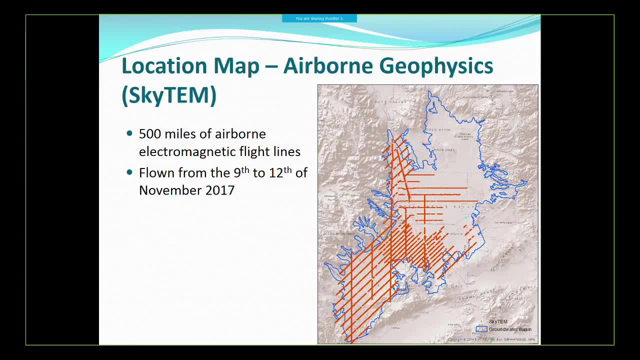 so we were fine with that. We got some pretty good dense lines. You'll also see that we concentrated a lot on this because at the time DRI had talked to us about the model and they said that they were having some trouble calibrating the model. 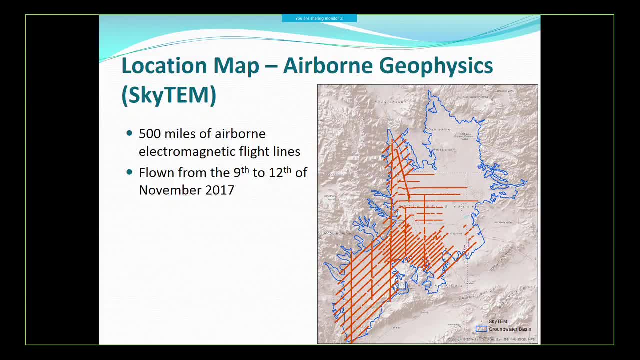 because of whatever this structure here is in the middle of the basin, which had been thought to be either finer-grained, some kind of a stratigraphic change, or else false. And so I'll turn it over to Max now, and he's going to talk to you about the SkyTEM survey and some other things. 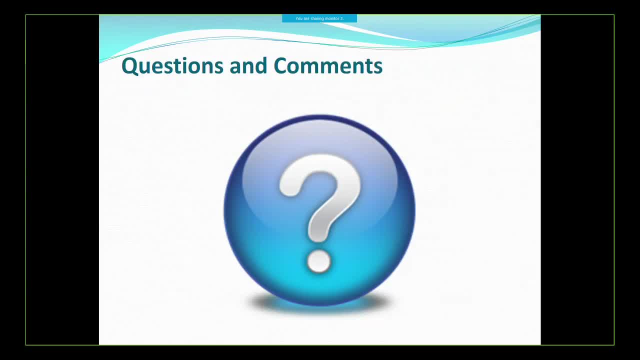 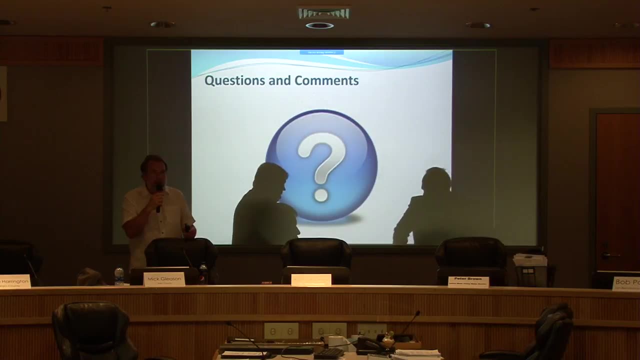 So, Max, Oh, actually, come on up, But we'll take a quick pause and see if anybody has questions or comments, because it's a good point as we turn from me to Max. Okay, perfect, Then let's just keep on trucking. 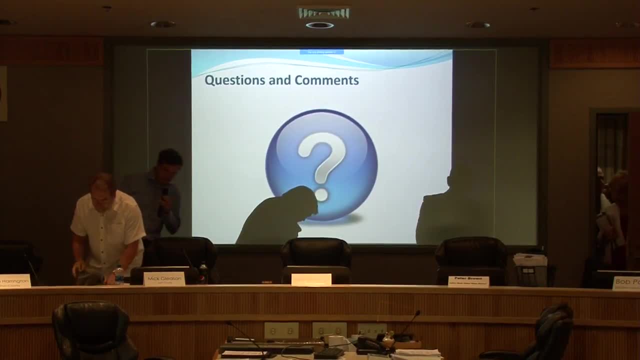 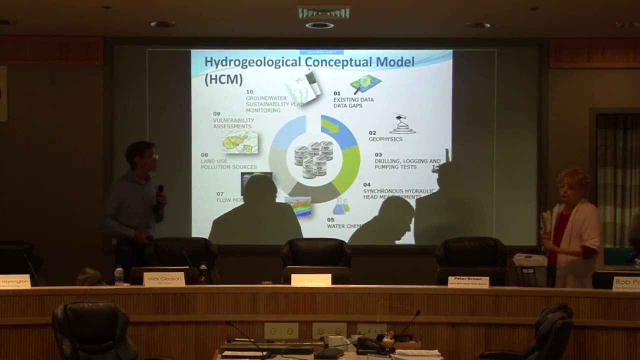 Thank you. Thank you, Yeah, Hello, I'm Max Helkian. We don't have a forum closed, so we're going to adjourn the meeting and we will put the tax on the tax that I would like to talk to. 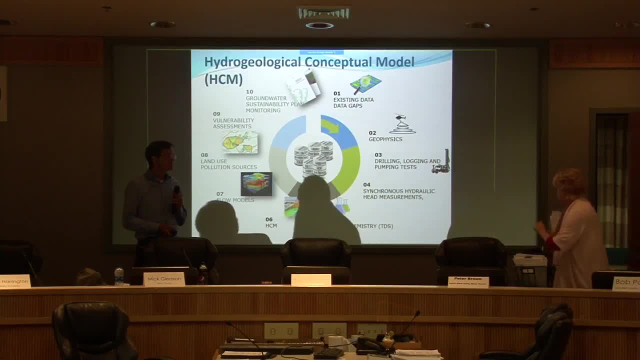 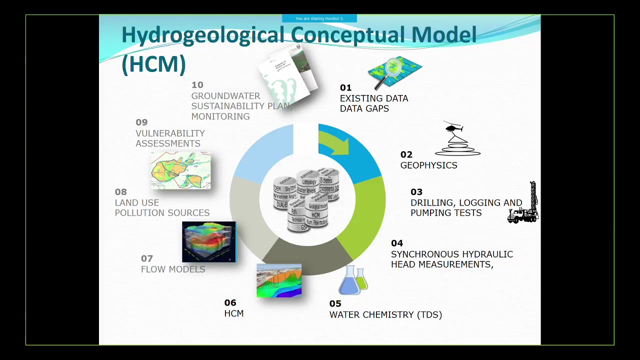 and ask the tax people to vote after this is over. So, thank you, No worries. Okay, I'll start out talking about what is the different tasks that we have been through here, or going through here right now when it comes to the hydrogeological conceptual model. 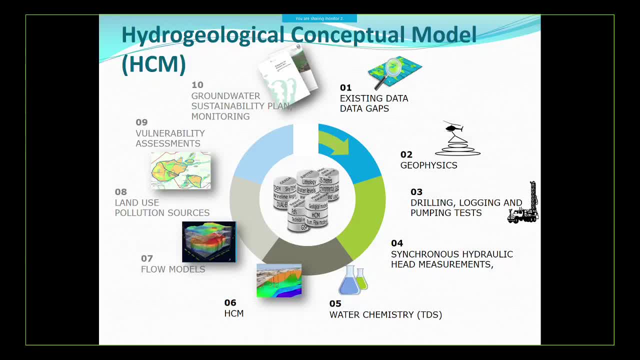 And it's basically as you said, Tim, it's about getting a hold of all the existing data, identifying the data gaps and then, based on those data, we decided where we want to do this airborne geophysical survey with the helicopter. 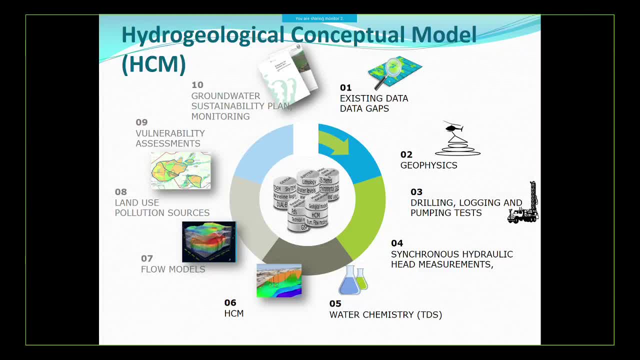 We have taken a look at all the drillers' completion reports. We have looked at the water tables, We have taken the water chemistry data, and where we will end up is here with- oh sorry, it's down here- where we have a conceptual model. 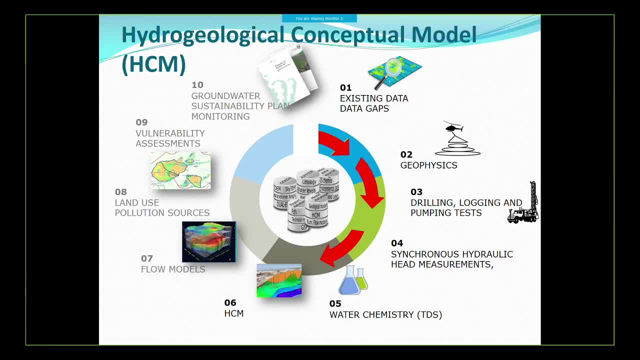 So that's how far we will reach with this exercise, with the project. So we'll deliver a 3D description of the different layers, the aquitains and the aquifers, where we have clay and where we have sand, which is very important for the flow. 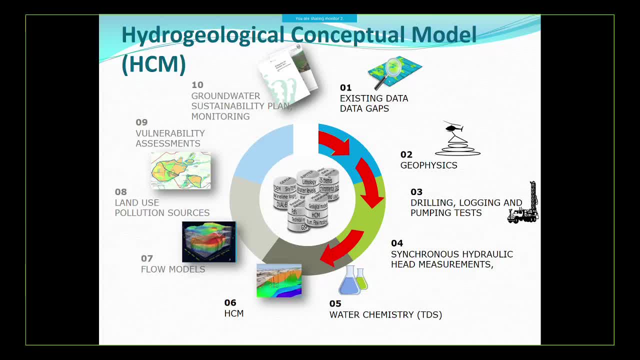 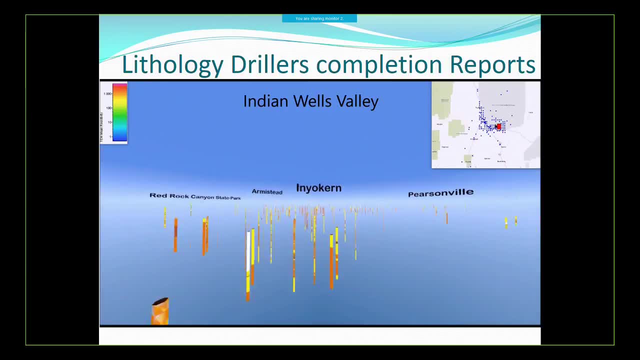 the water flow and our groundwater resource. So the very first animation here is just to show you. it's a. the camera goes from east- you can see it up there- towards west and all those different cylinders there, they represent wells that we have collected here. 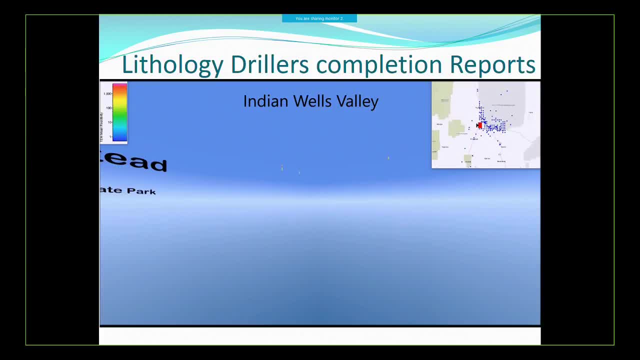 from the Department for Water Resources And, as I said before, there are 1,107 wells. Most of them are located here in the central part, around the cities, around Ridgecrest and around Inukern And when you get further south. 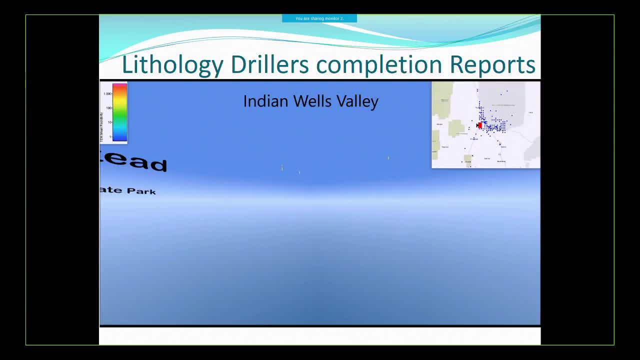 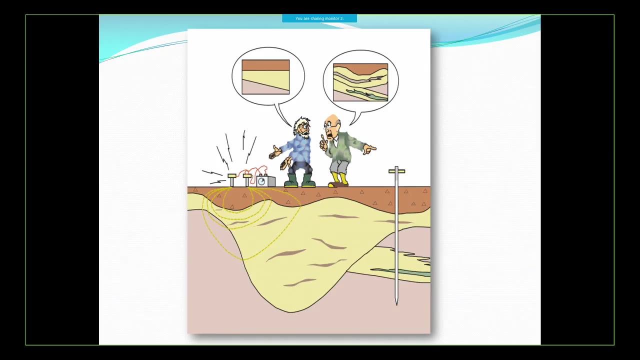 it's very sparse. We have very limited information. Also, what we have observed is that the quality of those wells- some of them- are very well-described because of the geology in the wells. Others are more poor in their descriptions. I also want to give you just some ideas on 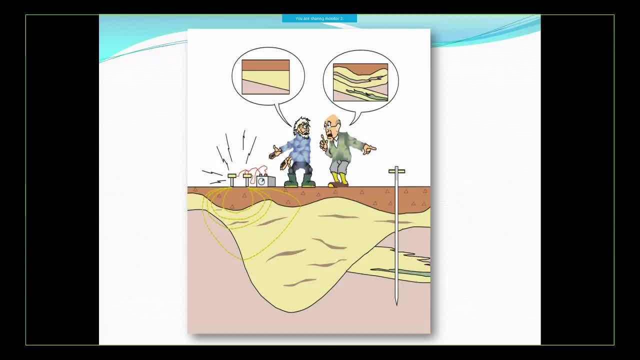 to the right. here we have the geologist. He will typically look at the geology from a well perspective, where we have very thin layers and a very detailed description of the geology. He knows exactly. here we have got one feet of layer. 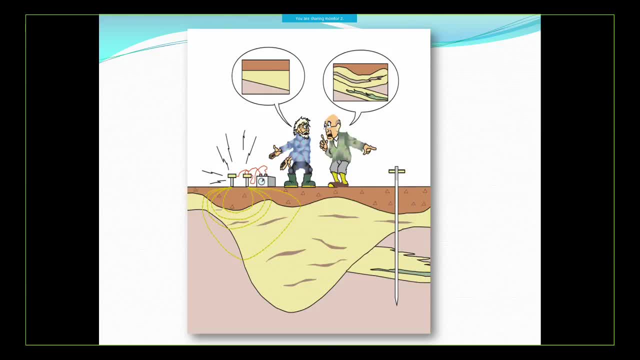 and another two feet above that compared to the geophysicist. He's looking at a more general perspective. He's looking at the layering. It could be that he imagined we have three layers or we have five layers, So we get an overall distribution. 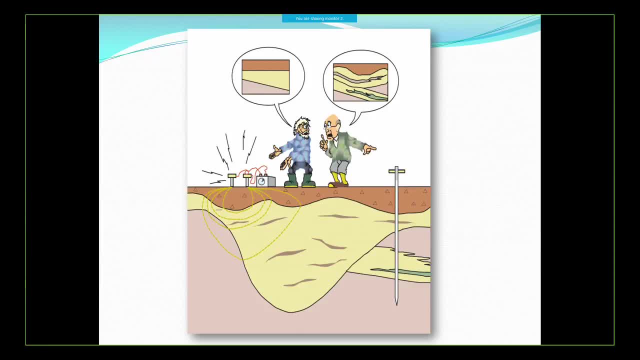 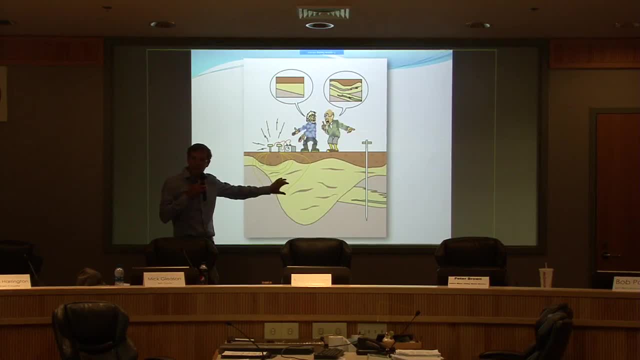 of where we have sand and where we have clay. So we get an average interval of the clay signal, the thickness and average thickness of the aquifers. So you should keep that in mind when you look at the data afterwards. It's a general description. 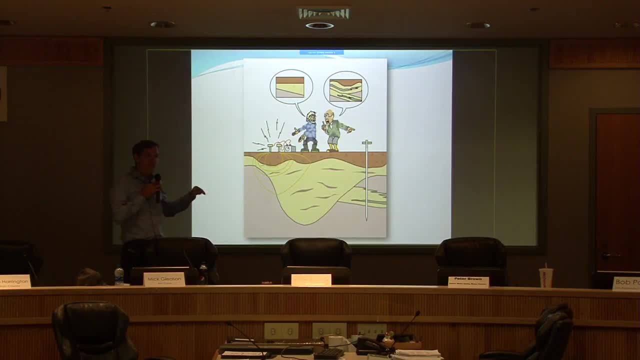 where it's most likely to have the thickest layers of clay and the thickest layers of sand. It's not an exact number And when we do collect all those physical data, we always go back and confirm our data. We tie them up to our wells. 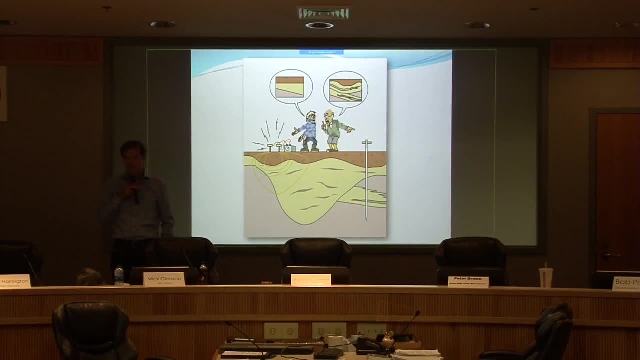 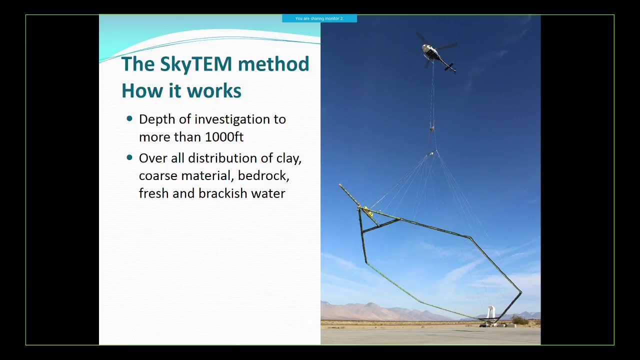 and compare with our wells to understand what we are looking at. So back in November we were flying this huge thing hanging below the helicopter. Some of you might have seen it- I'll show you a video very soon- And it's what you compare to: an MR scanner. 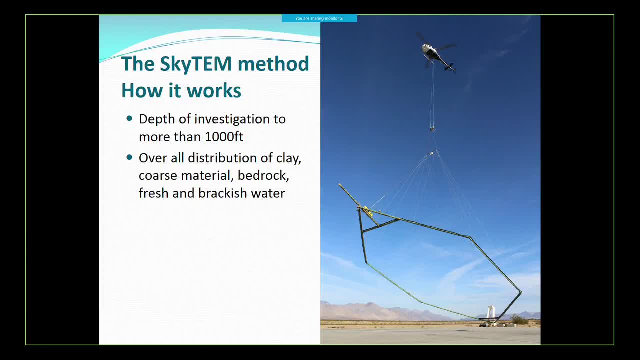 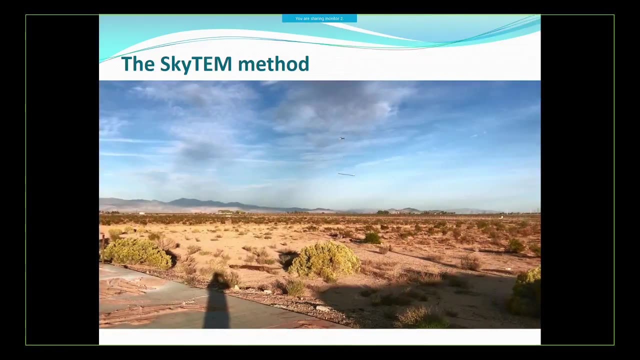 from the hospital. It's a scanner where you're introducing an electromagnetic signal and you get the response from the subsurface. that gives you an understanding of the geology, how the geology down to 1,000 feet. This is actually from the landing site. 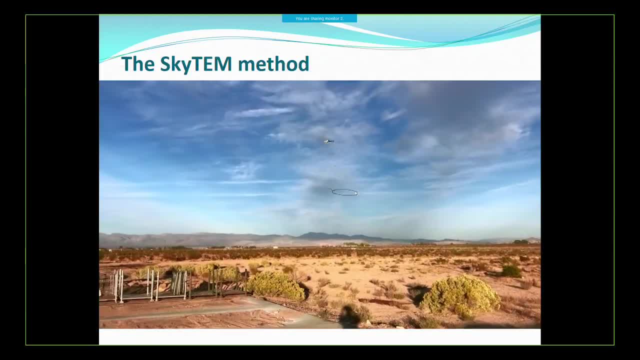 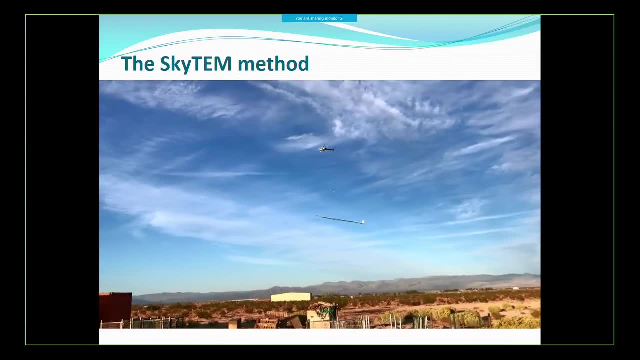 we had out in Inukern at the airport. there They were so kind to let us land and take off from the airport there, And here the helicopter is returning after being flying for two or up to three hours. So they have collected a lot of data. 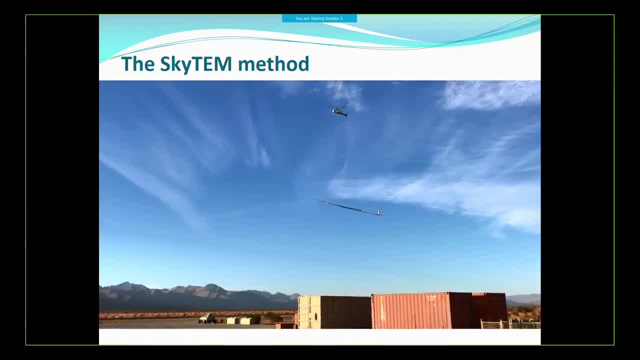 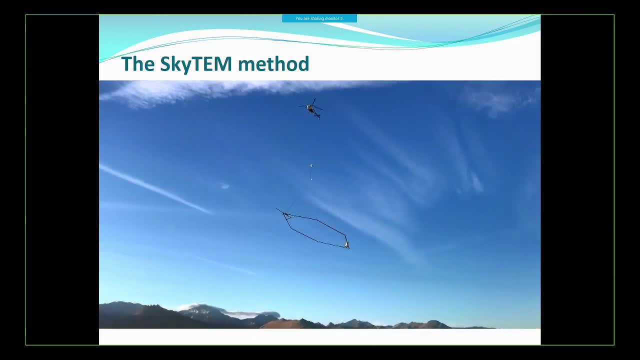 and then returned to base. They deliver the data to us as geophysicists and they refuel and maintain the helicopter And then they come back And then they're ready to take another flight, As the helicopter is flying at a speed. 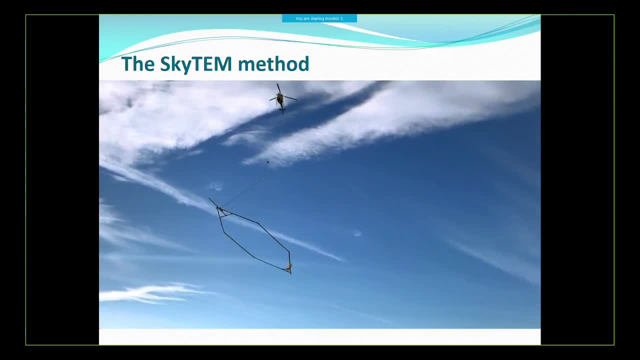 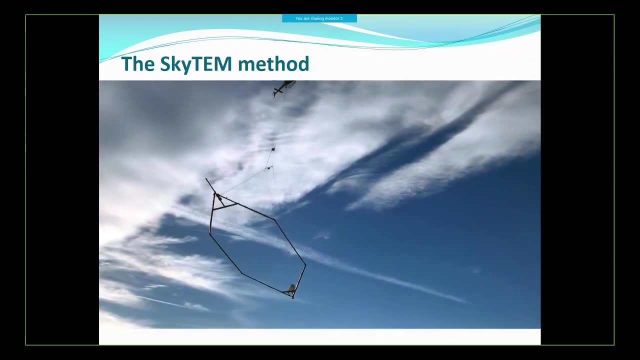 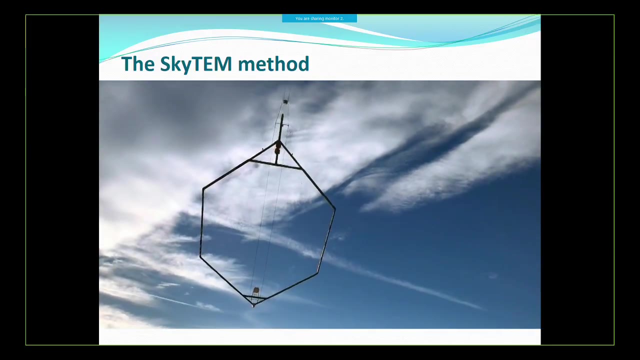 at maybe 50 miles an hour, they can collect a lot of lines per flight. So this is just to give you an impression. We covered the whole basin in only- I think it was two or three days. Basically, there should be a sound here. 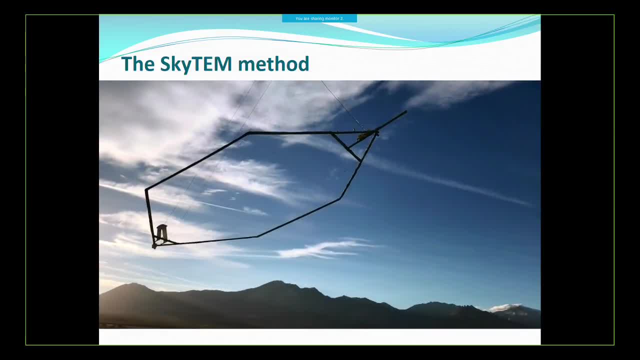 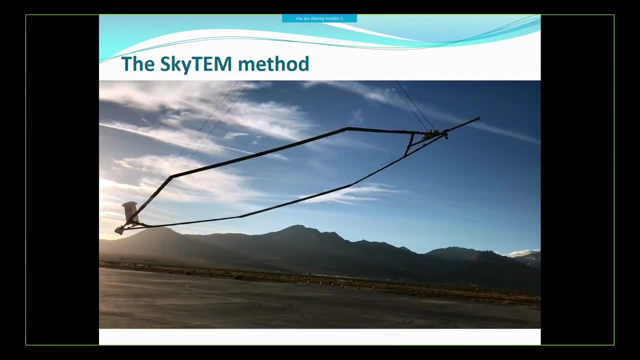 But it is a little bit noisy when you're just below the helicopter, But while it's flying you hardly notice it. If you are having cattle out there, they might get scared just for one second and then they just shake their heads. 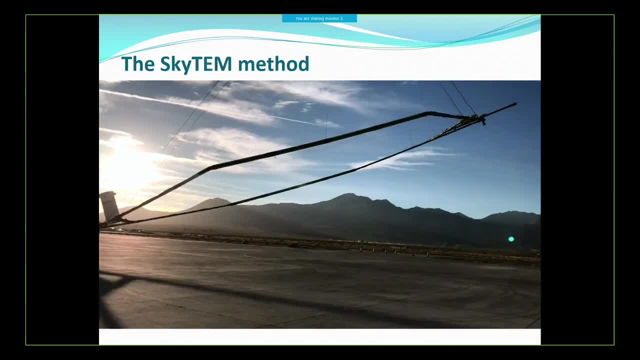 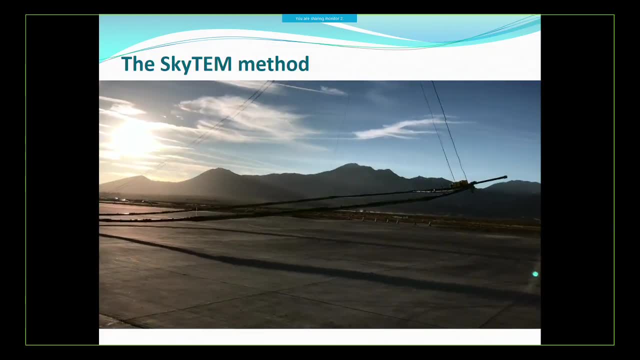 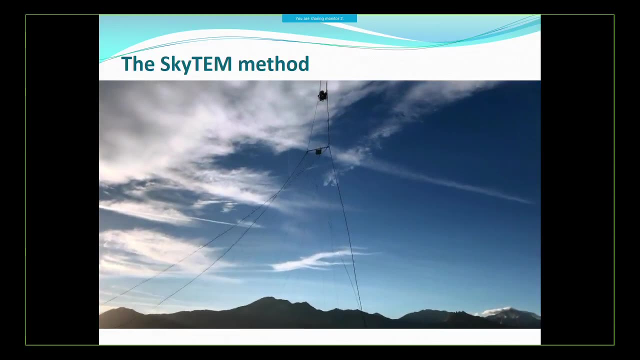 and then they'll move on, And it might be the same when it comes to people. So here we land and the helicopter pilot gets out and he's pretty exhausted because he has to take care of all the different obstacles that he will pass during this flight. 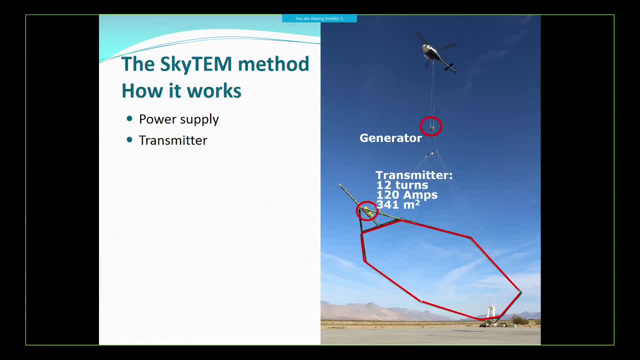 Okay, I'll move on. So what does the system consist of? Up here in the upper part, we have a generator and down below we have a transmitter. So we transmit a lot of current in a very large loop, And it is the size of this loop. 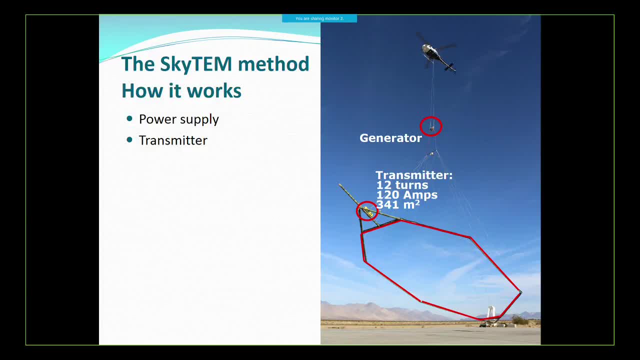 and the amount of current that we induce there or transmit. that creates the strength of the signal and how deep we can penetrate, And basically a conservative number is 1,000 feet here. We might look a little bit further in some places. 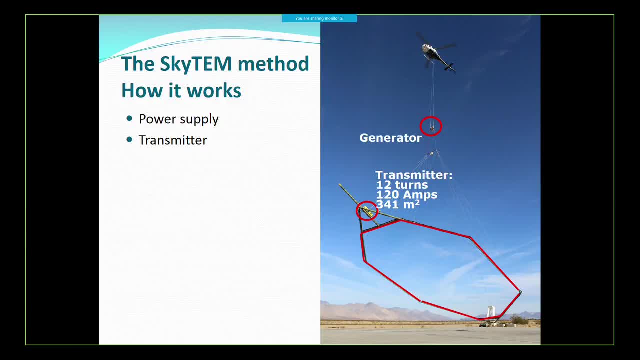 and where we have the China Lake, our depth of investigation will be slightly less. So it's geology-dependent And, as said before, up here in the front we have a magnetometer and the primary data is the electromagnetic data and then we use a differential GPS. 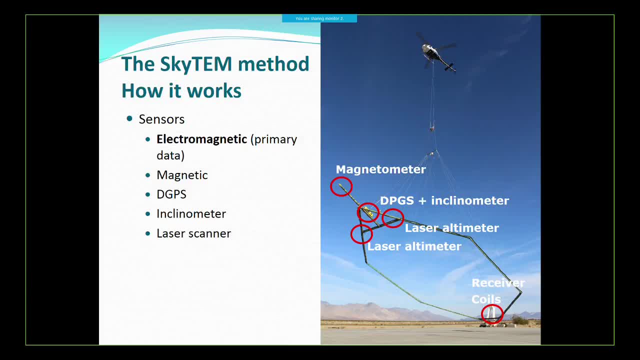 and lasers to measure the height of things, So we have everything under control. It's not like your wells, where we don't know where they are. We know where our data are, within centimeters an inch or better, So it's very well positioned. 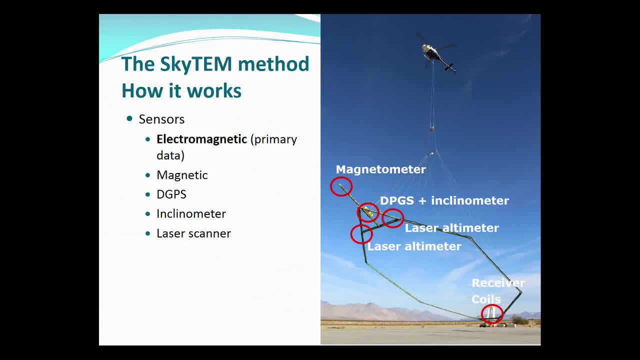 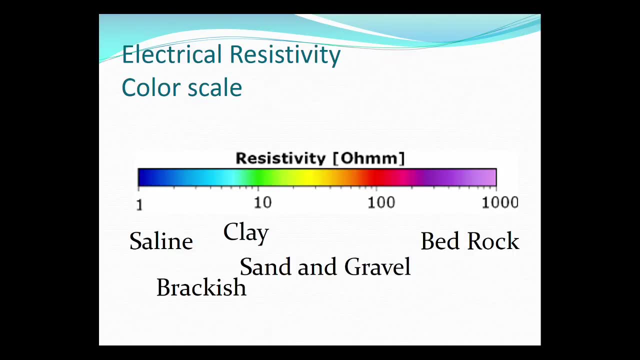 Now I'm facing the same problem. Okay, So what we measure here with the induction coil, the receivers, is the electrical resistivity. And now I'll try to teach you on how to read this electrical resistivity scale. here The colors means that's the resistivity. 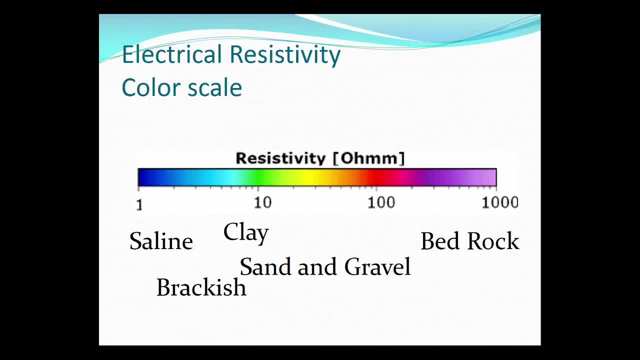 That's ohm meters. So when it's blue, it's saline water. When it turns more light blue, it could be brackish water, It can be turned into clay. When it turns green and yellow, it's sand and gravel. 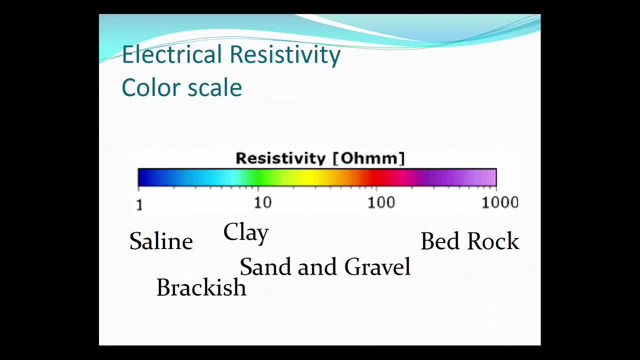 And further up here, when it gets very purple, then it's the bedrock that we see here. So that's the general relation in between our resistivities and our geology. So keep that in mind, because now I'm going to show you. 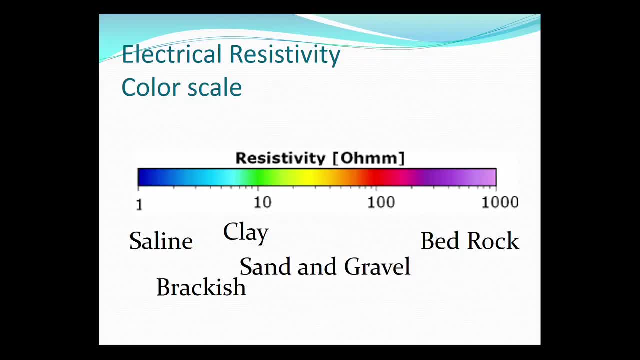 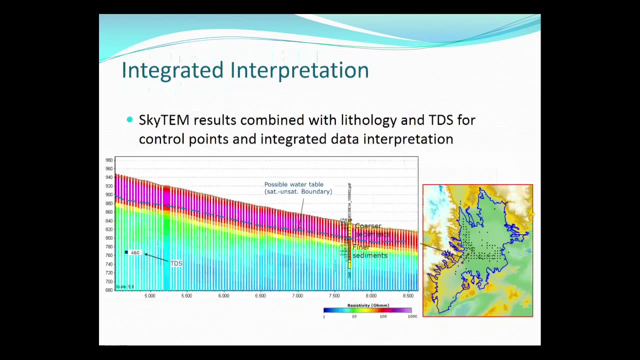 a few plots, illustrations, where I use this color scale. I might show it to you. Okay, I'm not in control here. It's good that I'm not flying a helicopter. This first example is just not an arbitrary, but it's just a short section. 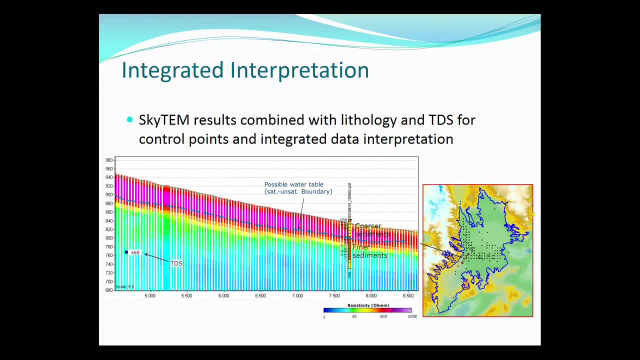 that we placed out here in the basin And here on the vertical scale. you can't read it from there. That goes from 900 meters above sea level to 700 meters above sea level. So it's a vertical section. So that's the line we have flown here. 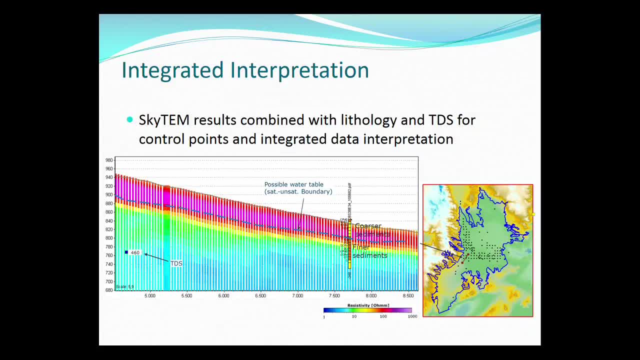 and that's the topography, That's the terrain that you see here, And down here we have a well, and it's described here with the yellow colors are sand and gravel, and then we have finer material down there And then out here we have a TDS value. 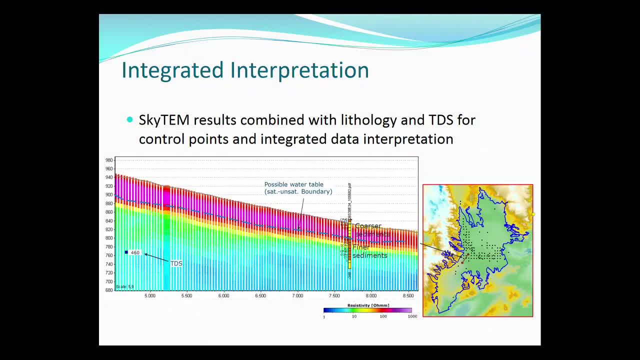 to compare with And we see some nice patterns and we are able to do what we call an integrated interpretation of the data. So we try to understand what does the resistivities reflect and how do they correlate with the geology and the TDS values? 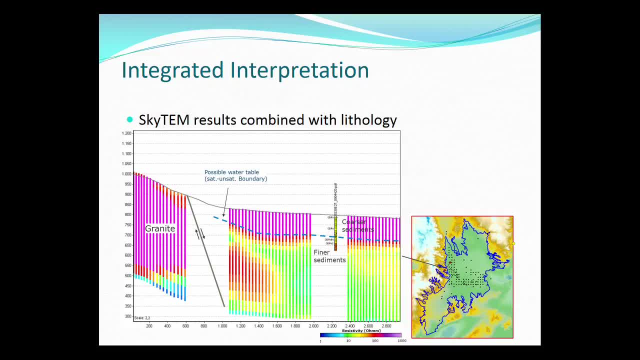 Another example here. this is actually again a vertical section. It's from a little further north, And here you see the granite here to the left, and this is actually the boundary of the basin. So with the data we can really precisely determine. 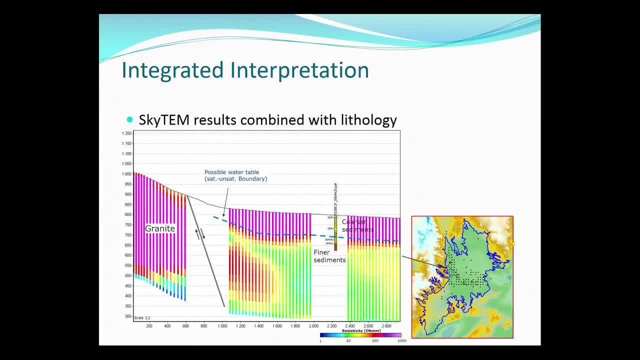 where do we have the boundary of the basin? We can also look at the material here just up in the upper part and find out where would it be feasible to infiltrate surface water, storm water, if you like It might be. in some places we have clay. 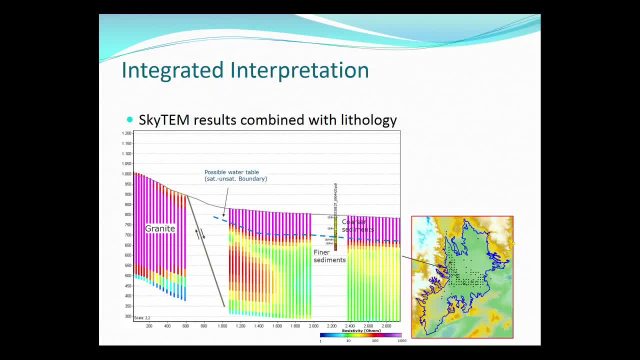 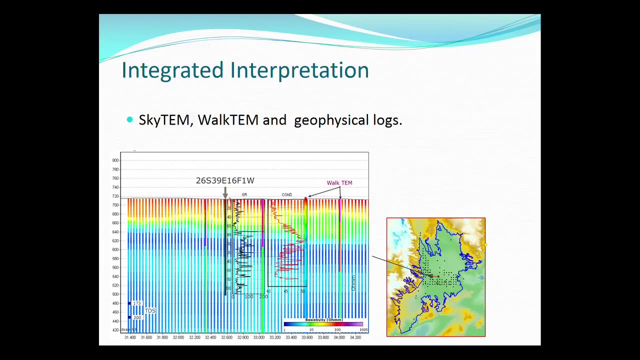 and in some places it's not as feasible to infiltrate storm water as it would if you had more coarse material. And again here we have correlated with where you have your faults, And that's very often related to the basin boundary. On this illustration here: 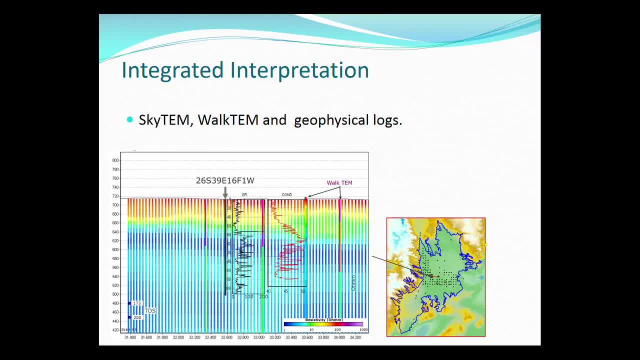 I compare the results with the geophysical logs. You mentioned that we have close to 100 geophysical logs And again the resistivities, conductivities. they should correlate very precisely with the SCITEM data And by having the geophysical logs. 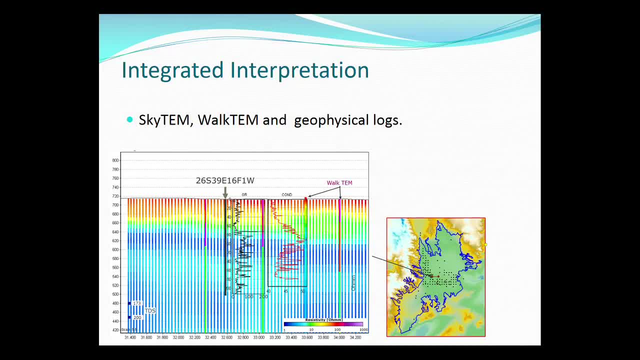 by having the lithology, the geology described in the letters, then we can create an atlas, a link in between resistivities and geology, which is very valuable when we in the future should further develop our understanding of our geology here. 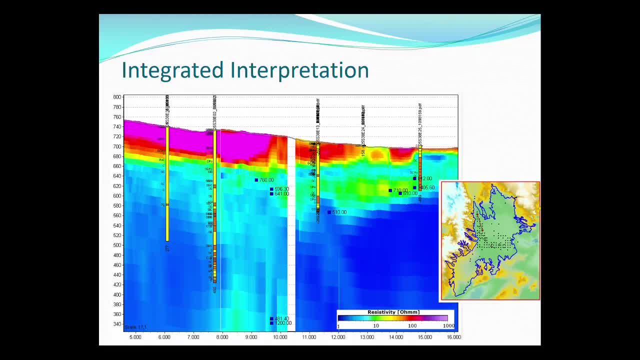 This example is picked just to show you that we in some places have a number of wells and they are pretty deep, So that gives a very good possibility to get an even deeper correlation in between the wells and the resistivities. Also, we see here that we have a number 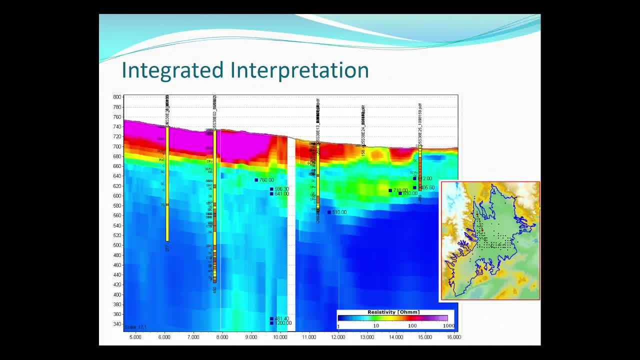 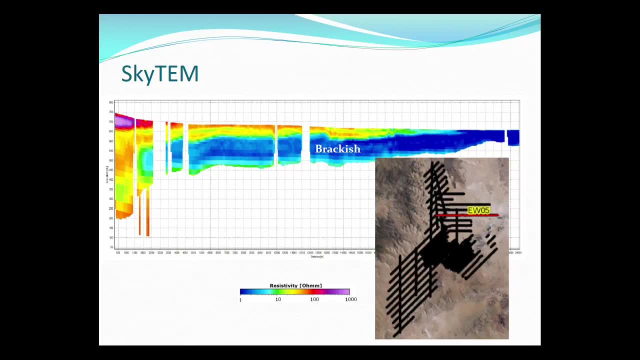 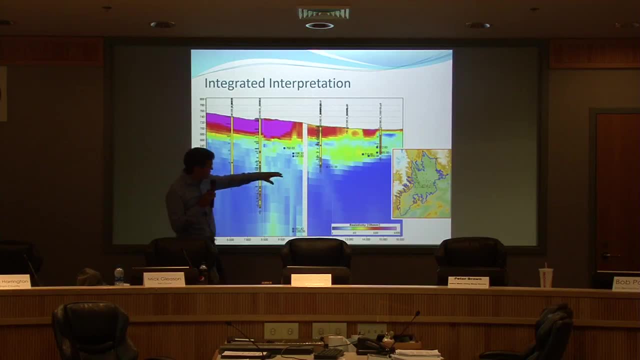 of locations where we have TDS values. This section, Yeah, it is. For the moment it is brackish water But honestly, here in the deeper part we might have to mask some of the data. So we are still finalizing. 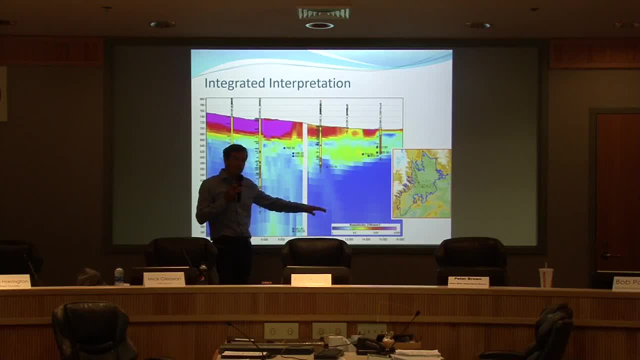 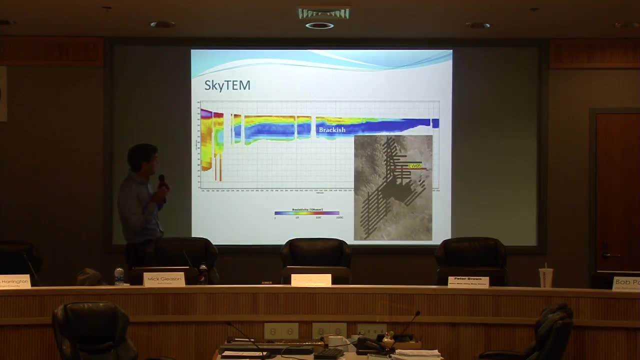 our interpretation of the data And it is likely that we have some which is not as saline in the deeper part of it. You can see here on the next slide we have actually masked some of the results. You can also see. it's a different. 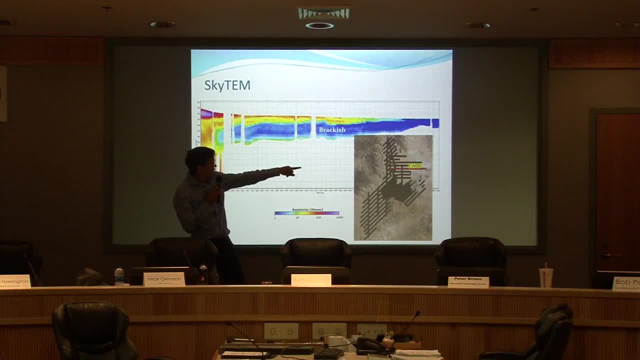 illustration. So we have masked some of the data And it starts out there in the China Lake, where you see we have salt all the way to the surface, as you would expect, And then you can see how the brackish water propagate to the west. 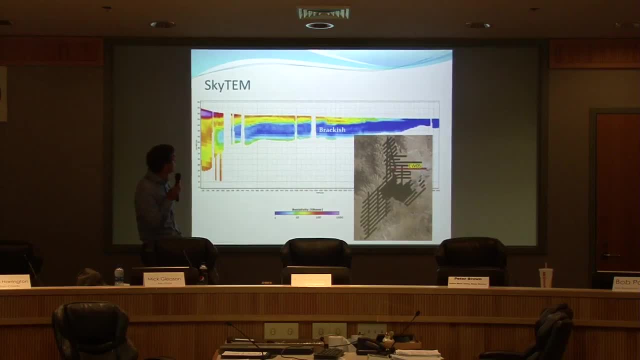 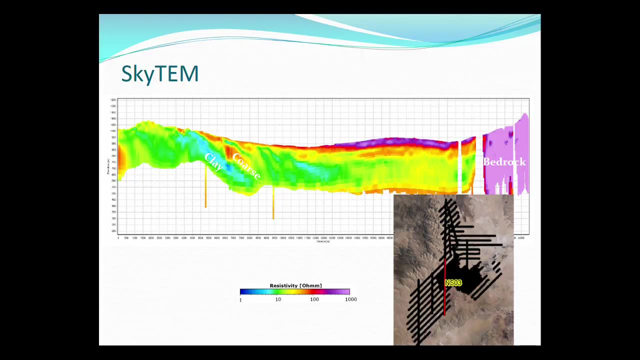 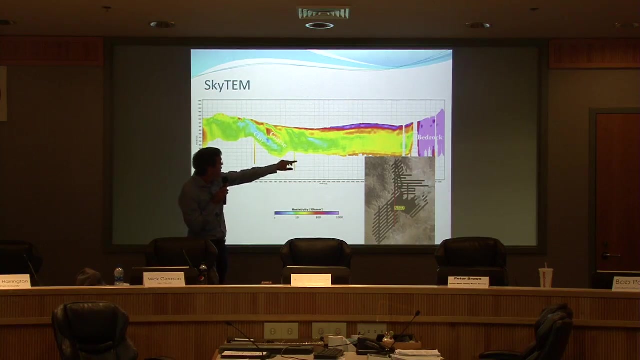 So I hope you can locate yourself there. This section is from the more southern part It's going from. This is to the south And this is to the north, So it ends up in the bedrock to the north And here you can see down south. 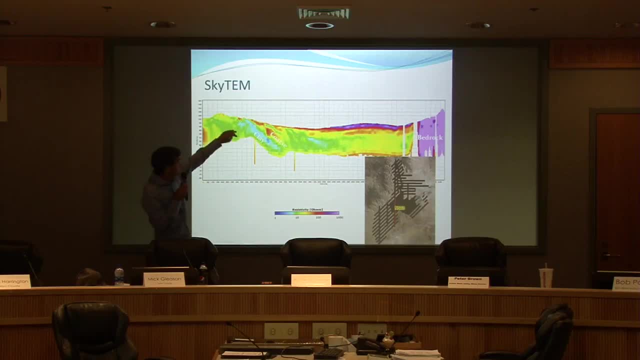 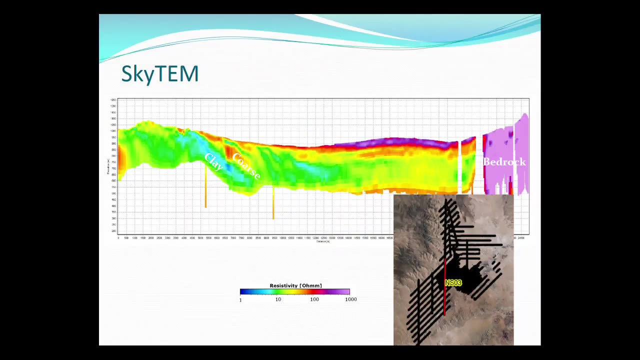 the geology gets very complicated. So we find here we have some dipping layers And in certain areas you might find that we have pockets with sand and gravel divided by clay. So I think one of the conclusions down here will be that we have some lines here. 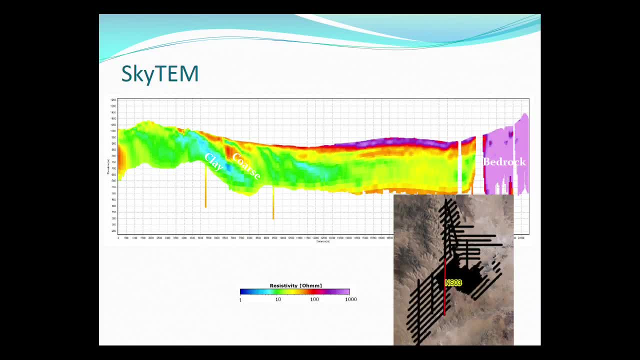 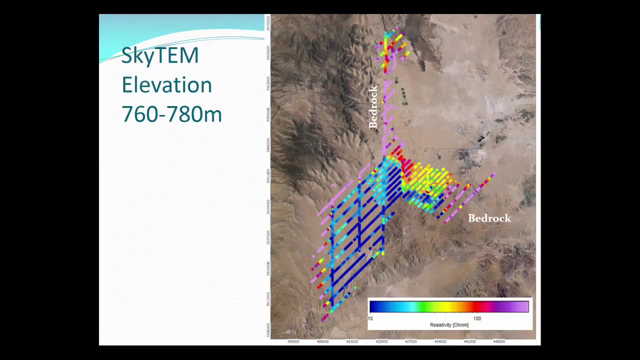 They are flown with two miles spacing, But the geology is complicated, So we get our first impression of the data And we have only a few boreholes to tie up with. This plot is seen as a horizontal view across the area, The reason why we do not have data out here. 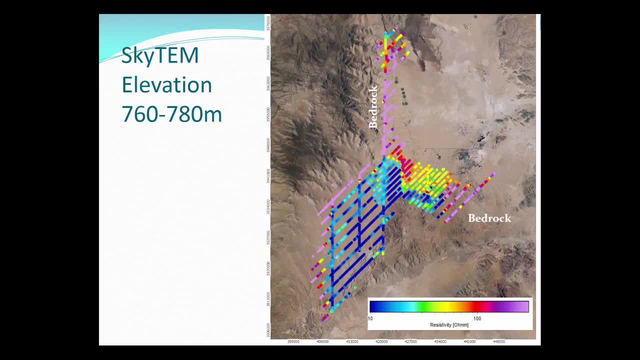 in this area up here is because it's a horizontal view meters above sea level. It goes from 760 to 780 meters above sea level. Out here the terrain is lower than that, So it's not presented here, But I'm showing that because I want to point out. 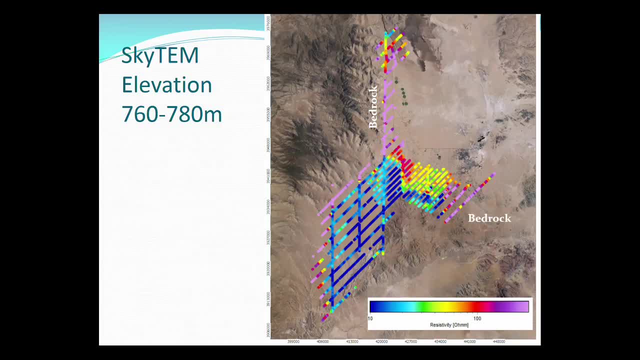 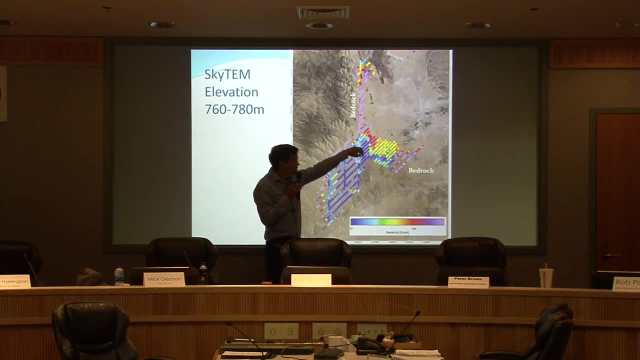 sharp boundaries like this- And this is exactly what you referred to before, Tim- where people are discussing how do we calibrate our numerical flow model, our groundwater model, in this area, And I hope that we will be able to give them a much more detailed and better understanding. 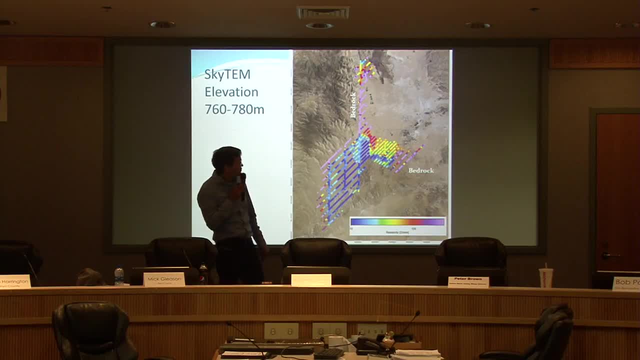 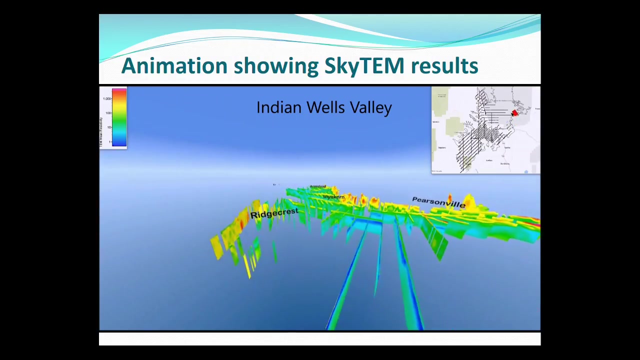 of where do we have clay and where do we have the more coarse material in an area like that. Out here we also see we have the bedrock here, maybe forming the boundary of the basin here in that depth. The final animation here is actually a way to show. 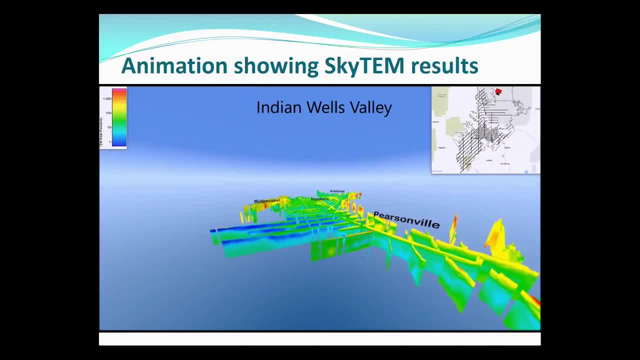 and illustrate all the SkyTem data. You can see it's a camera up there turning around. So now it's looking from the north here to the south. Here you have the China Lake. Now you follow it here along the mountains looking into that. 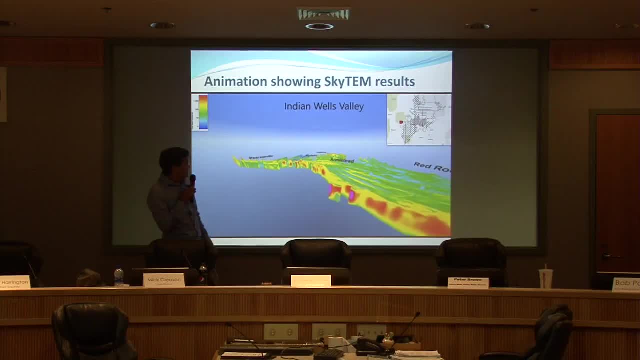 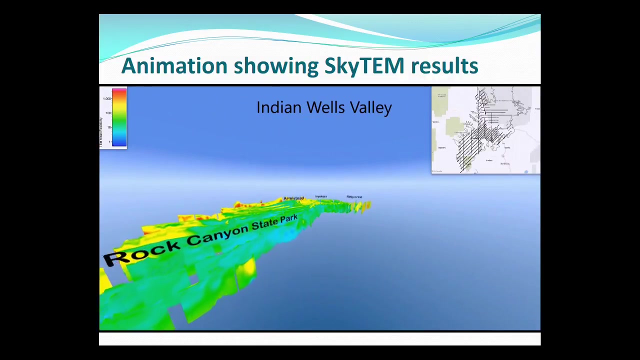 Ridgecrest is there in your kernels up there, So it's a way to compile and visualize all the data. So right now we are trying to get hold of as many data as possible and then develop our final understanding of the distribution of sand and clay. 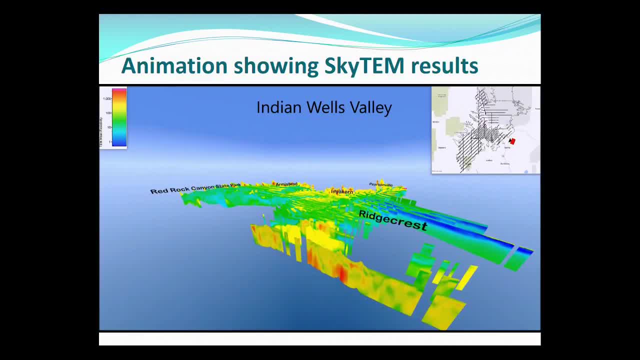 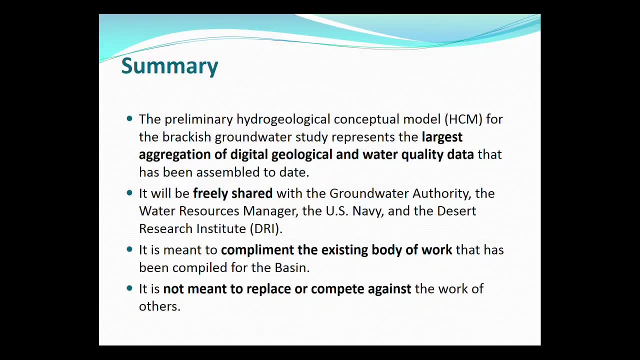 and other coarse materials across the basin. I think that's the last one I had here. Then I'll give it to Arda, Are you done? Thank you, Yeah, We might have some overlap When we're talking clay. 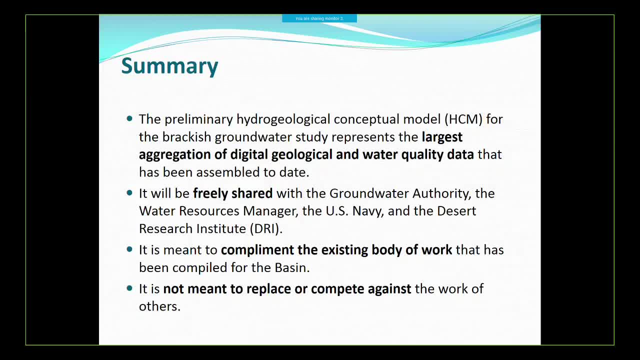 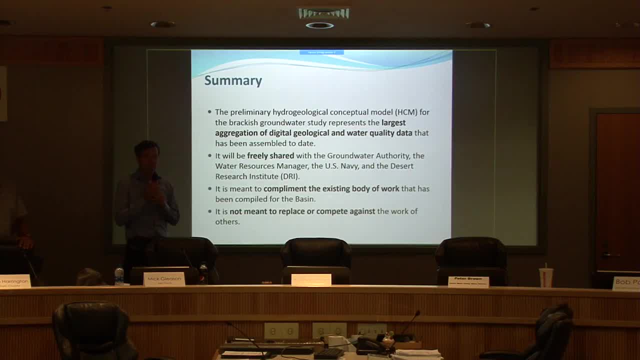 you might have wr し water as well, have a higher resistivity, So it will show up as more hot colors, the red, and maybe even towards purple, on the plots. You never seem to make that distinction. 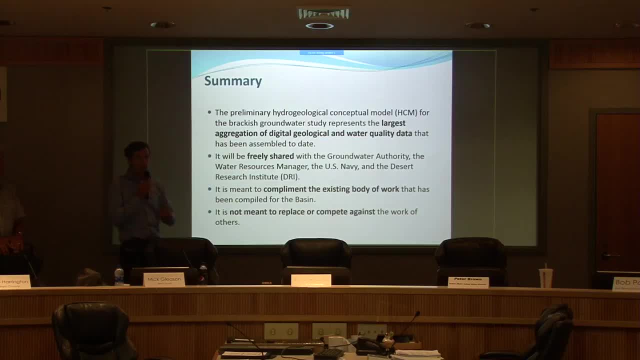 I was just wondering whether I'm making that point. Yeah, but it's a good point. We will also bring in the water table, the contoured water table, and then we can compare with that and see where we have that boundary. So it is possible that we'll be able to determine the water. 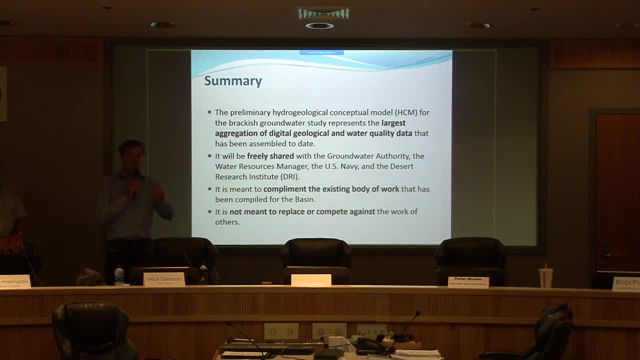 table, because the salinity, the conductivity of the water here is relatively- will give a boundary in our data. Yeah, so if you could maybe quote your questions for just a couple of more slides and don't wrap things up, Yeah, we'll just wrap it up. 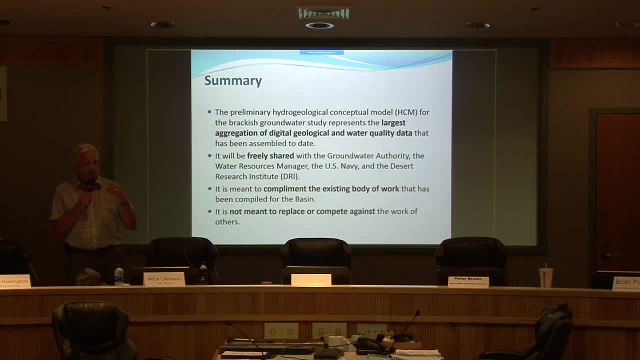 If any of you took public speaking classes, you know you're supposed to tell your audience what you're going to tell them. Then you tell them. then you tell them what you told them. So that's what this slide is here. You've seen this before. 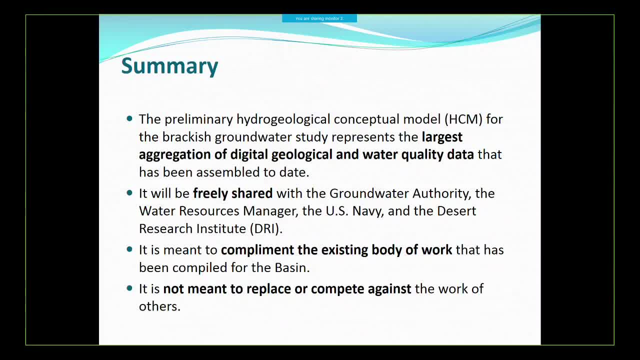 I just want to reiterate that the preliminary hydrological conceptual model for the groundwater study. again, it represents the largest, as you've seen, the largest aggregation of digital geological and water quality data that's been assembled to date. Intent, again, is to freely share it. 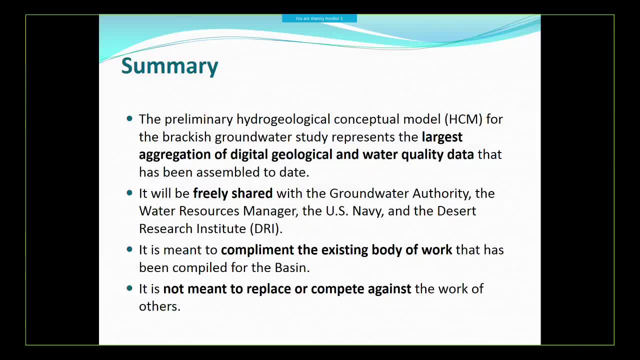 with the groundwater authority, with the water resource manager, with the Navy, with Desert Research Institute. Let them look at it and consider if there's value to add it to the model that the Navy up there has produced. So I'm going to go ahead and wrap up here. 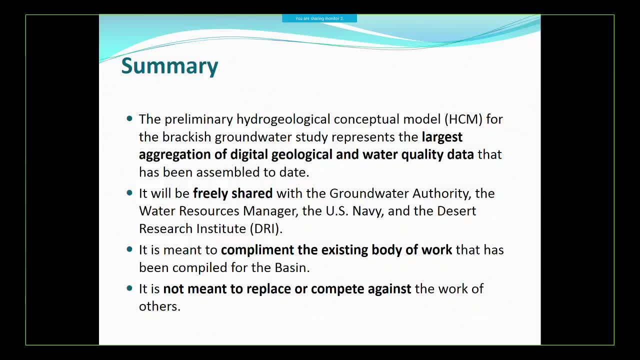 If anyone has any questions, let me know. I think this is probably about time. the slides are up in dates And if you haven't seen it yet, you can go ahead, do so. So we're going to do one more slide. I'm going to switch back to the slide, that's. 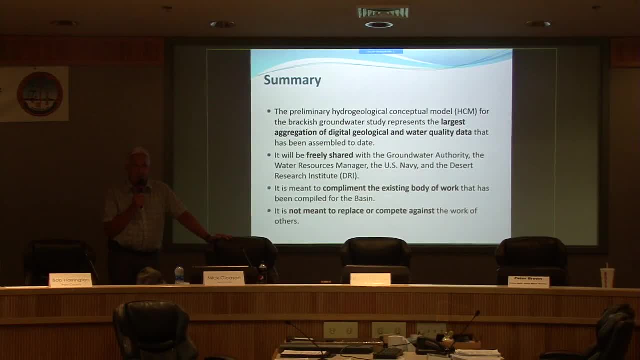 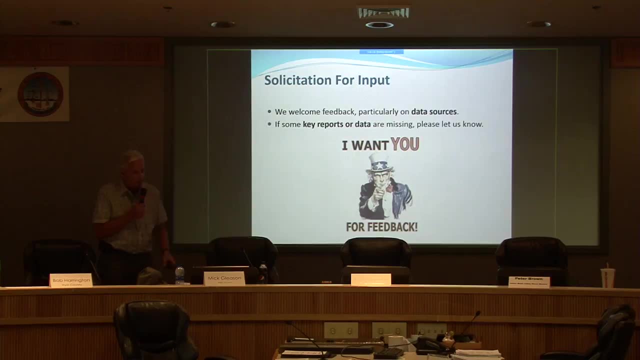 coming up and we're going to go to the next slide, And the first slide is about your data, and we're going to look at data as a whole. What you're doing here is showing your data as some sort of model, And what I've done is I've been understanding. 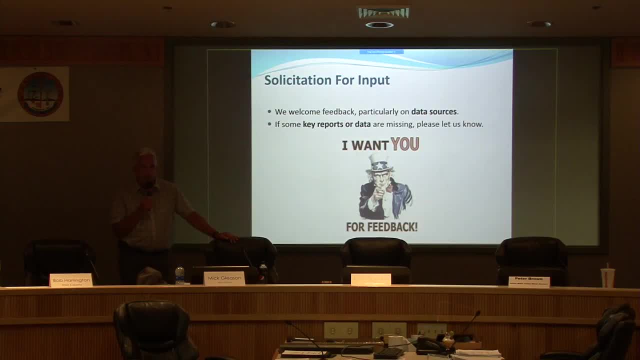 the data and seeing what's happening, particularly on the data sources. if there's other information that you have, we certainly welcome it. if there's some reports, as we handed out that Tim and Max handed out that list of reports- if there's something missing, please let us know. we'll be glad to include it as it says there. we want you. 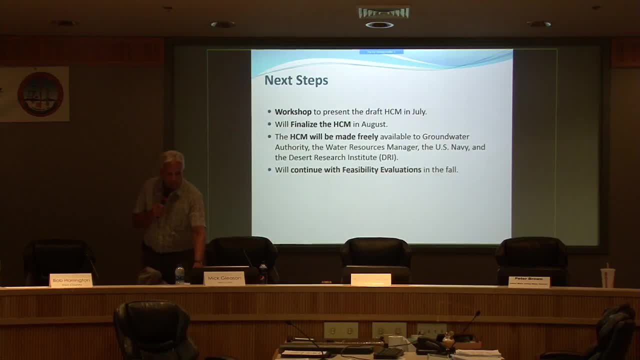 for feedback. so the next steps, as I said, the HCM, the hydrological conceptual model. the intent is to bring it out July, Friday, July 20th, nine o'clock in the morning- hopefully you're a little fresher than you are right now- also after getting input from that, that meeting to finalize the model again. 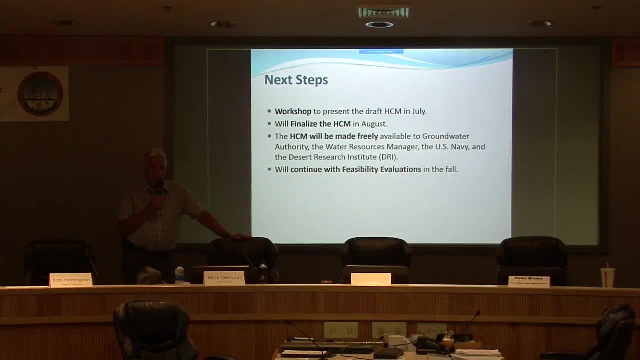 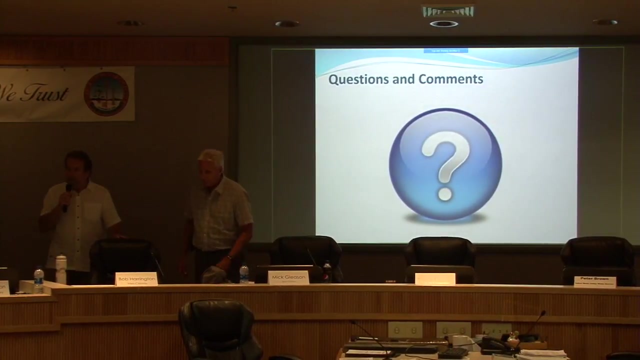 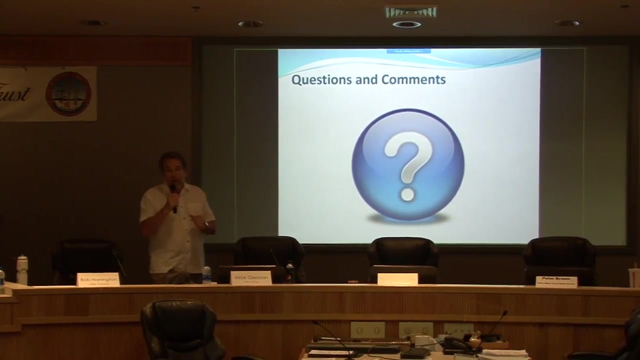 it'll be made available to the groundwater authority, to the water resource manager, to DRI, and we will continue with the feasibility evaluations in the fall. I need to add just a couple of comments in terms of the gap project. so I'm going to make a distinction and Max and I were talking about this earlier, so this gap projects. 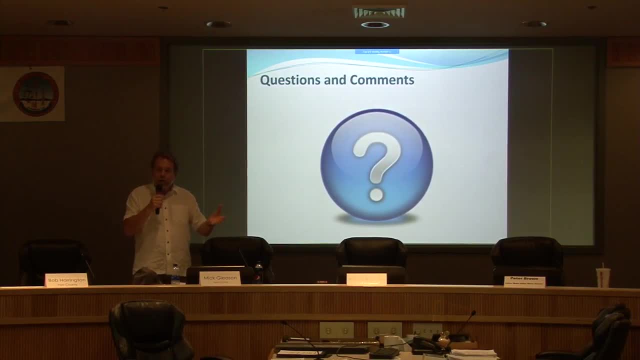 a research project. it has a research component that Stanford and the danish and the state water resources, the Control Board and Department of Water Resources are developing. What this work is, that we're going to present in July, is what we would call the sort of standard approach. 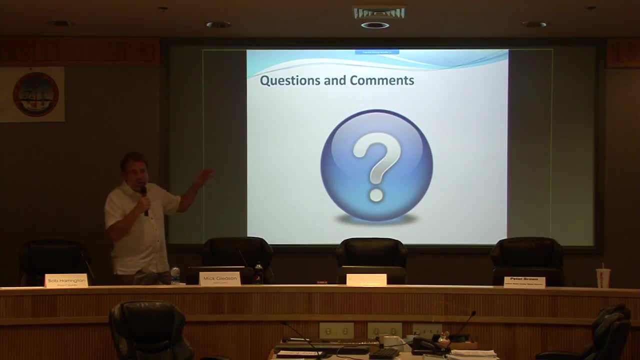 to doing a conceptual model, where we're taking data and putting it in a 3D model and comparing. as I said, we like to. hydrogeologists like to have lots of tools in our toolbox, tools like water quality, water level, lithology, geophysics. 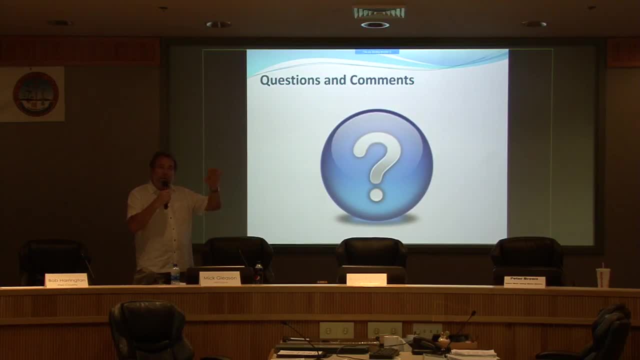 We're taking all that data and basically connecting the dots in a static form in the model, in this 3D computer model. What Stanford is going to do after we complete that is they're going to use multi-point geostatistics to develop. 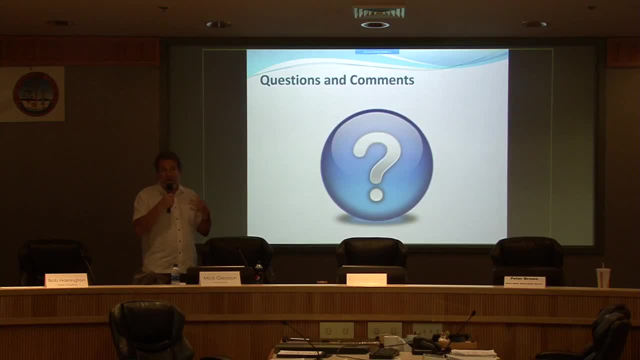 and I'm going to kind of maybe go over some people's heads- but multiple realizations in a modeling context And by that way they will actually fully populate the model beyond what we're doing, and it's an automated way to build a model. 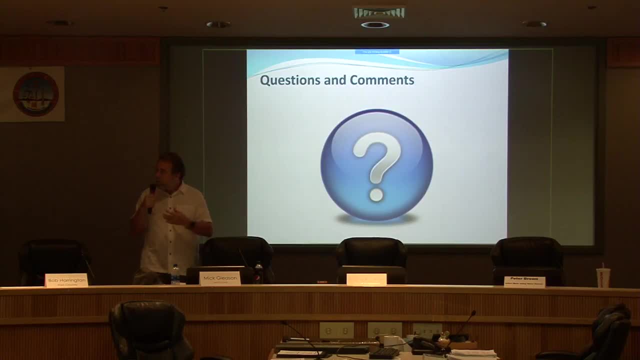 and they'll do uncertainty analysis and pick the model with the lowest level of uncertainty. So there'll be two products coming out of it. One of them will be coming out in a matter of months, The other one will be next year sometime, I think. 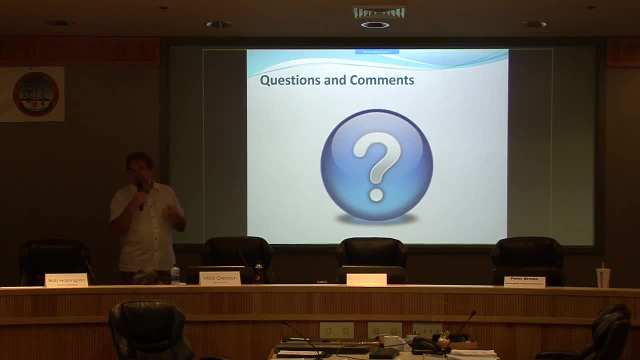 So I just wanted to make sure of that, especially Stetson and DR. I understand that in terms of the model and updating the model, because I think that from my perspective and Max's perspective, we can use the product that's coming out. 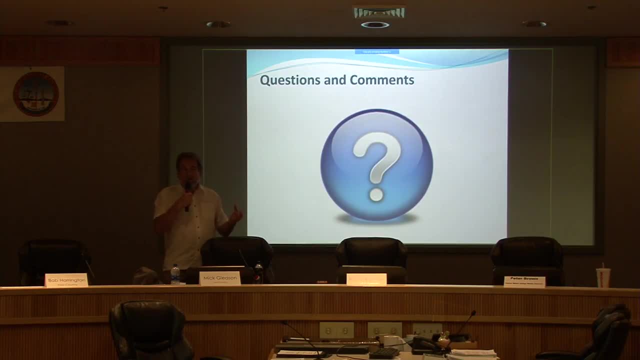 in the next few months to use in terms of a qualitative comparative analysis with the existing flow model to understand the uncertainties and where there's calibration issues. But if there's any talk of additional revisions to the flow, it should probably be after the 3-D multipoint statistical approach is completed. 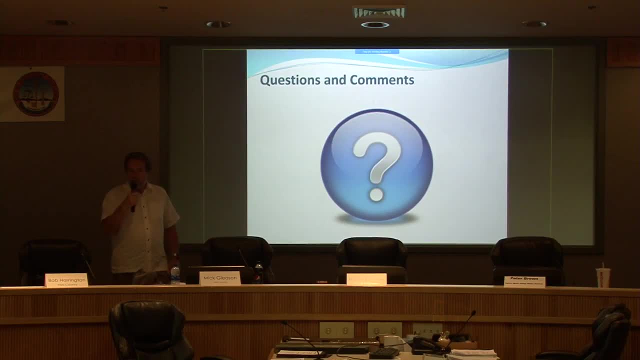 So just wanted to make sure that that message got across. So now any questions? comments. How long did that take me to say Yes down in the front there, Renee? I'm sorry, Could you use the? I hate to ask you to do this, but just since we're recording this, 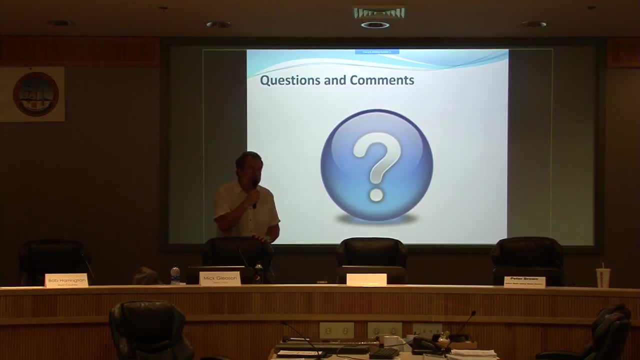 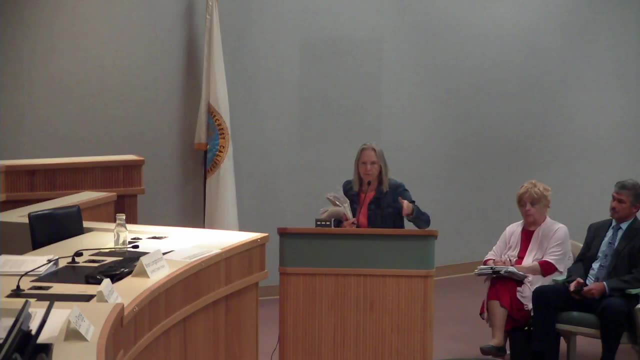 we're going to do a YouTube, We might as well do it the way we record things here. Thanks, Renee. Okay, As far as like the different layers or whatever, does it quantitate? Is this model going to be able to quantitate how much water is actually there? 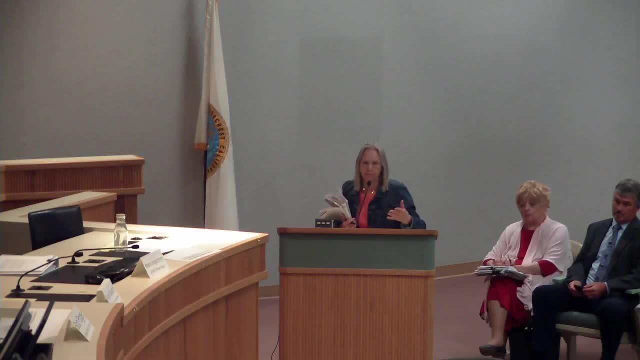 besides the brackish You know, like the depths, And besides brackish, Because you started off you said blue was on one side where it was saline, and then brackish water turns yellowish, green sort of towards less blue. 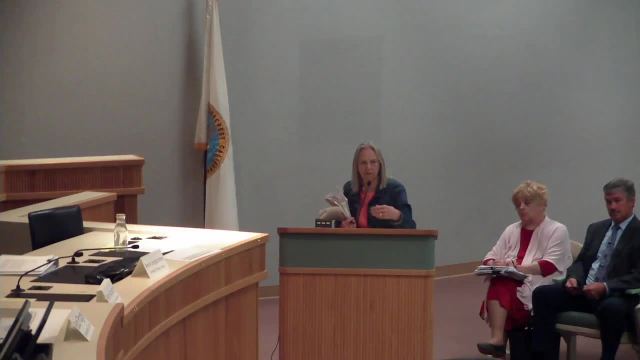 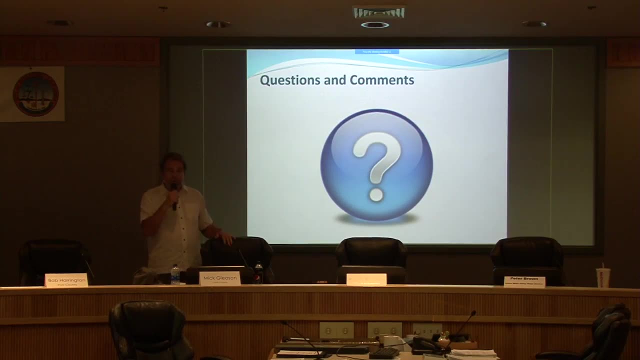 and then yellow-green, becomes sand and gravel Right. So is there going to be a quantitative? Yes, it will be quantitative. There will be uncertainties with it and those uncertainties will be as you remember. you may have seen where we have the most. 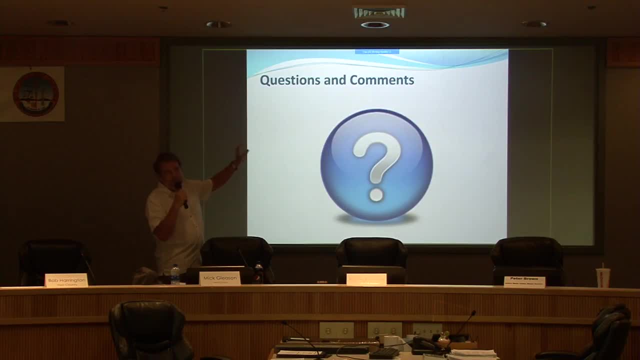 the most data: the wells, the water levels, the water quality. We're going to have a lot less uncertainty of those areas than we are out in the El Paso area, where we have very few wells, But then we'll have the conception, this hydrogeologic conceptual model. 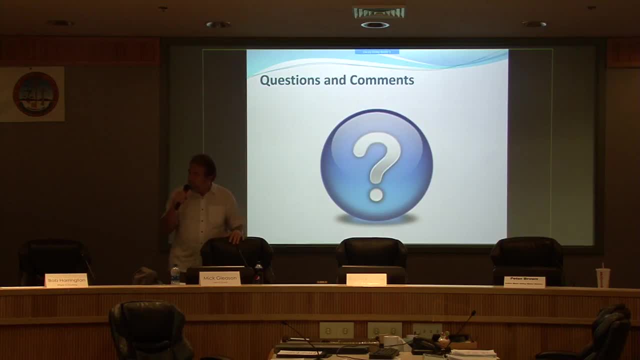 will show how much water. It will have estimates of aquifer properties which will help us estimate how much water is in there and the quality of the water. Okay, so it's not just going to concentrate. It's not just going to concentrate on brackish water. 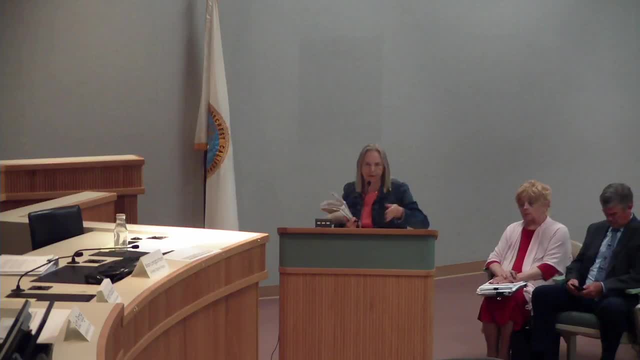 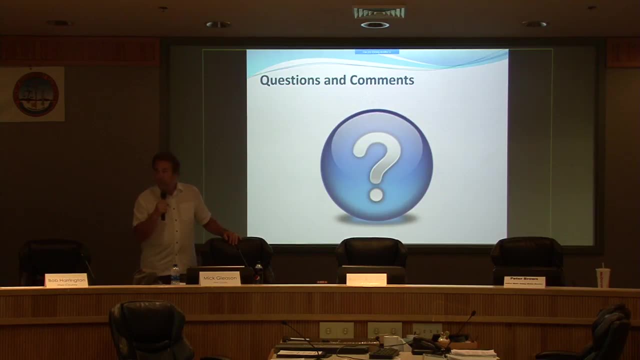 It's going to show all the different available. what is it? layers of water, Right? the different layers that we can identify. yes, Okay, Yeah, yeah, if you, We could actually move over here so we can all three share answering these. 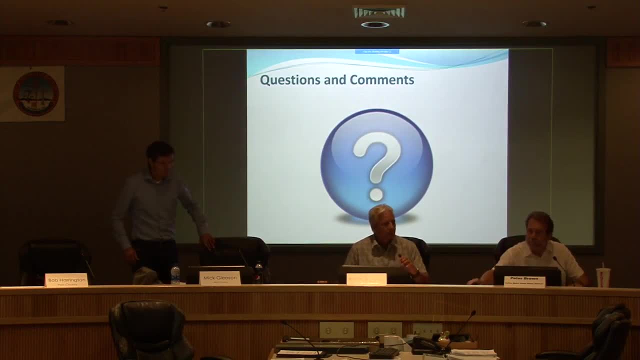 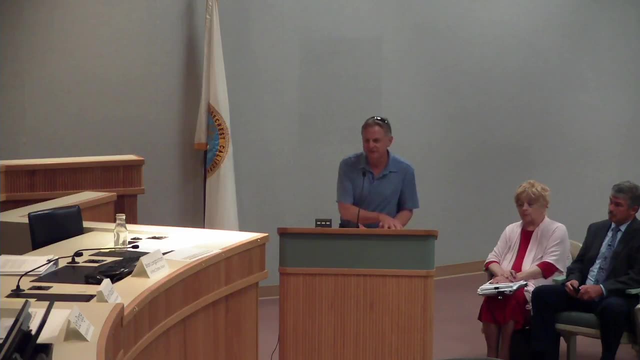 Yes, Stephan Max, your examples show you. extrapolate between data points. Yes, Yes, Yes, Yes, In the valley there are dense data points areas and then there are other areas where there's less data. Do you apply Well? and then there's really sparse areas where there's so little data. 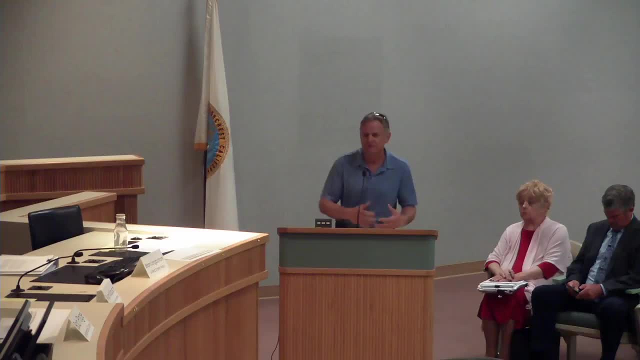 we're calling it a data gap. Do you apply some kind of algorithm to give you a level of quality where you think you have a good extrapolation between data points, or when it's really sparse, it becomes a true data gap. Or is that just a matter of judgment? 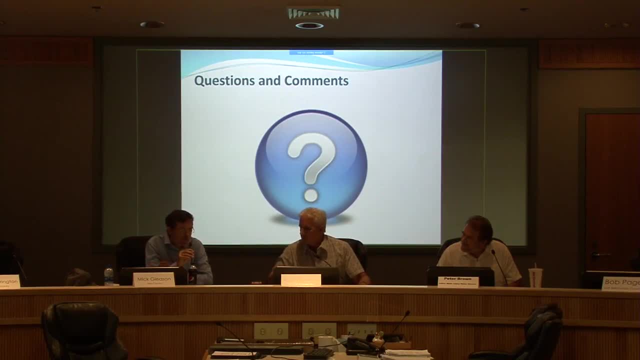 Can you hear me? Yeah, I'll say it's more. Initially, we had a budget on how many lines we could cover, So we had to prioritize where we found that the data would create most value. So that's basically how we came up with a flight plan. 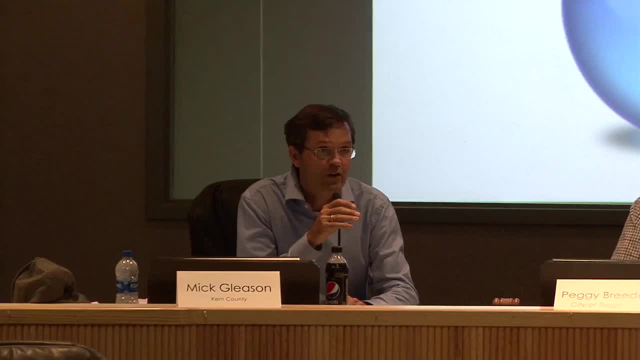 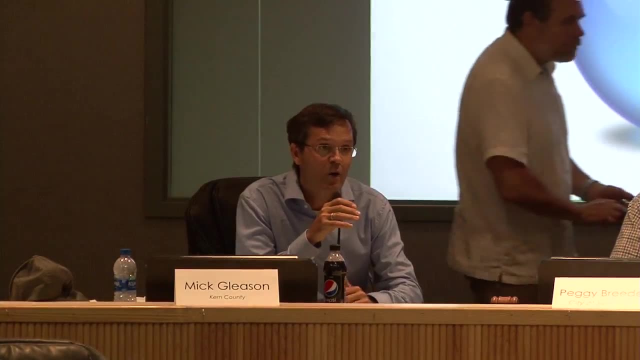 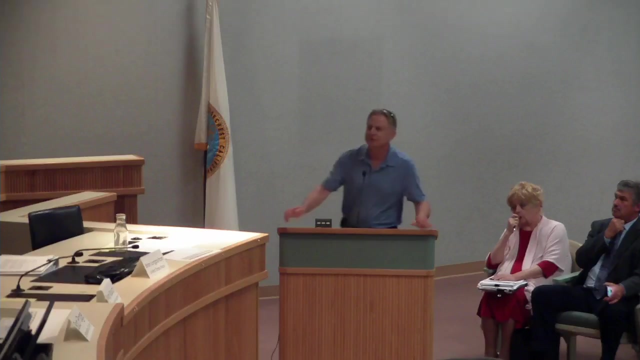 And the flight direction was also controlled by the geology and our general understanding based on existing data. And of course, we will end up with a model here Where our resolution is more sparse- in the southern part of the basin, I guess what I'm getting to. 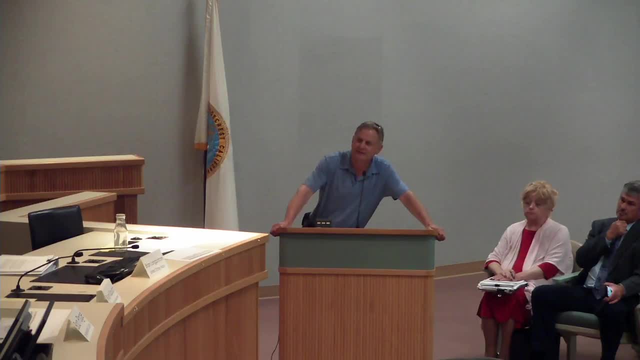 There are probably data gaps that you will identify, that you want to target with additional investigation. If you just go straight off of what you've already extrapolated, you have nice lines between data points and then there's going to be areas where you really feel like 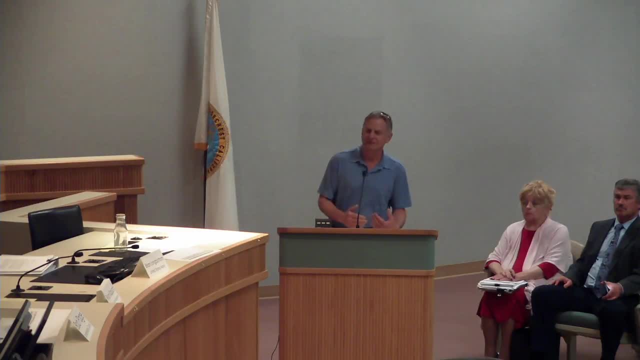 we need some more data there, And I just wonder if there's any kind of statistical algorithm applied saying, yeah, this is really a gap here, Or if you just think that there's something going on there and therefore this is a data gap. 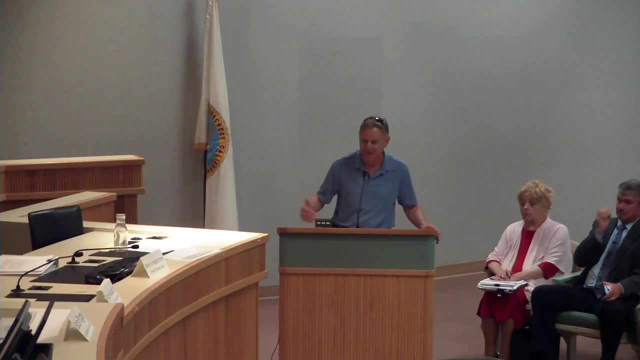 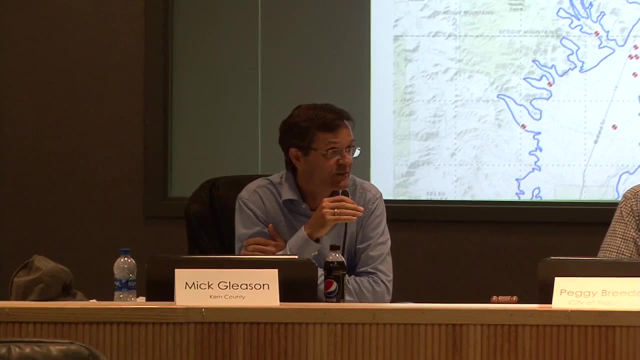 and we ought to get more explanation. See what I mean: More of an automated process or else just professional judgment. Yeah, I'll call it professional judgment. We haven't applied any of the statistics to evaluate exactly where we should position ourselves, And also the results will not be qualified by statistics. 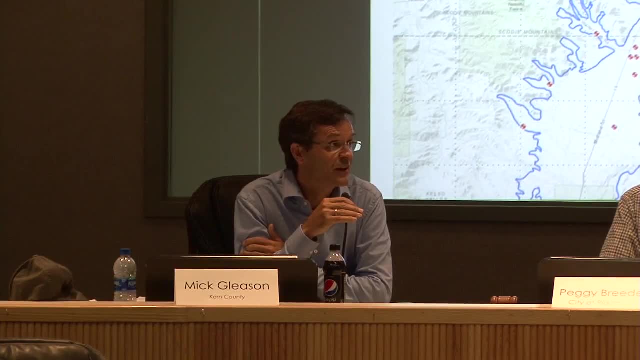 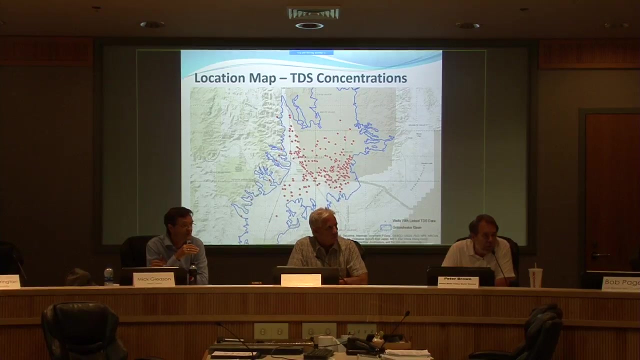 Any analysis in that aspect. Well, for this first phase, But for when the Stanford multi-point geostatistics is done, that will provide quantitative uncertainty associated with this and help us identify the data gaps through that quantitative analysis. So that's the second phase. 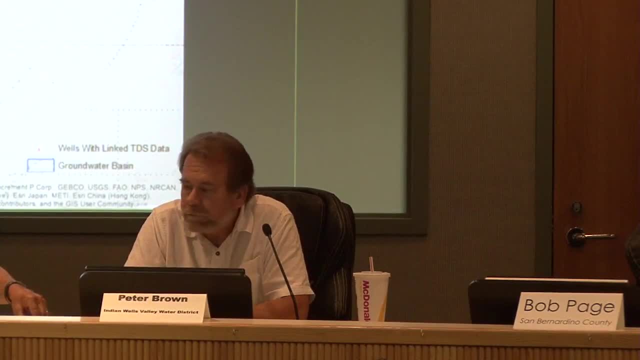 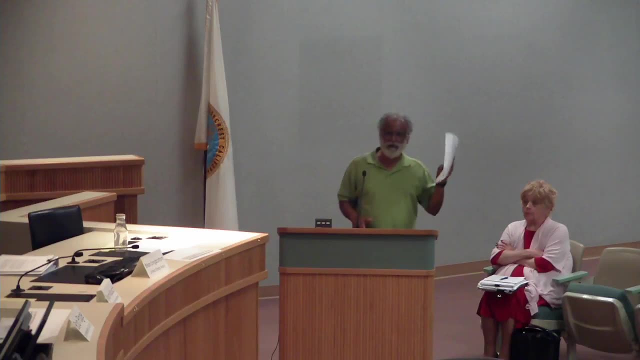 That's next year. Thank you, The answer to this is probably somewhere in one of these papers, But what is your initial estimate? or do you have an initial estimate of the total quantity of brackish water that is extractable, that you think is extractable? 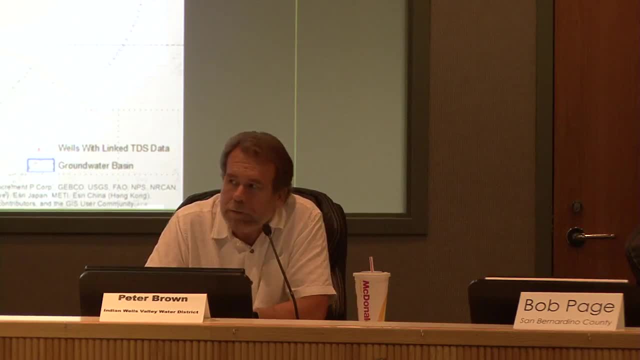 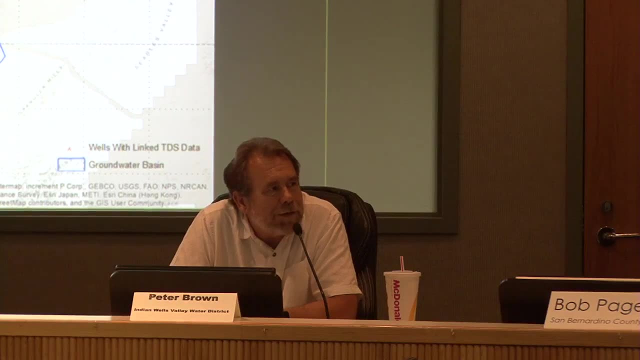 I don't think we have that currently. I'm not sure that. I guess it would be helpful if you could identify yourself. Oh, my name is Jim Vijay. Thank you, Jim. I'm a member of the public. Thank you very much. 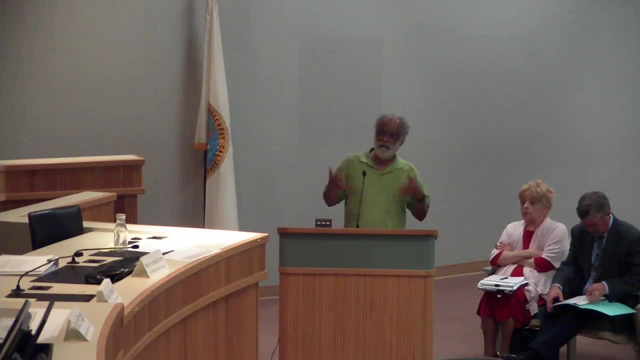 So before you go into this brackish water study, you're not confident that there is going to be enough brackish water to be worth its while. I don't think I said that at all. I said we don't have You asked for a volume estimate. 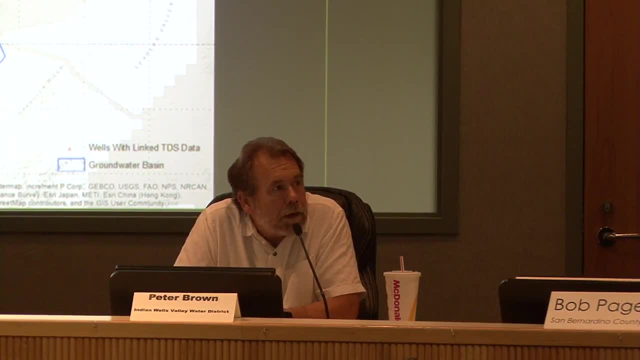 We don't have a volume estimate per se, Not even a back-of-the-envelope type estimate. Well, I'm sure we could come up with a back-of-the-envelope one, but you asked for a volume estimate. An estimate, Yeah, A first-order estimate. 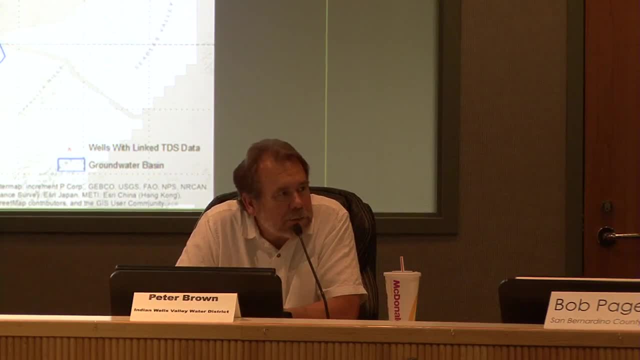 We haven't done that with this hydrogeologic conceptual model And, as you said, yes, the research and the existing data in the basin already has verified that there's a lot of brackish water. I'm not going to put a number on it, though. 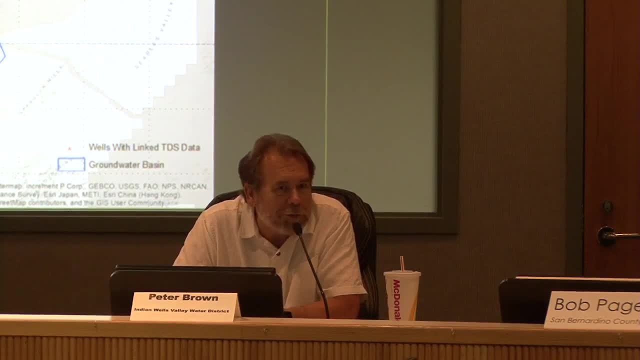 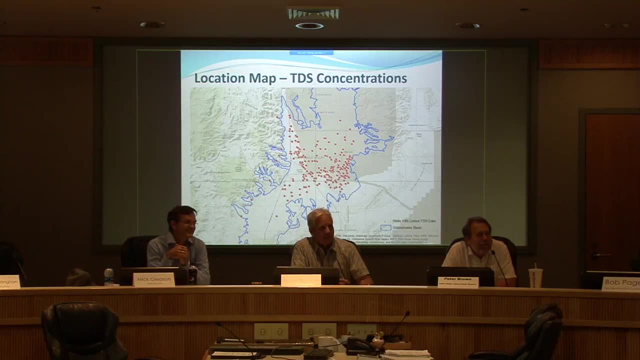 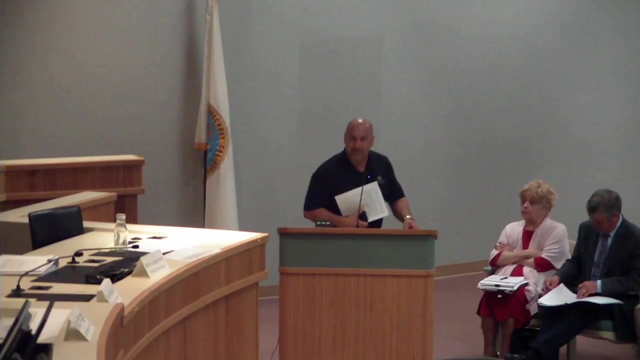 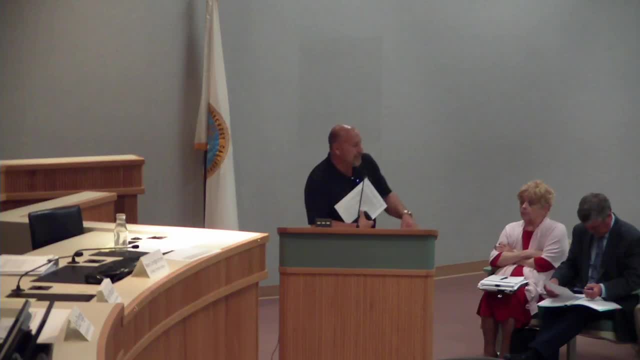 As somebody who contributed some dollars- our company did anyway- to this study. obviously we think that there's significant value here in doing this work and we would not have made an investment had we not thought that there was a rather large brackish resource here. 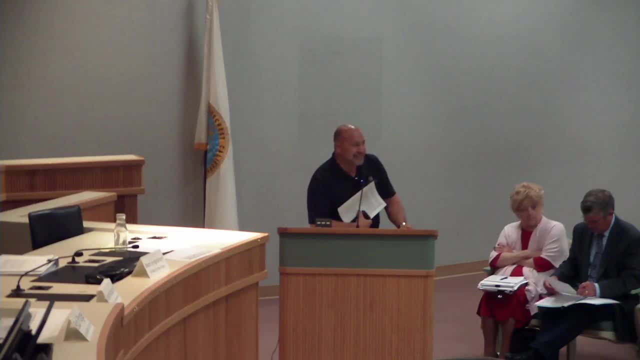 If that helps, and and and, yeah, well, i, i so the the big thing about studies like this and i think, in general, the the public should understand that, uh, the best thing that we can do is continue to collect as much information as possible before we, um, before we just start publicizing things. so, 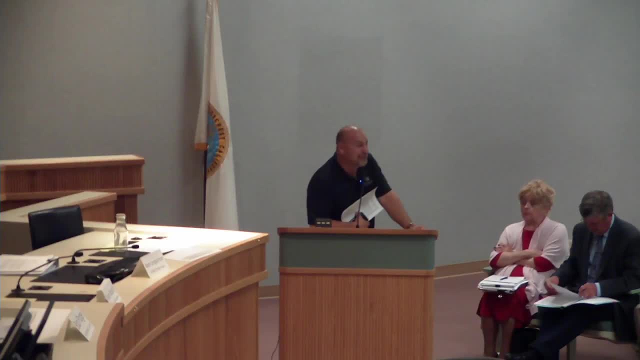 i think by the time we get around to july 21st, we'll have a lot better uh answer for you, um, as a group and, uh, you know this is a nice step forward for us. so, um, you know, we'll see where it goes and we'll see what the uh, what information we glean from it. but, 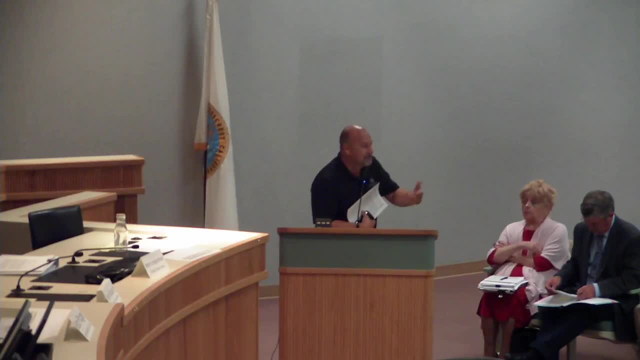 i did have a question, though. um, believe it or not, there's a question in here somewhere. um, so at some point, i would assume that we will take this data- and i already know the answer to this- and we'll overlay it with all of the known data that we've got, uh, associated. 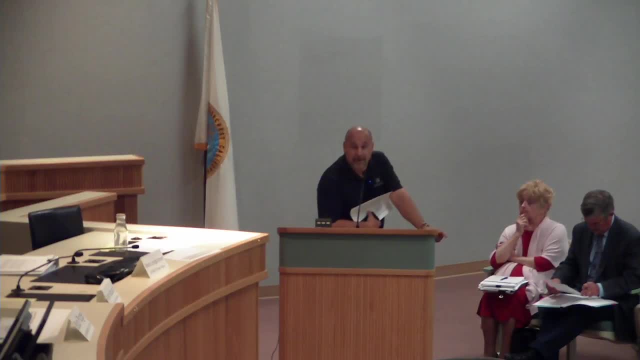 with the models and we'll validate. So that's a yes, we're going to do that. And then, in addition to that, we talk about data gaps, and without going too far into detail as to what next steps might be, but there are real-time opportunities to fill data gaps. 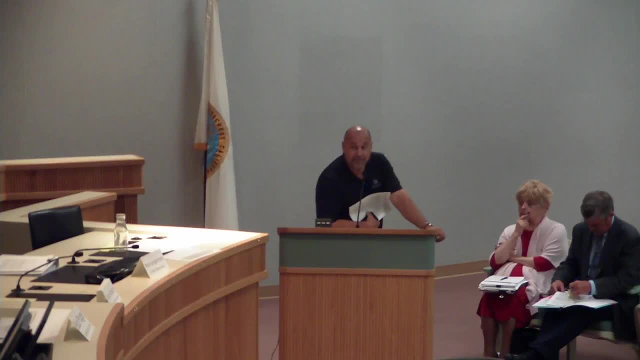 that will require additional investment, I would assume, And you know we're prepared to work with the GA and the TAC in an attempt to develop information that can be helpful in filling those data gaps. So that's – is that okay? 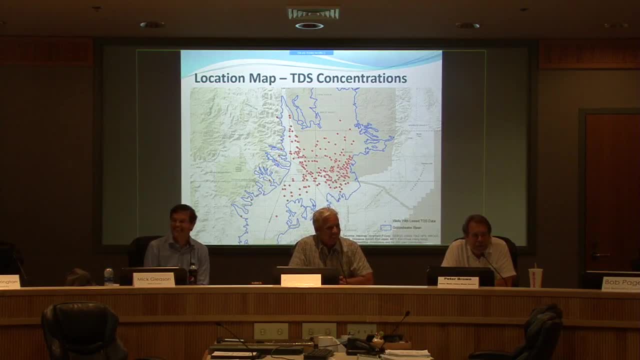 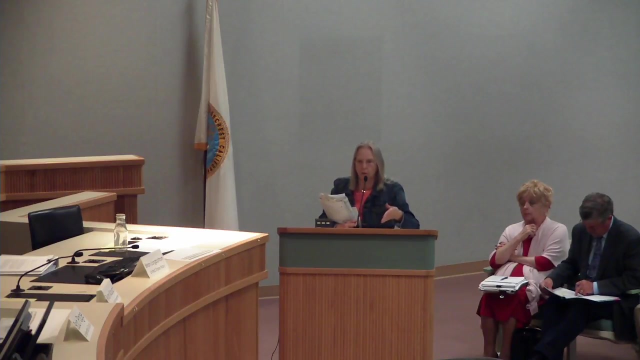 Thank you, Mr Ellis. All right, thank you. I think the answer was yes. Any other comments or questions for our expert panel here? Renee, you want to? I just wanted to kind of get an idea If we can treat brackish water and make it drinkable. 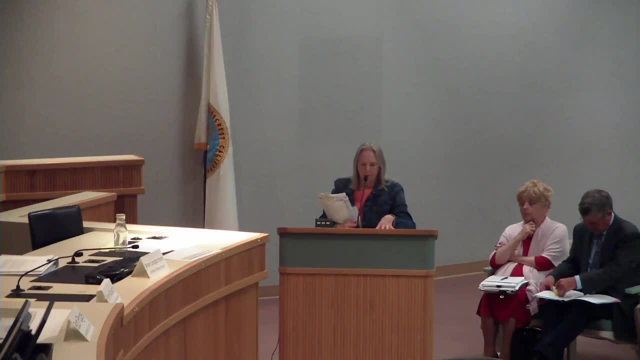 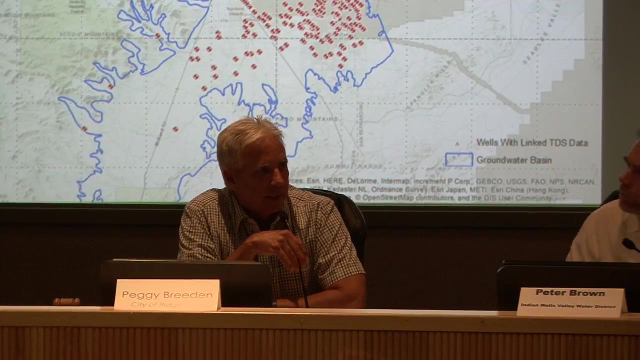 then how does this fit into recharging our basin, et cetera? Like we'll be taking water out, but will we be considered going back in because we're using it? Are we flushing it back into the system? Let me just stop you there, because I think the intent here is not to treat it. 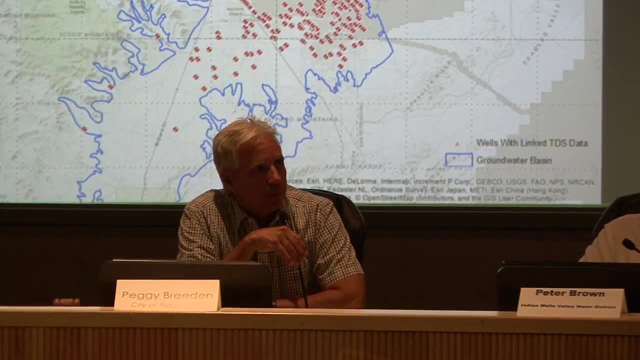 so it's used as drinking water, but to identify where it is, treat it to a level where it can be used to maybe offset current uses of potable water. There are several examples of that. We have kind of a unique situation here in this basin. 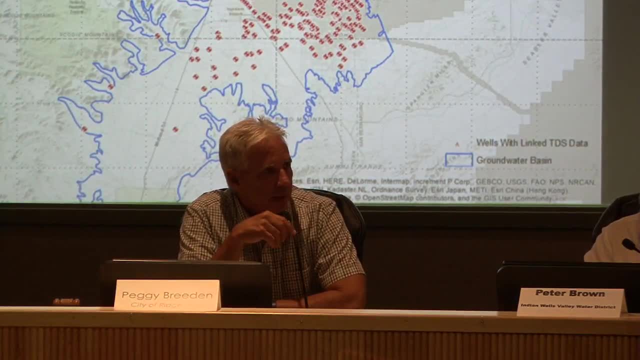 which I think Tim and myself and Wade Major went to Sacramento and when we were submitting the application for the grant and met with DWR and one thing that they recognized was that it's very rare for an inland desalination plant to have customers, if you will, for the product of the desal plant. 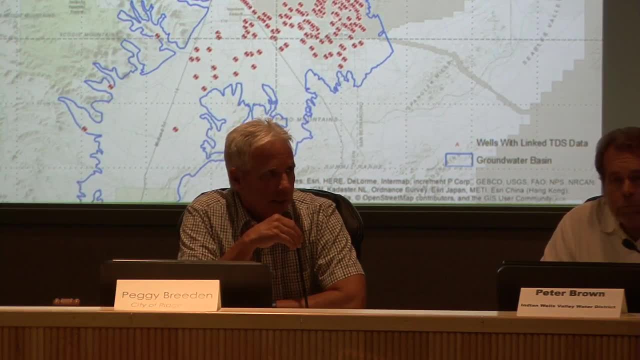 We have a couple of potential customers in Searles Valley: Minerals and Coastal Geothermal, possibly even agriculture Pistachios. my understanding is they don't require potable water, So it's to find where the brackish water is, to quantify it, which we don't know quite yet. 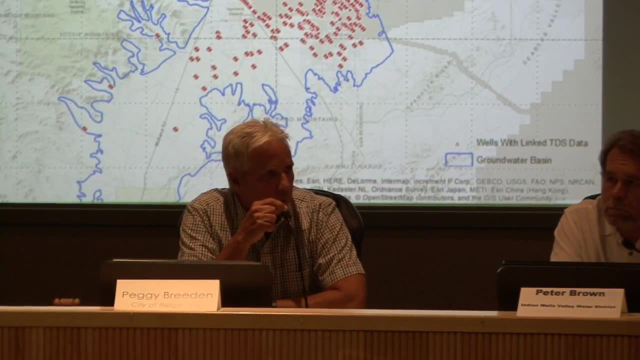 and then find an end user for it that maybe is using potable water. now that could use the brackish water in place of that. So again, just the intent isn't to treat it to drinking water standards I mentioned earlier when we were talking about the district. 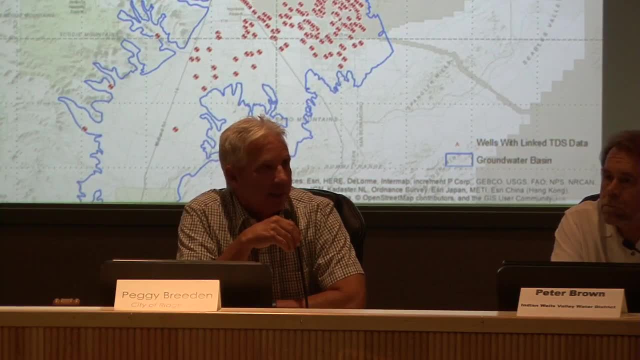 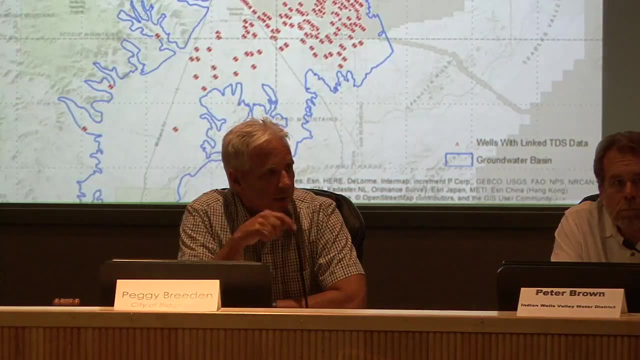 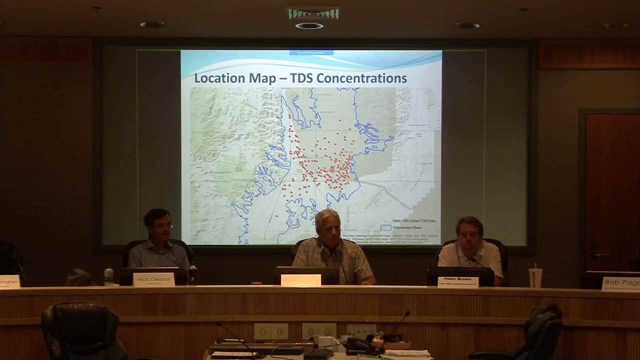 the water district pursuing brackish water that the intent then was to look at using it as a source of water for our customers, but that scope has changed now In this current feasibility study. Okay, Thank you. Anybody else? Last chance Going once. 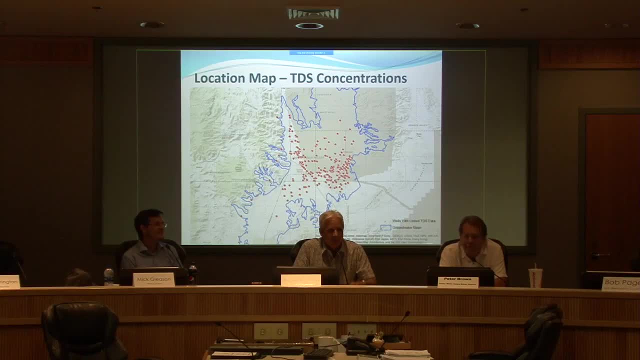 It's been a long day and I appreciate those of you that stuck through it to the end here, but hopefully you found this of interest and if you did again, July 20th, Friday, 9 o'clock, is the intent to have the follow-up to this meeting.